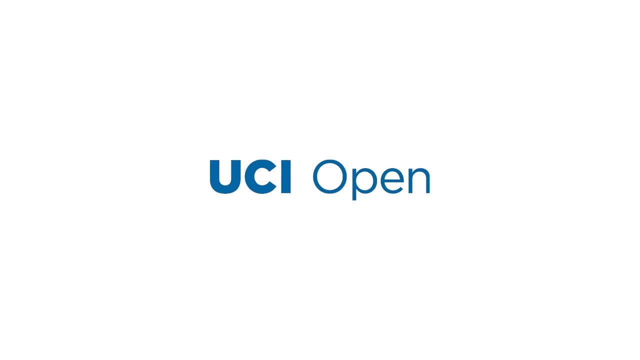 We're going to talk about pericyclic reactions today. I'll introduce the idea of what pericyclic reactions are today And then we'll discuss electrocyclic reactions- electrocyclic ring opening and closing reactions, And we'll talk about thermal and photochemical processes. 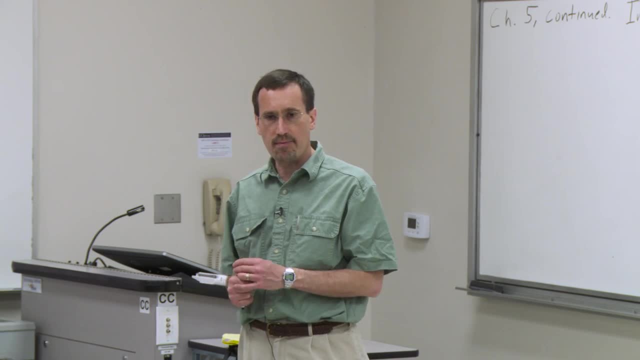 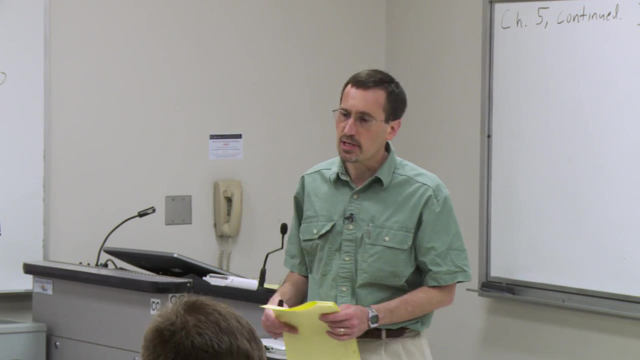 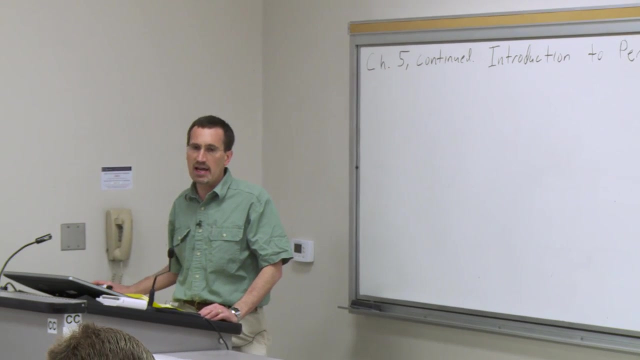 And then on Monday we'll pick up talking about, we'll finish off chapter 5, talking about cycloadditions and sigmatropic rearrangements. So let's begin. Okay, so we were developing concepts of orbitals last time and the idea that conjugated pi systems have molecular 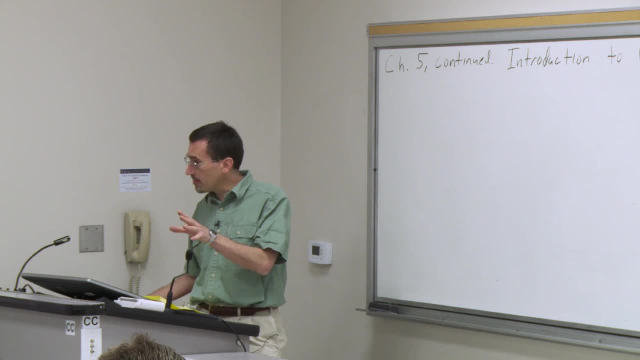 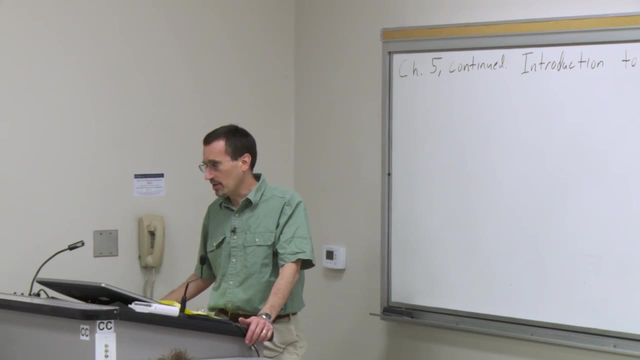 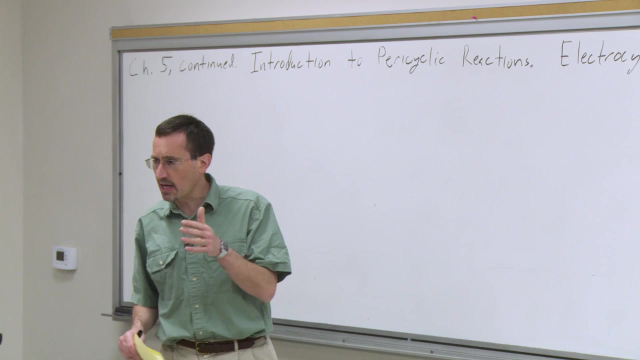 orbitals And we looked at how the atomic orbitals, specifically the 2pz orbitals, are combined in making the molecular orbitals of pi systems. I also said there's something very important about the highest occupied molecular orbital, the HOMO, and the lowest. 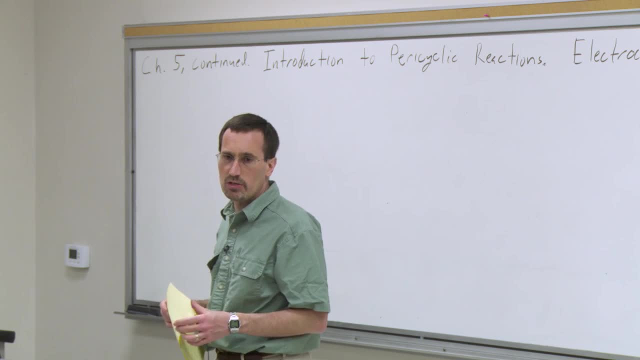 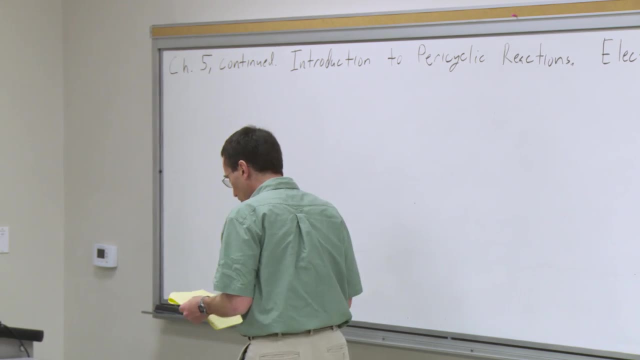 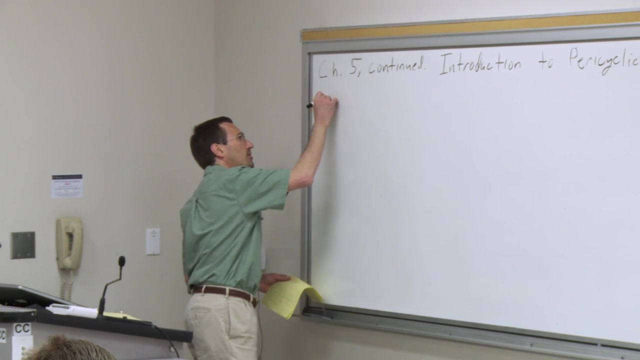 unoccupied molecular orbital, the LUMO. These constitute the what are called frontier molecular orbitals, the molecular orbitals that are involved in most reactions. Alright, we're going to use those concepts today, Okay, as we discuss pericyclic reactions, And so what I would like to do for starters, 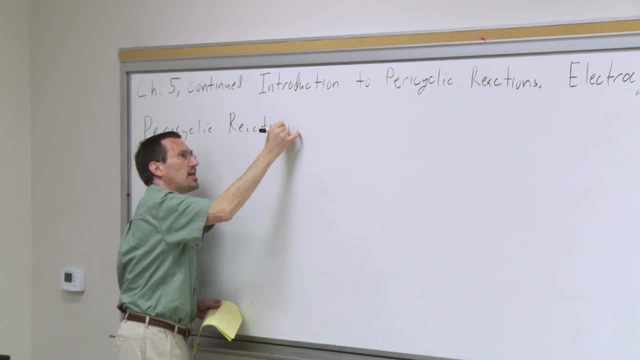 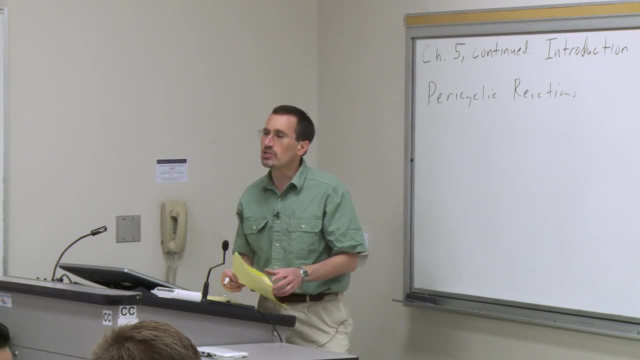 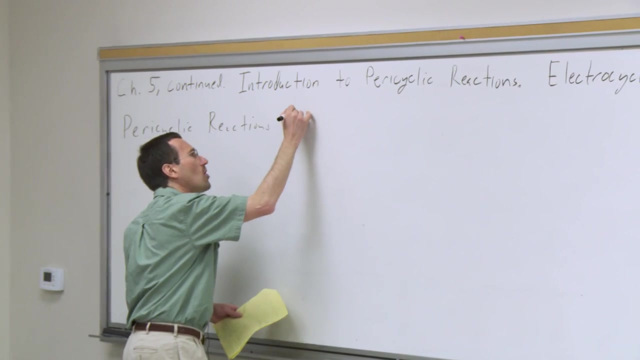 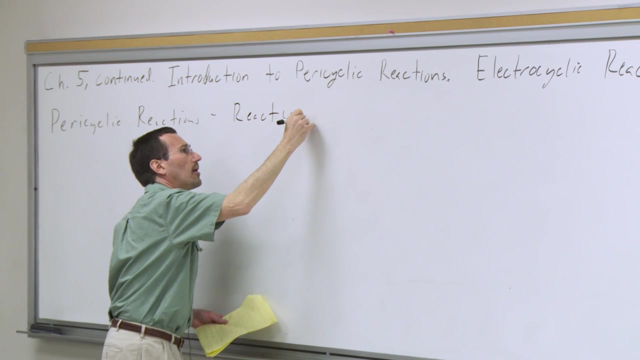 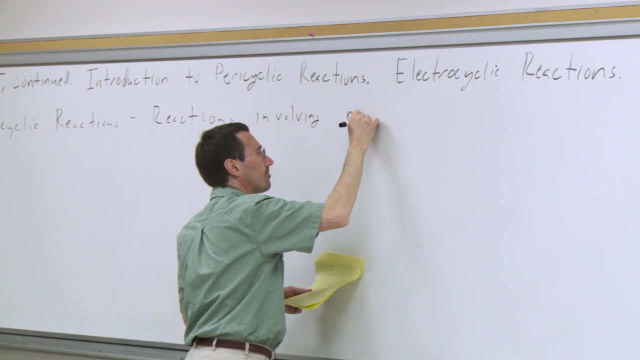 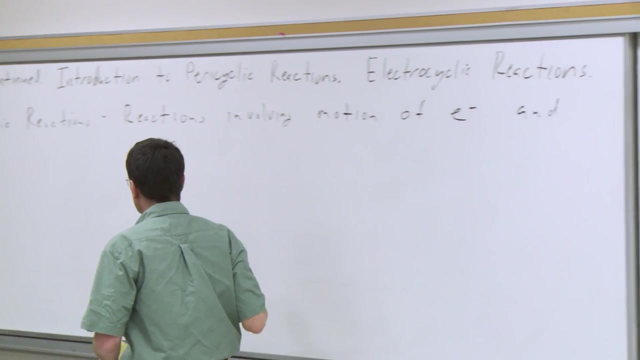 is to introduce pericyclic reactions and just talk about the three categories of pericyclic reactions. So pericyclic reactions are reactions involving the motion of electrons and the reorganization of bonds without the formation of intermediates. Here we have the linear response. that is the same reaction as the linear response of the. 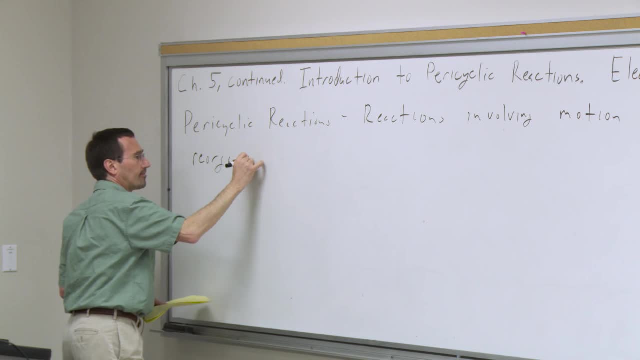 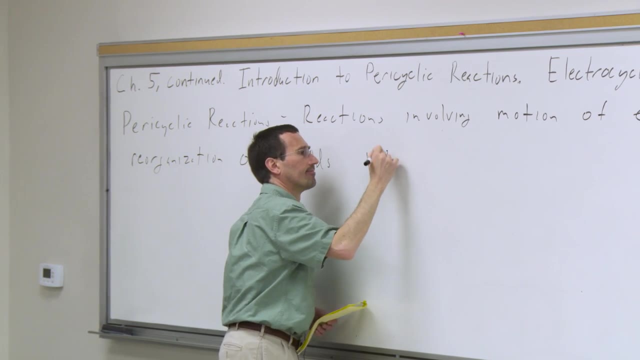 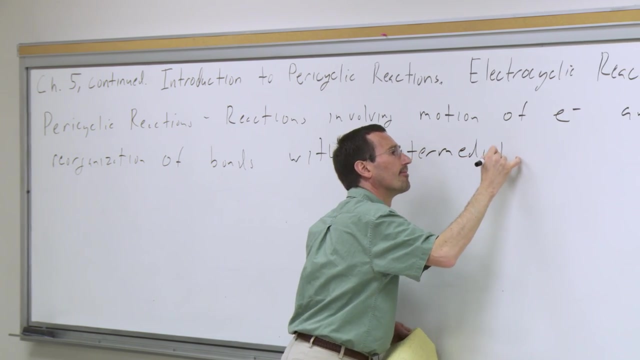 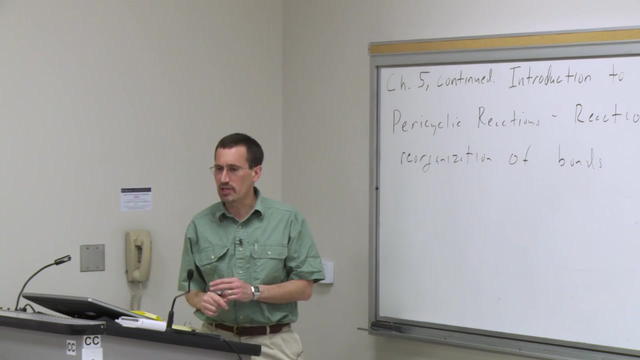 balancing of bonds without the formation of intermediates. So first we're going to compare these two. Okay Alright, here we go. Okay Okay, Okay Okay. Classic example of this would be say, a Diels-Alder reaction, the example that you learned in sophomore chemistry. 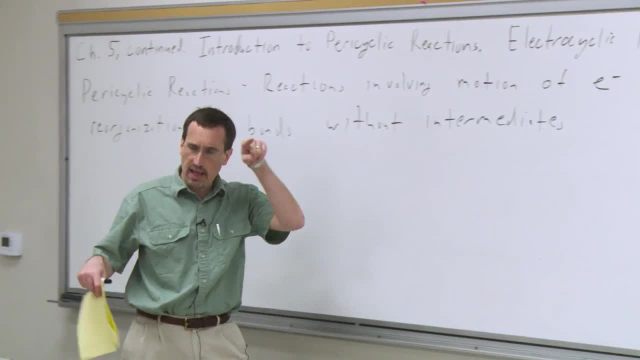 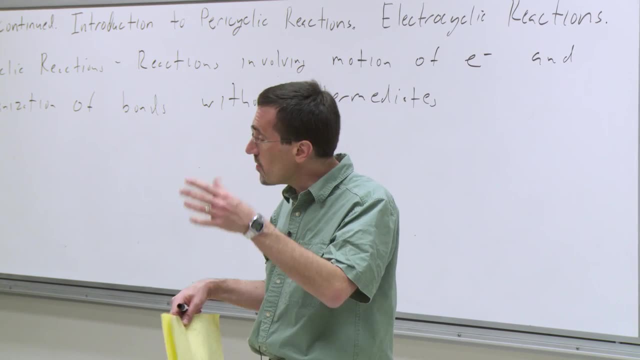 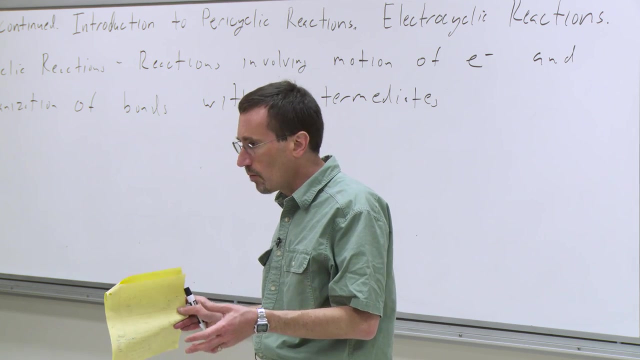 and probably remember still, where six electrons move around at one time and you get new bonds and there's no point along there where you have a carbocation or an anion or a radical- All the electrons move around at once. Now there may be cascades of pericyclic reactions. 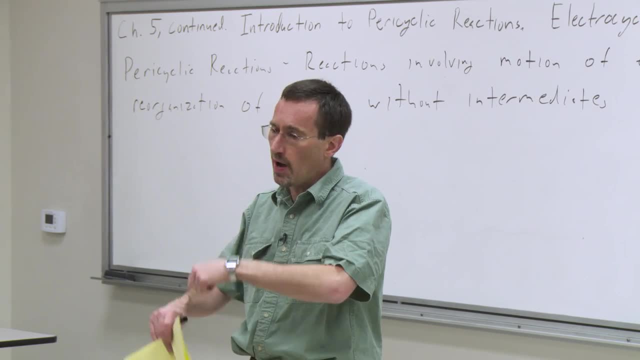 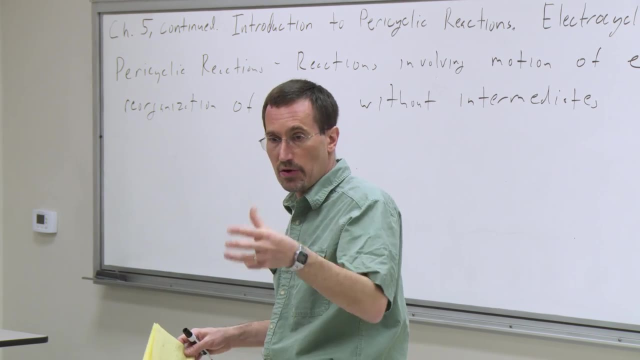 You will see them on the homework problems where, for example, you have one electrocyclic ring opening and then another, say a cycloaddition, or another electrocyclic ring closing And of course there you have an intermediate in this cascade. 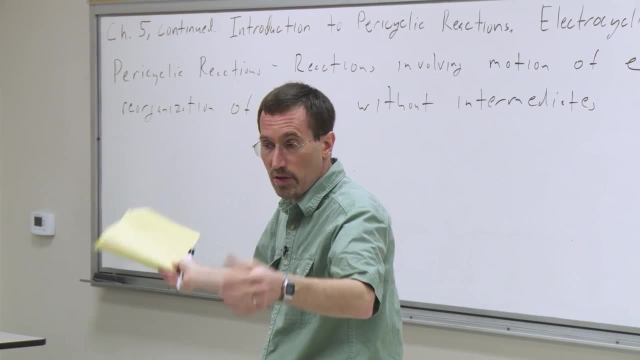 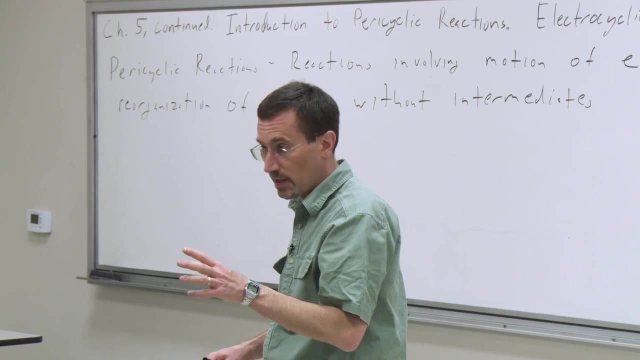 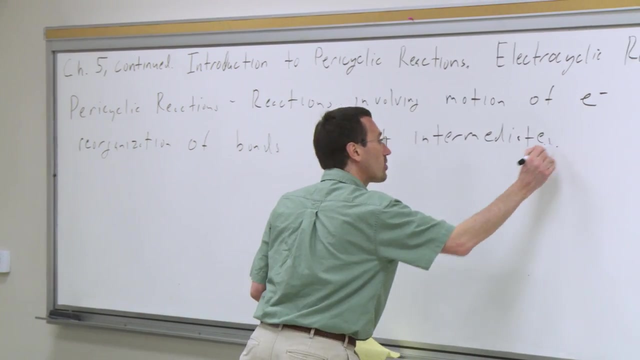 It's the product that formed by opening or the product that formed, you know, by some other process. But the point is, in getting from one species to another species, we have no intermediates, no reactive intermediates here. All right, there are three main classes. 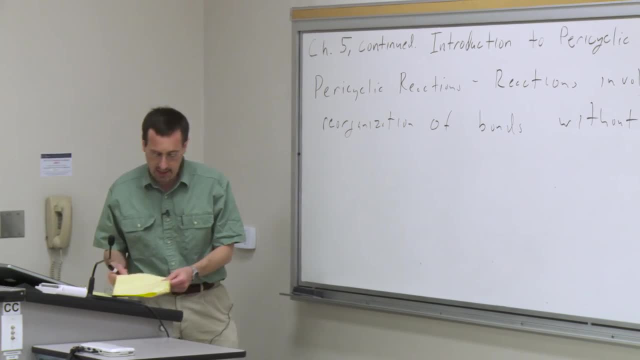 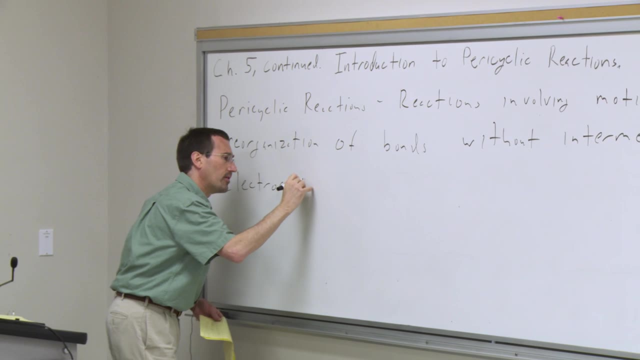 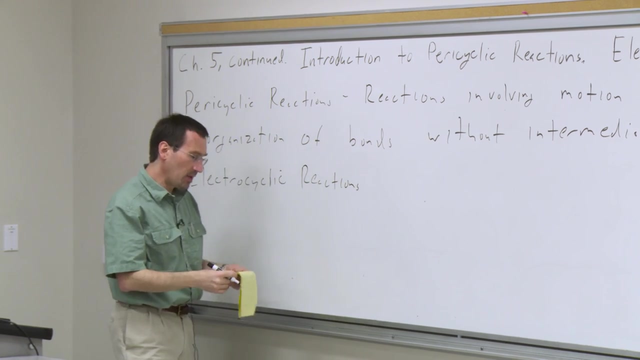 of electrocyclic, of pericyclic reactions, And I'll write out with examples. So, electrocyclic reactions, what we'll be talking about is the reaction of an anion, And I'm going to draw out today and so, an example of this. 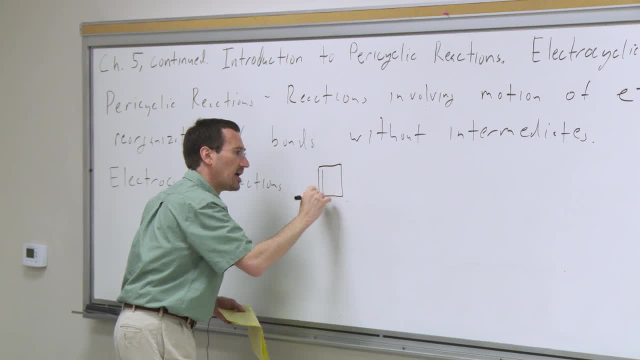 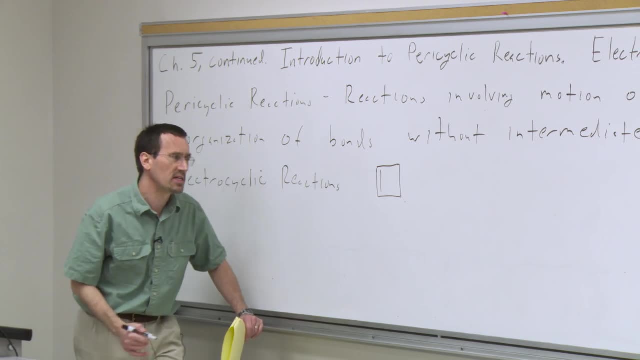 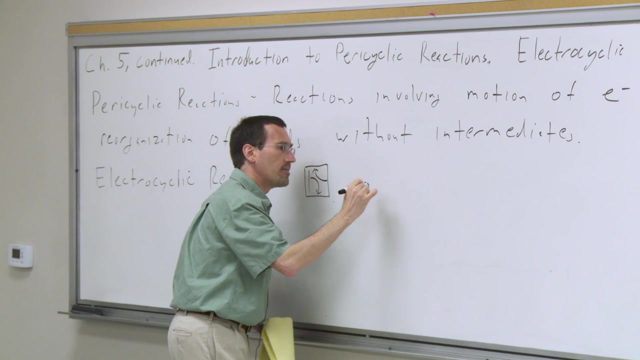 one that we'll be seeing later on in the lecture is, say, taking a cyclobutene and all the examples I'm about to draw out. now I've just drawn the minimal systems moving electrons in a ring like so, And by now you should understand the meaning. 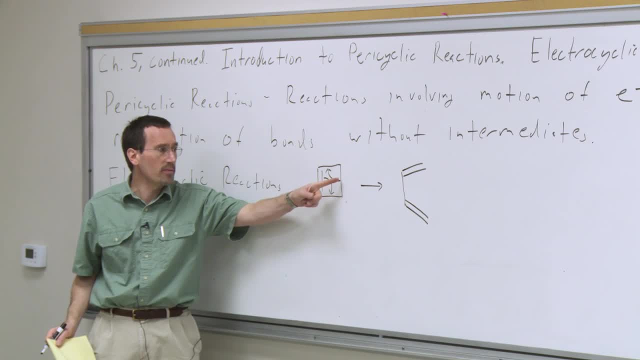 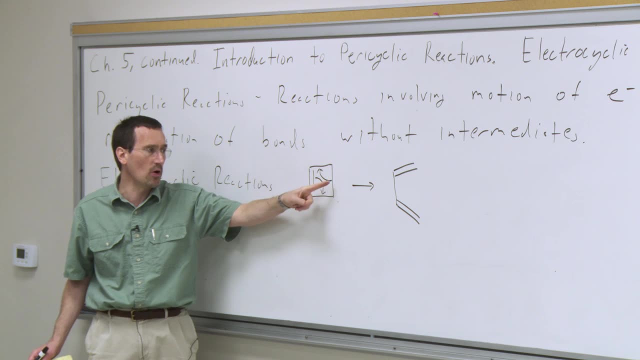 of that, The meaning of the curved arrow. in other words, the curved arrow means we're moving electrons from this bond here on the right over to this top bond here and going from a single bond to no bond and then, on top, going from a single bond to a double bond. 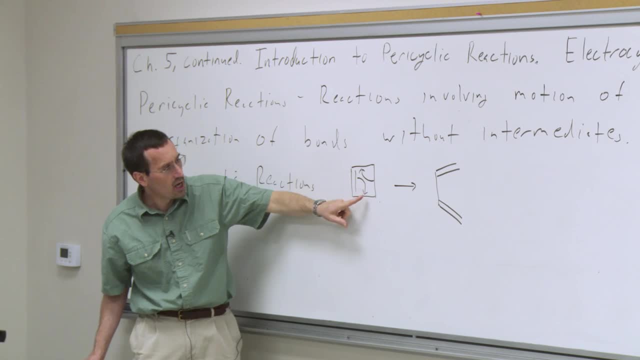 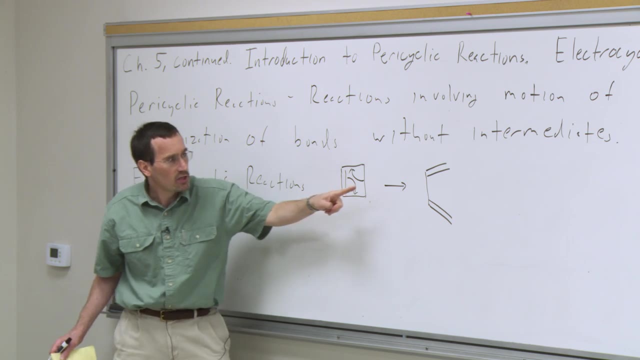 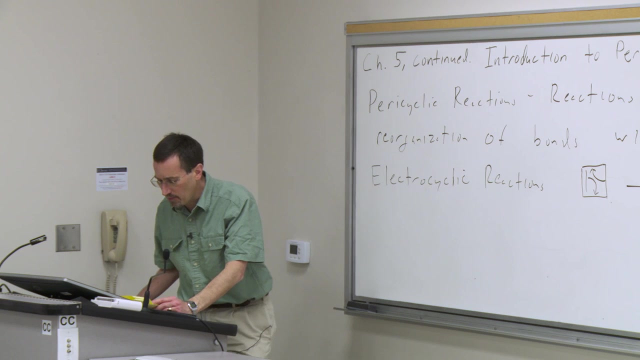 We're moving the electrons here from this pi bond on the side to this bond on the bottom, and so we're going from a double bond to a single bond And then on the bottom we're going to a double bond. So if I had to describe this process in general, 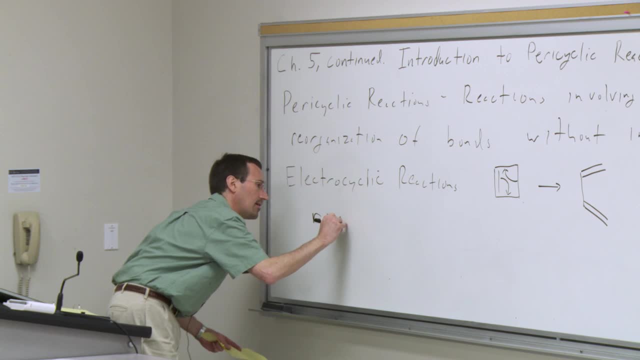 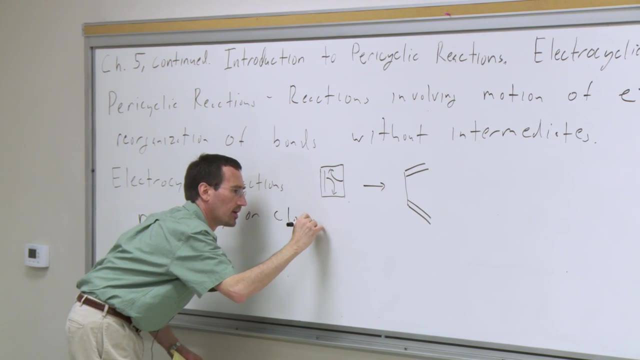 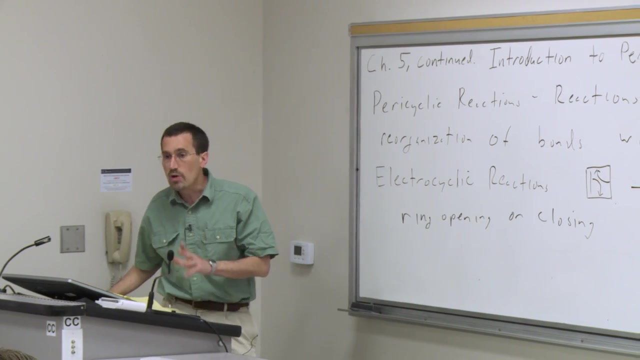 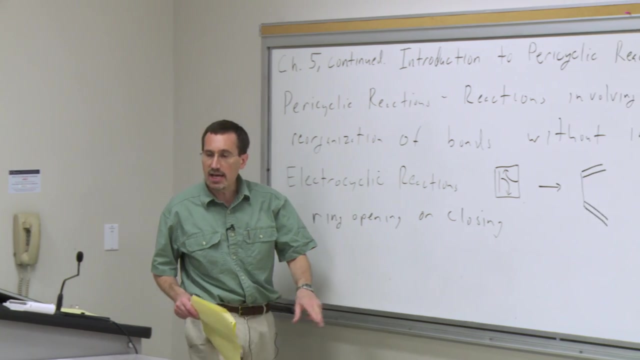 I'd say ring opening or closing. we'll start with an example of closing. in fact, as we get into this topic- ring opening or closing- and the other hallmark of an electron, And so the reaction we get is that we can see that the nucleotide reaction is a very similar reaction. 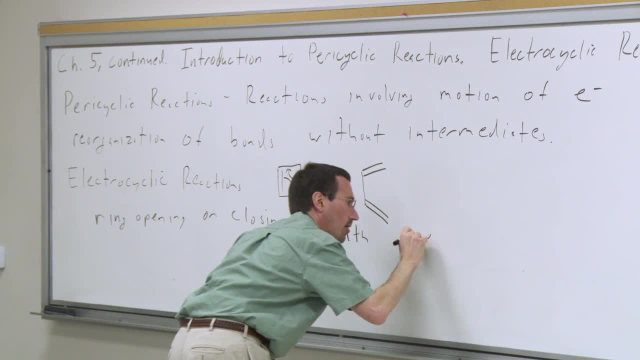 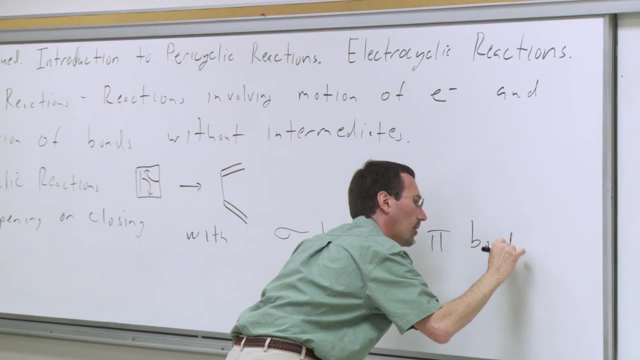 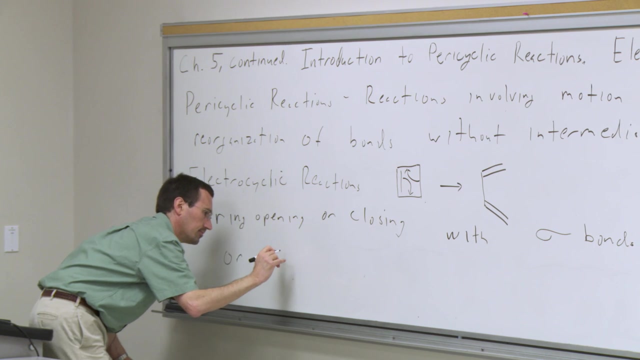 to the electron cyclic reaction. So if we have a ring opening, we're going to a double bond on the side and then on top of that we have a ring opening or closing. on top of that we have a ring opening and then on top of that we have a ring opening. 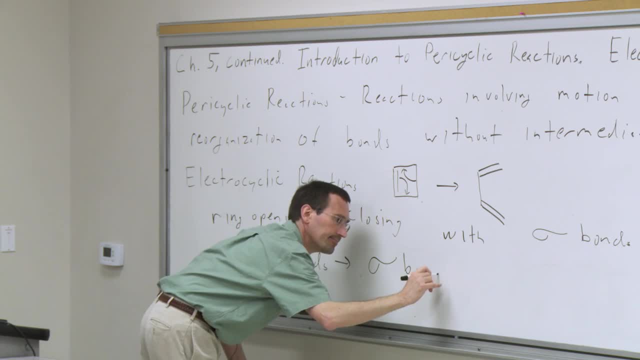 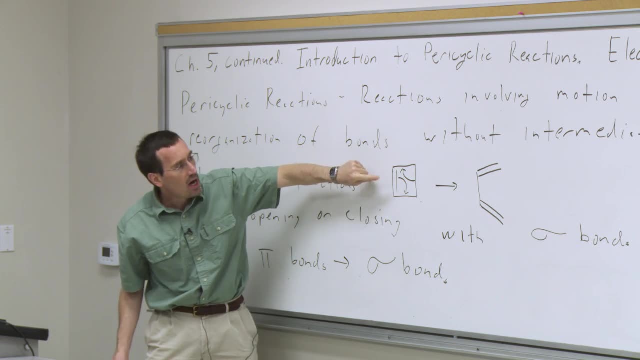 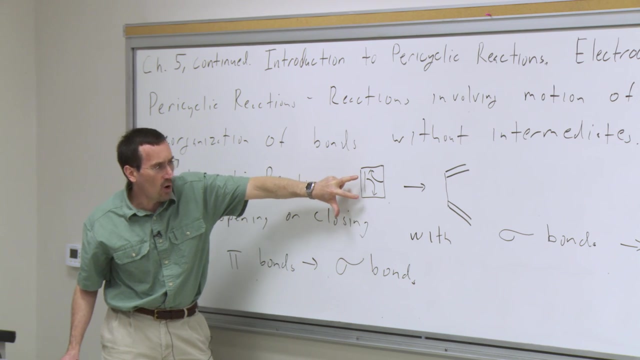 So we're going to have a ring opening. In other words, in this little example over here, we have one pi bond on the left and two pi bonds on the right. We had four sigma bonds on the left but only three on the right. 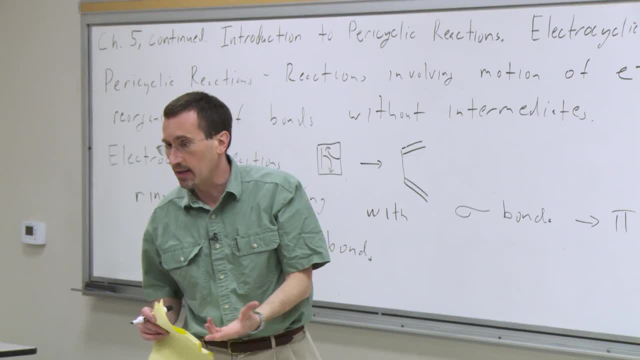 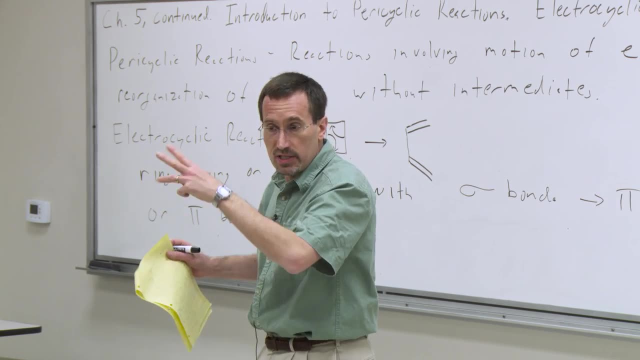 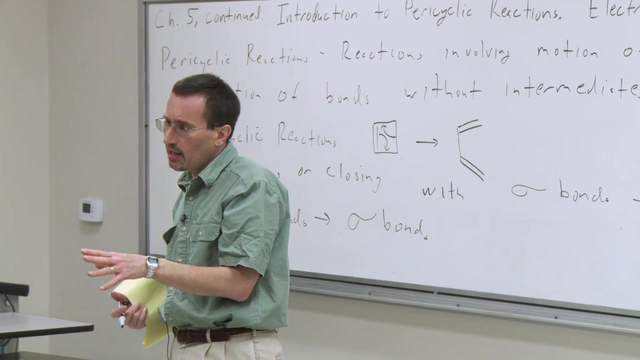 In other words, we still have the same number of electrons in the molecule, We still have the same number of bonds, but we have transformed sigma bonds into pi bonds And indeed- although we're not going to discuss this in depth- in the class the reaction occurs by a smooth 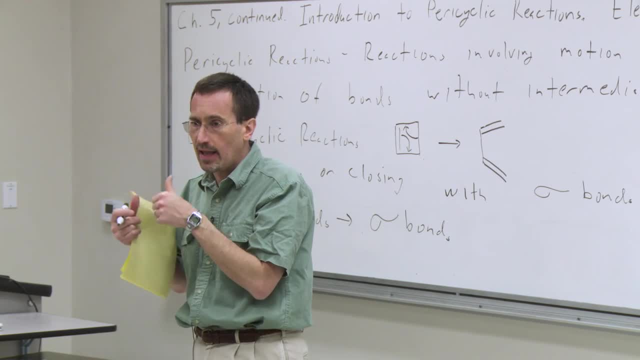 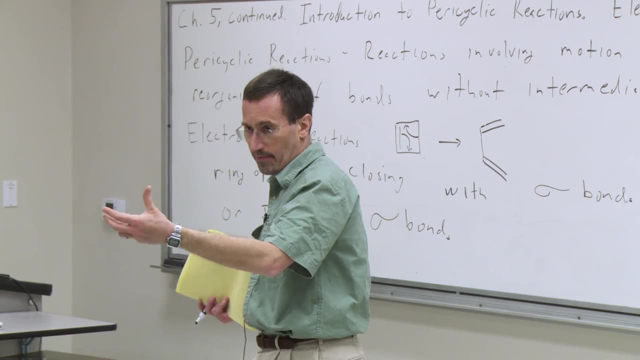 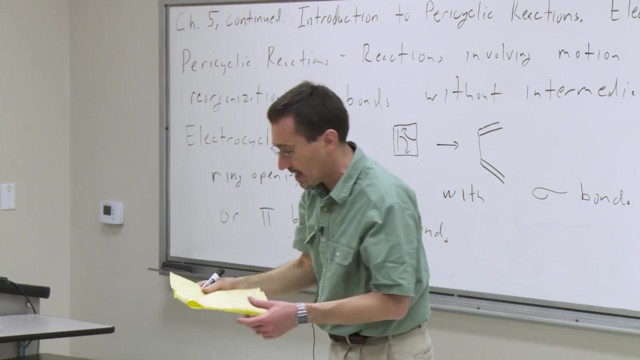 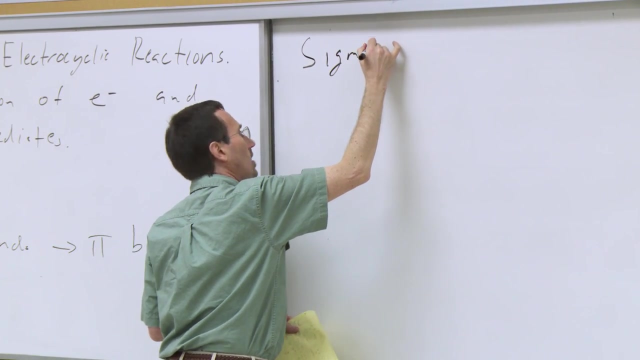 and continuous transformation of molecular orbitals. In other words, a pi-type molecular orbital becomes a sigma-type molecular orbital. as the orbital is transformed, The orbitals rearrange as the reaction goes over the transition state and on to the products. Okay, the next archetypal paracyclic reaction. we'll talk. 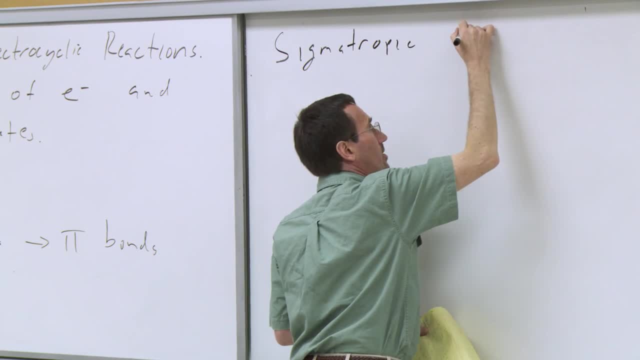 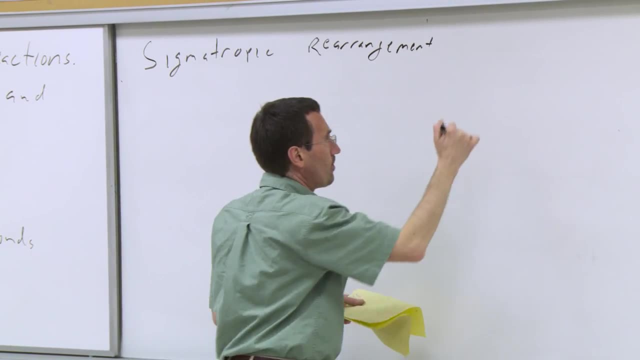 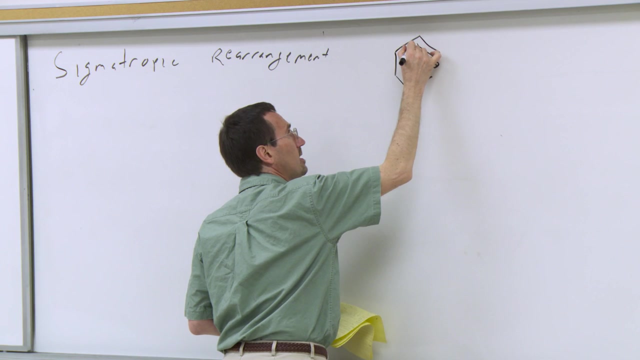 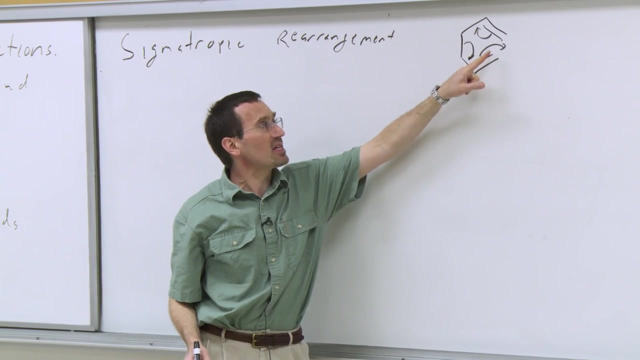 about is a sigmatropic rearrangement, And I'll just draw out one example. It's a 3,3-sigmatropic rearrangement called a Cope rearrangement. I've pushed, so I've started with a diene. I've pushed six electrons around a ring. 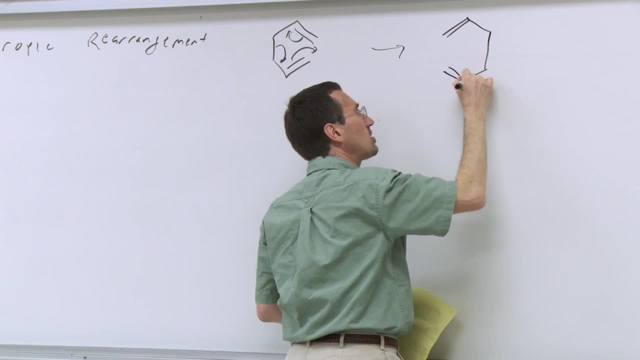 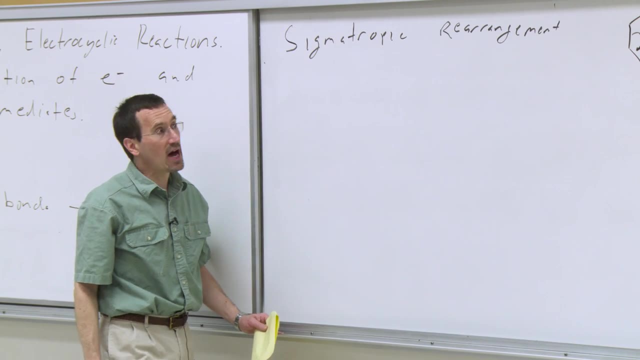 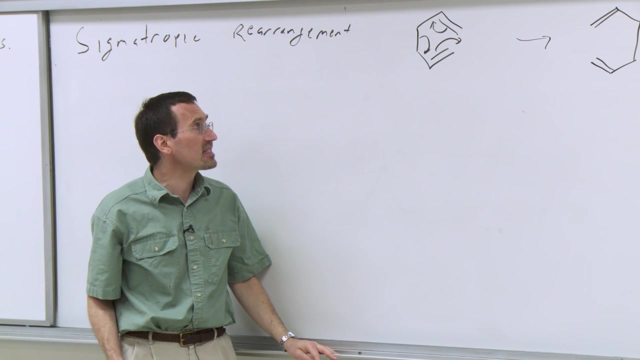 And, in this particular example, without any substituents, the reaction is degenerate, meaning that we started with a diene, we ended up with a diene, or, specifically, we started with 1,4, with 1,5 hexadiene. 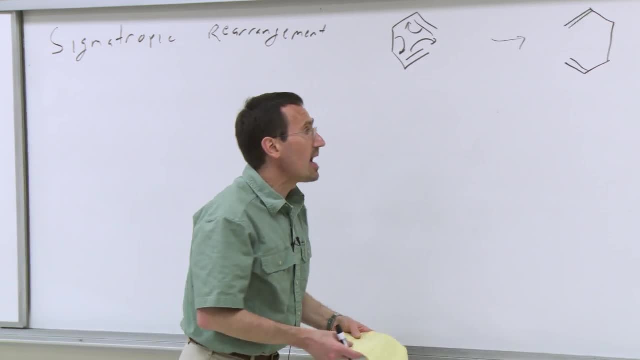 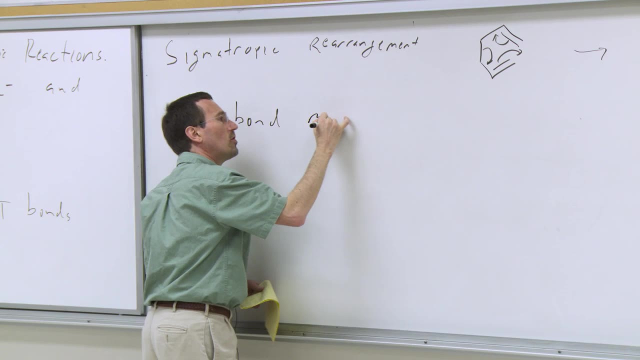 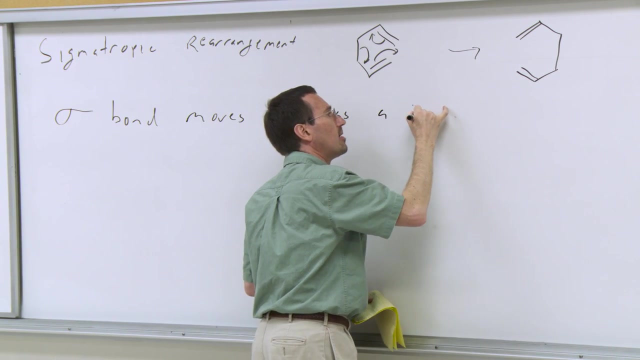 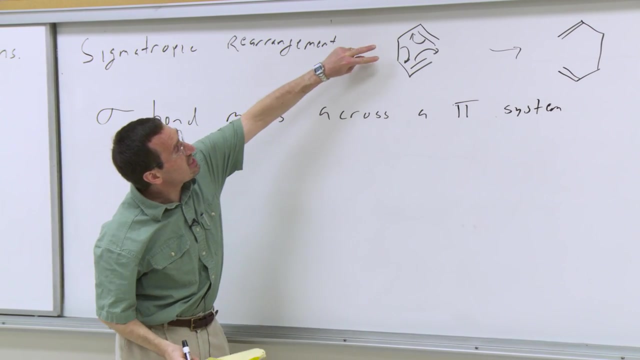 and we've ended up with a diene And we've ended up with 1,5 hexadiene. And what's the hallmark of this reaction is that a sigma bond moves across a pi system. In other words, you could think of this sigma bond here. 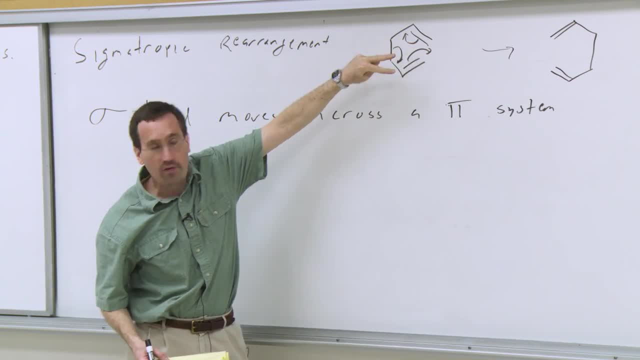 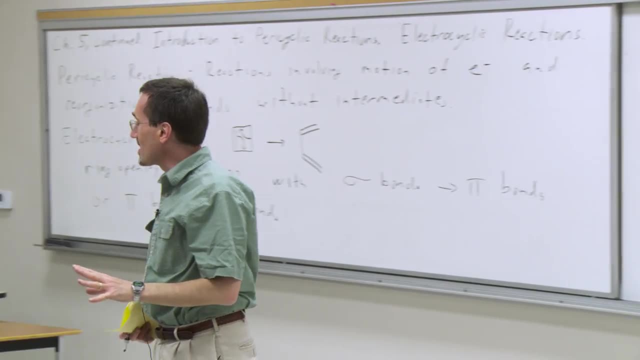 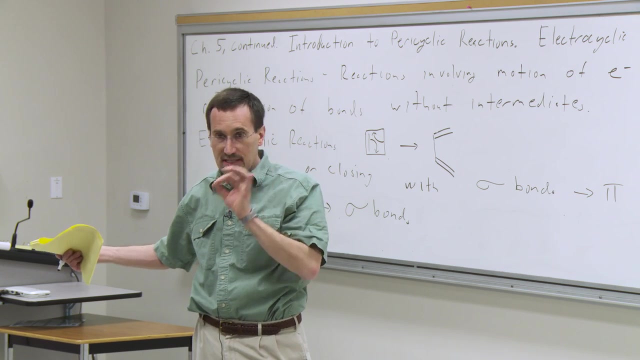 as skating over the molecule, over the pi system, And getting moved here- And that's a very nice metaphor for identifying a sigmatropic rearrangement- There's no change in the number of sigma or pi bonds. A sigma bond has simply moved. 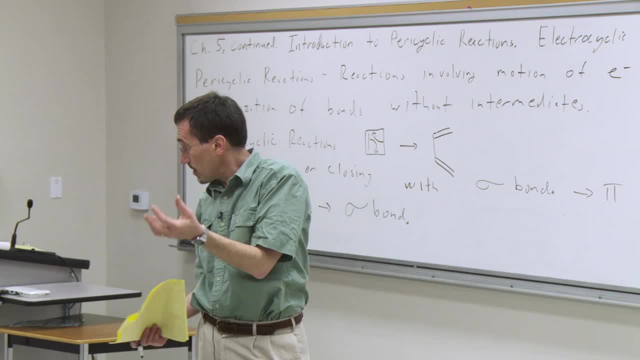 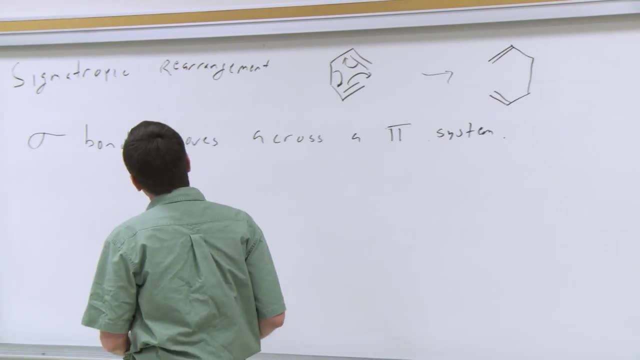 And that sigma bond can be between carbons, It can be between a carbon and a hydrogen And in all these cases, whether you're having a car, you can have bonds to oxygen. in all of these cases you can have bonds to oxygen. 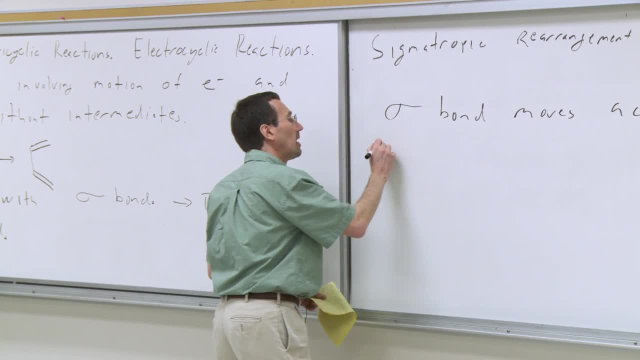 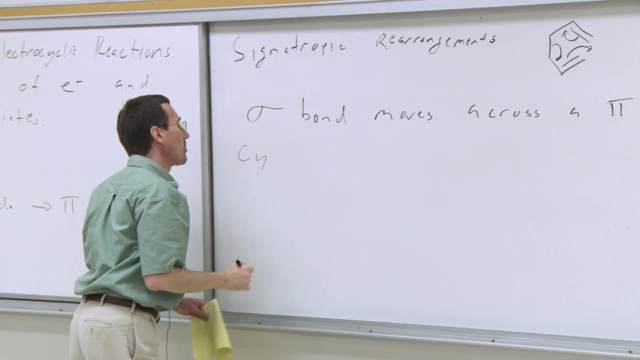 You can have bonds to oxygen So you can get this sort of basic skating motion. The last type of reaction is, I guess- since I'm trying to be consistent here, I'll write- sigmatropic rearrangements. The last type is cycloadditions. 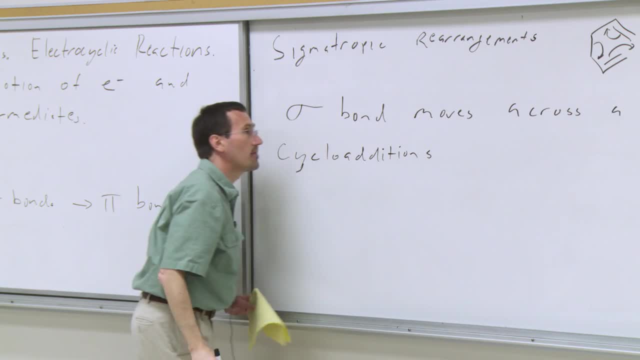 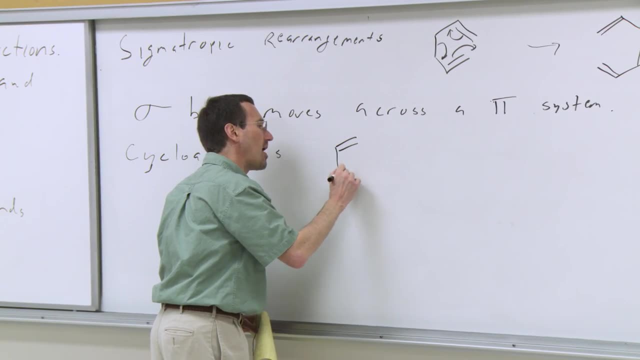 The last type of paracyclic reaction that we're going to talk about is cycloadditions. In cycloadditions, you're talking about bringing two pi systems together, Or the reverse: Sygmo-tropic- Sygmo-tropic. 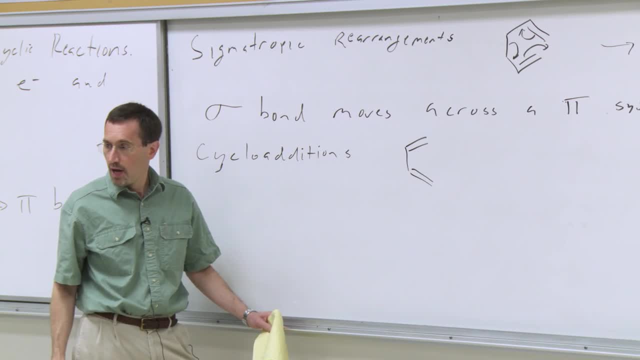 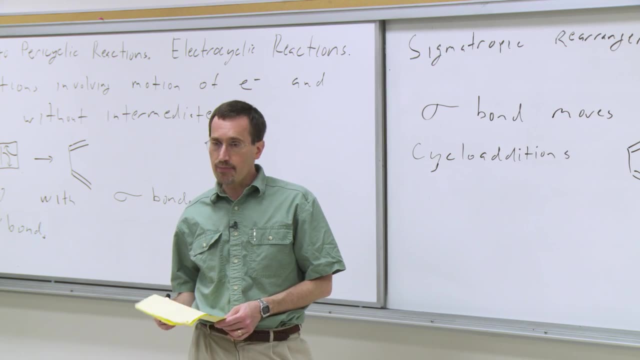 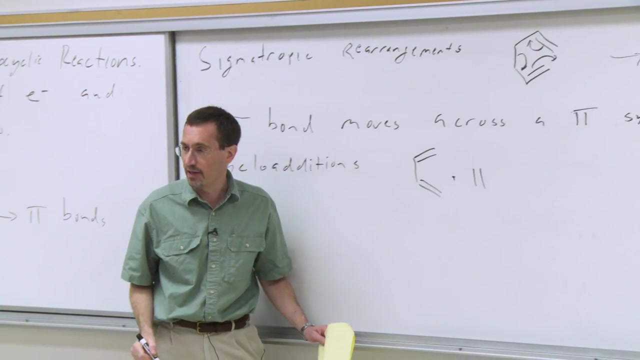 Sygmo-tropic. taking a system and breaking it into two, I'm going to draw a minimal drawing for a classic Diels-Alder reaction. Realize that in practice the Diels-Alder reaction doesn't occur with butadiene and ethylene to any appreciable extent. This is a common mistake that students 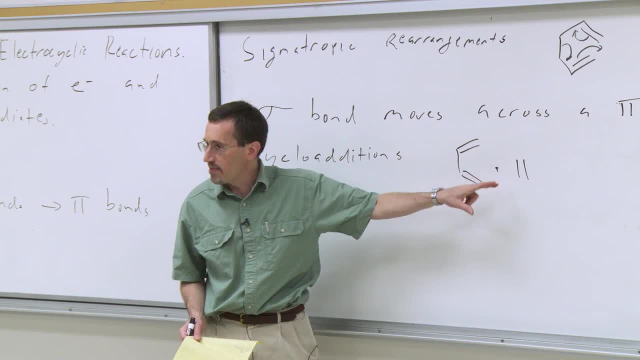 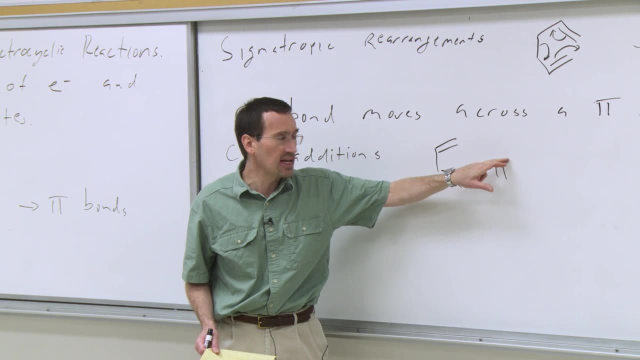 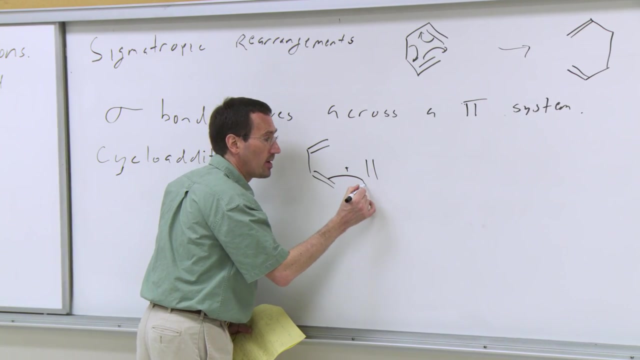 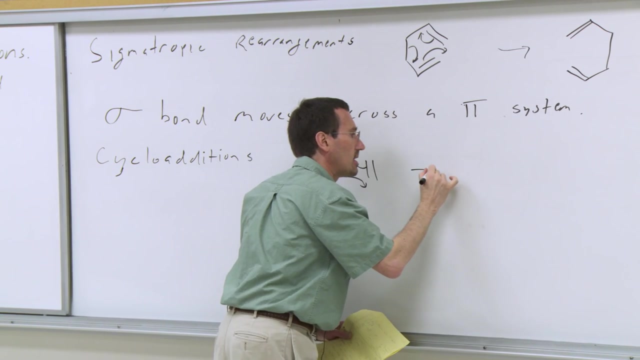 make, because often we as instructors draw the minimal structure and then people assume that that actual reaction occurs. Usually you would need, say, an electron withdrawing substituent on your alkene component, but I'm drawing the minimal representation of a Diels-Alder reaction here as an archetype of a cycloaddition reaction. 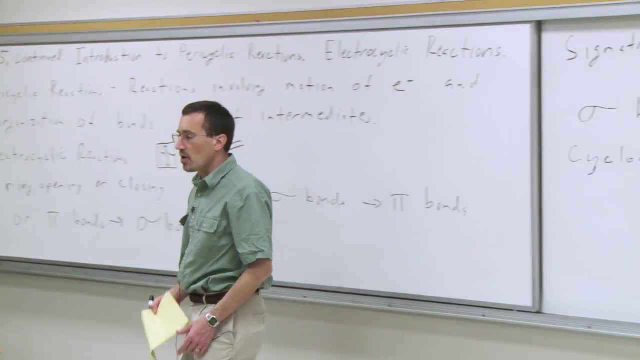 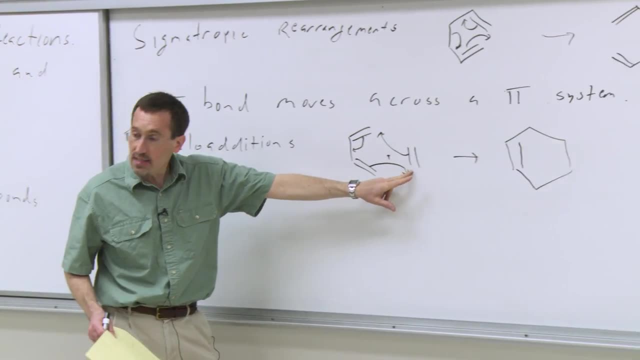 And so, if we want to describe this reaction, we've brought two reactions. One is a cycloaddition reaction and the other is a cycloaddition reaction. Two components together. We have a pi system here and a pi system here. They don't need. 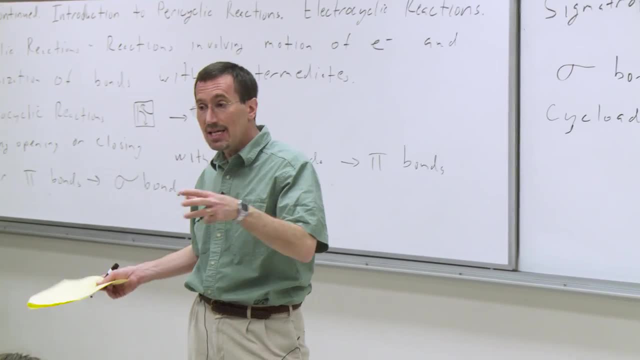 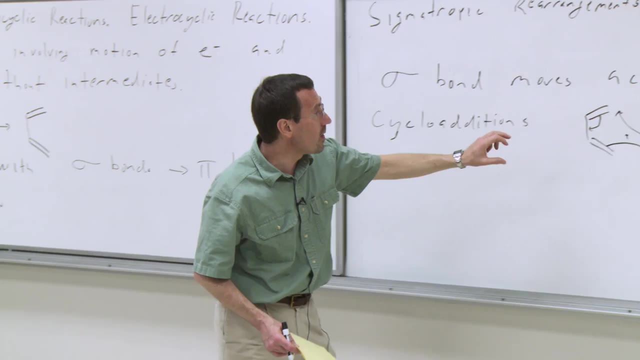 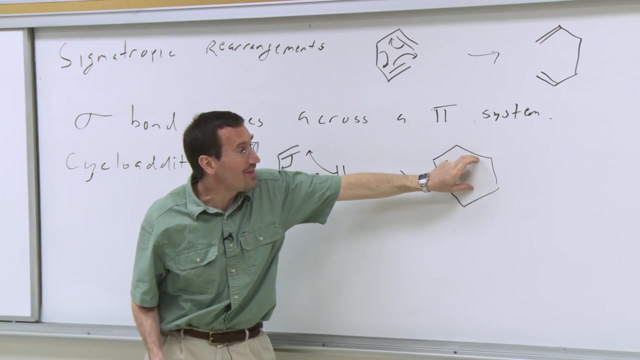 to be in separate molecules, but they need to be separate pi systems, even if they're connected by, say, a chain as a tether. And we've started with a number of pi bonds, in this case three- We're down to one. We've made new sigma bonds in the system, So I'll 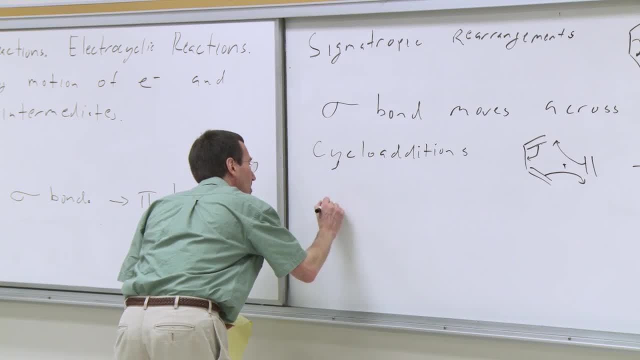 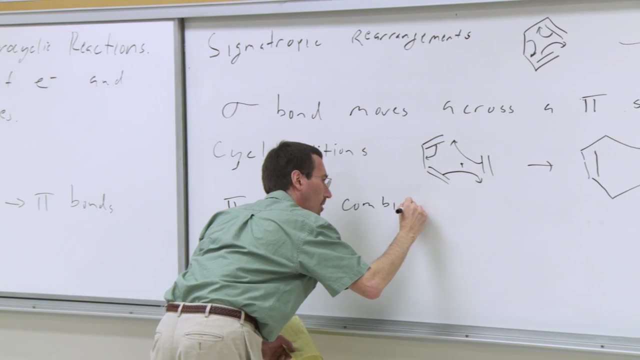 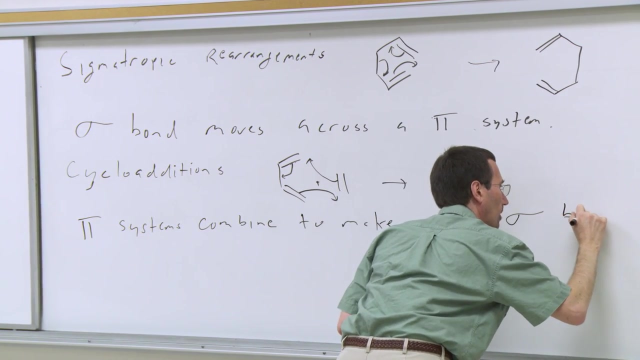 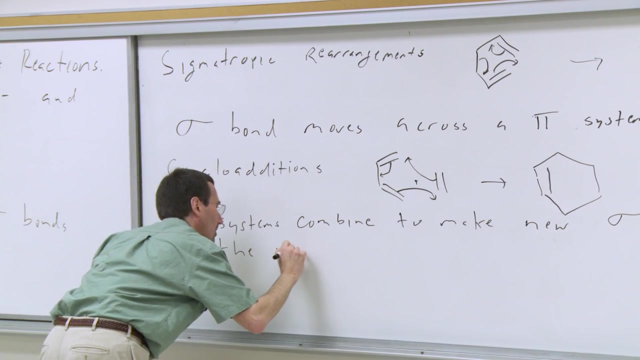 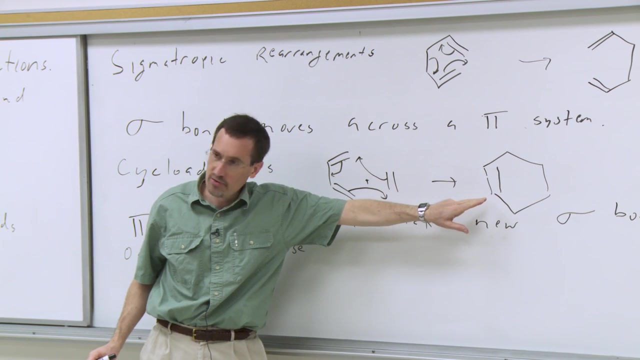 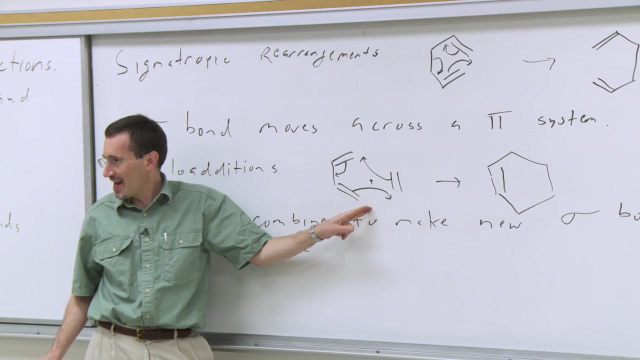 say, pi systems combine to make new sigma bonds or the reverse. and if you want to think about the reverse, just take this example. So if we were to take this arrow and flip it around, or alternatively, draw this cyclohexene on the left and draw butadiene and ethylene on the right, that would be called a retrocycloaddition. 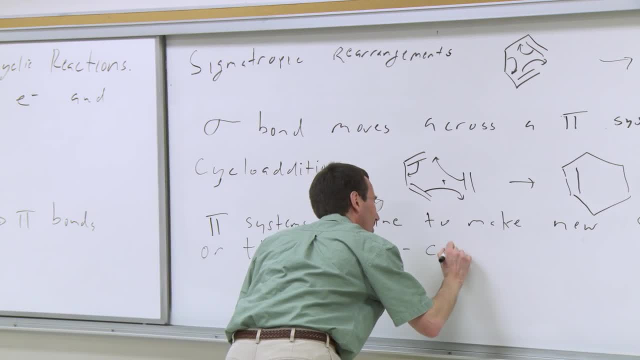 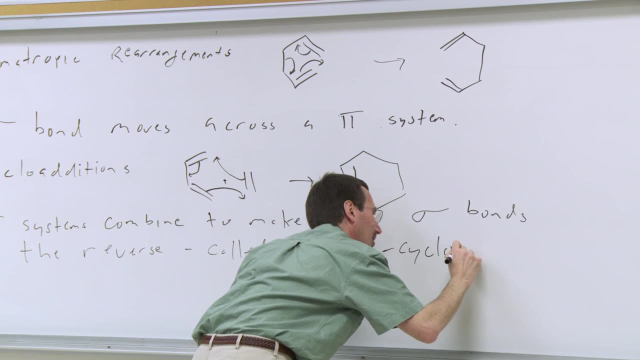 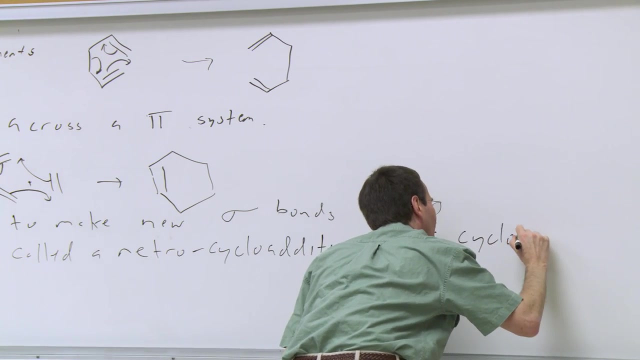 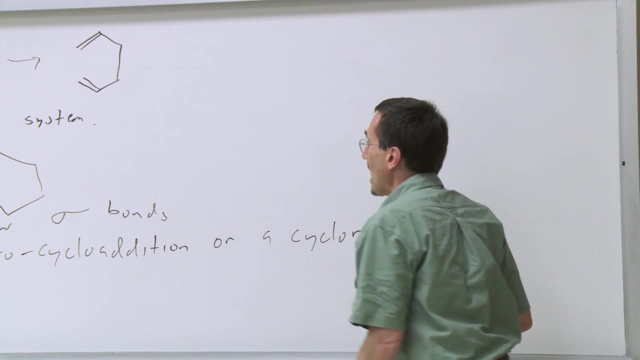 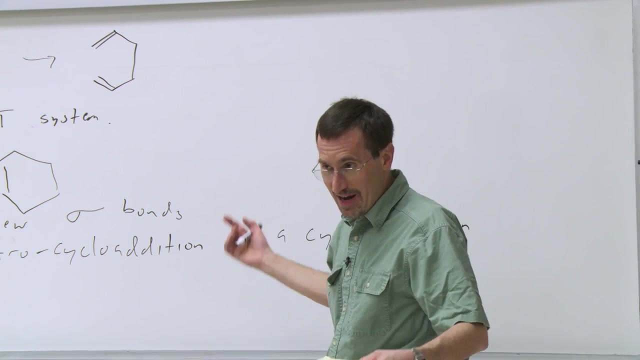 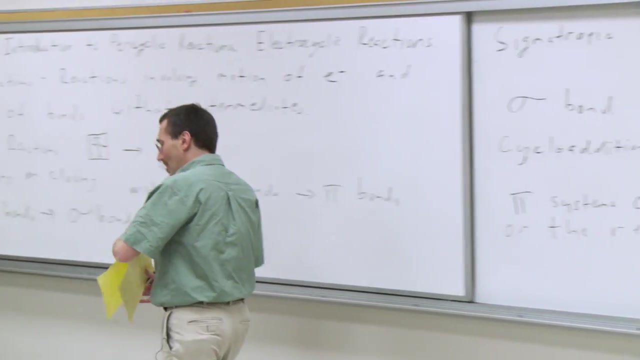 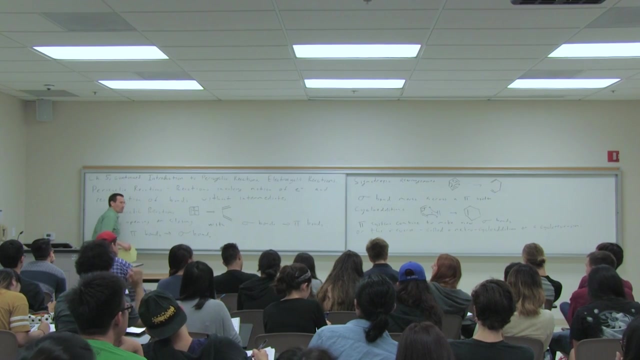 or a cycloreversion, And in that case, of course, it would be basically sigma bonds breaking apart and forming new pi systems. All right, Well, with that introduction, I want to dive right into electrocyclic reactions and show you some cool observations. Yes, 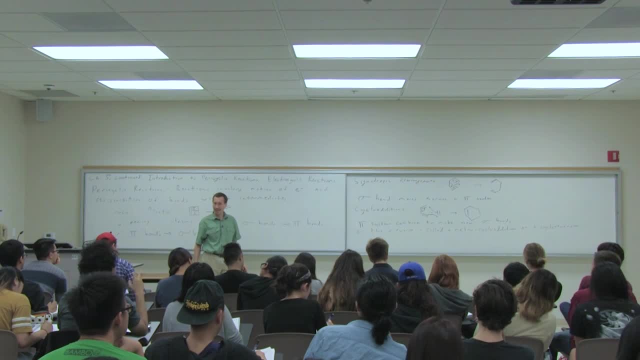 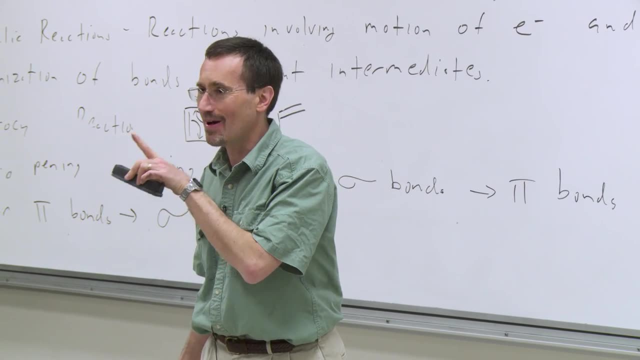 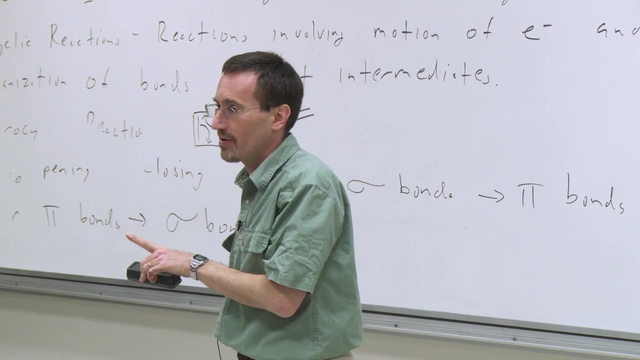 I'm just curious. but is the reverse reaction in equilibrium? Ah, beautiful question. Is the reverse reaction in equilibrium? Absolutely, And often that equilibrium lies way, way to one side or another, But we've got entropy working on our side. 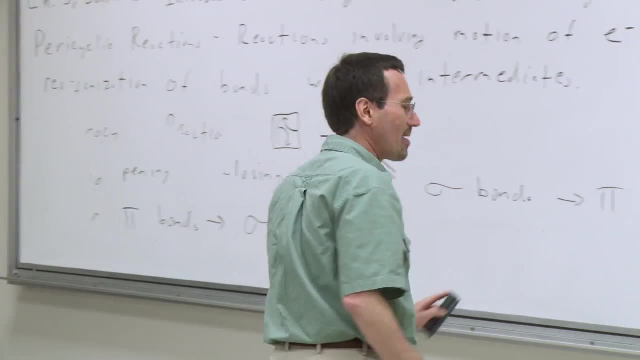 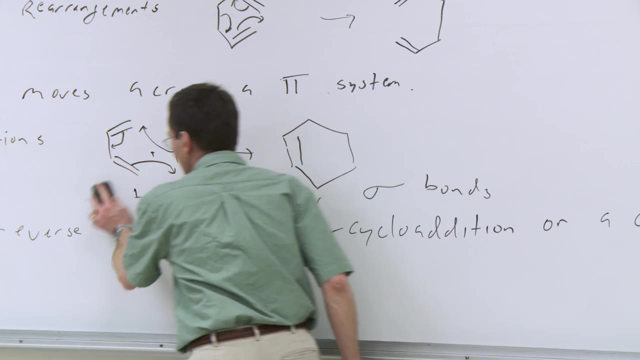 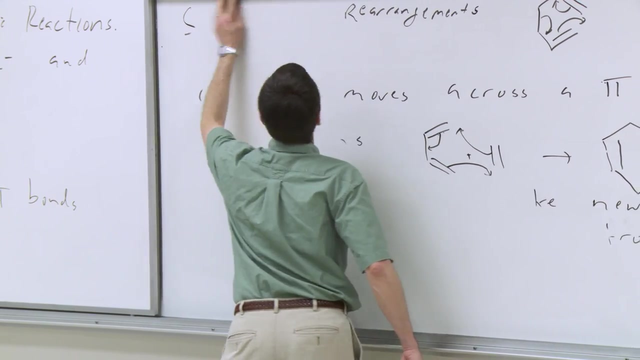 so often you can tweak that equilibrium. Yes, You can tweak that equilibrium with temperature. Did you in sophomore organic chemistry do a Diels-Alder reaction? What was your Diels-Alder reaction? Do you remember? No, no, no, But I mean, do you remember your reagents in your Diels-Alder? 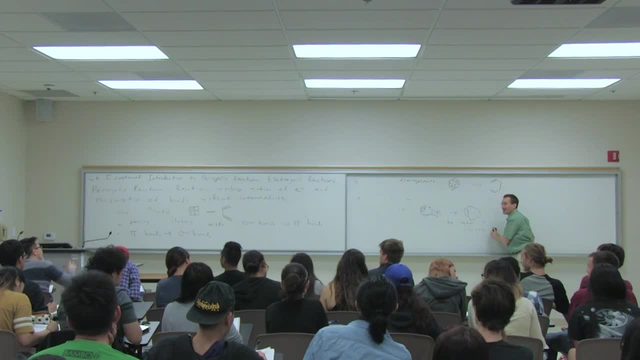 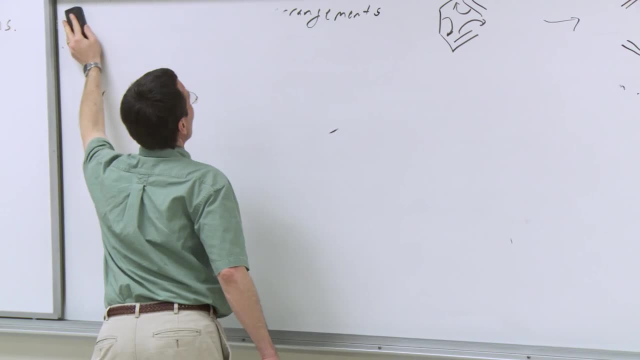 Not really Anybody remember. Uh, you had a diene and a dienophile. Do you remember the diene? Yes, What was the diene? The diene, The diene, uh, the name of it. Did it smell bad? 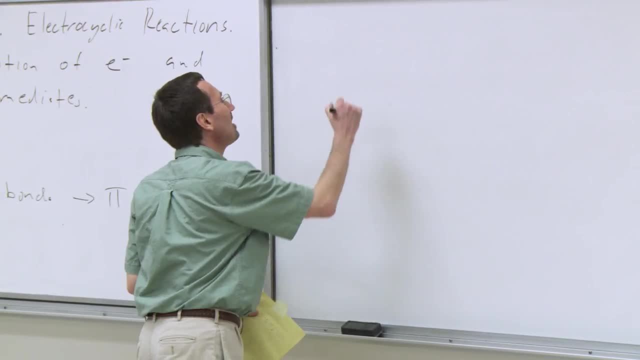 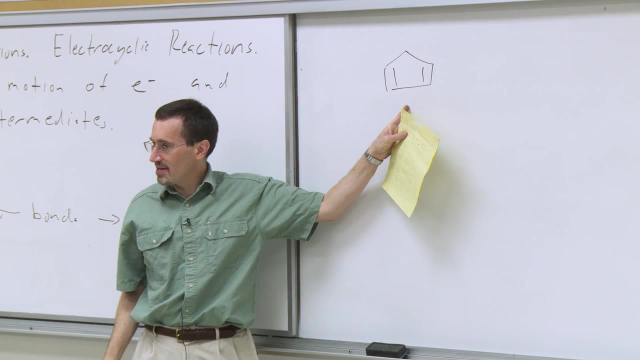 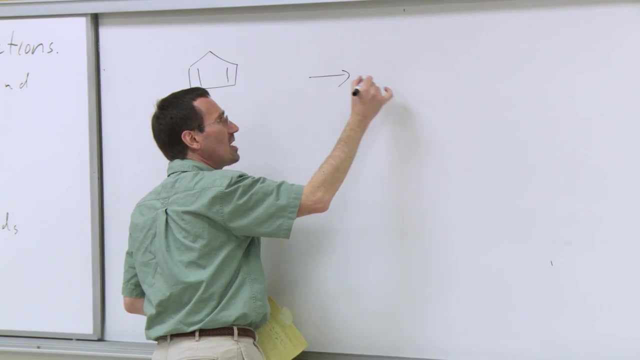 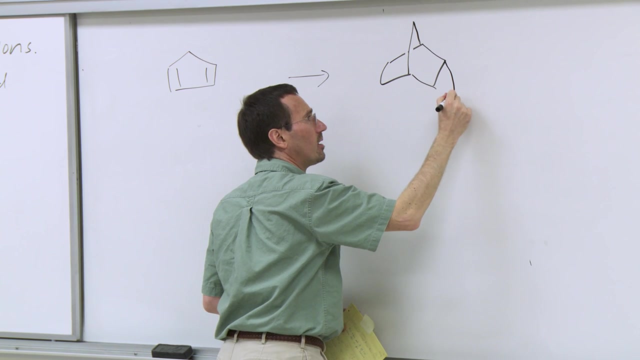 All right. The one that a lot of people do in sophomore organic chemistry is to use cyclopentadiene, often N-molaic, N-hydride Cyclopentadiene, if you just leave it alone with itself, undergoes a Diels-Alder reaction. you have a diels-Alder reaction. It's the. 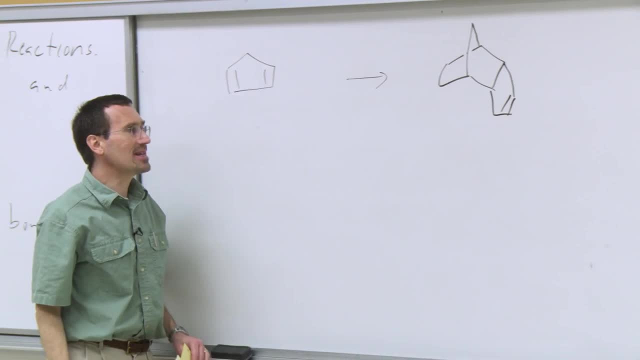 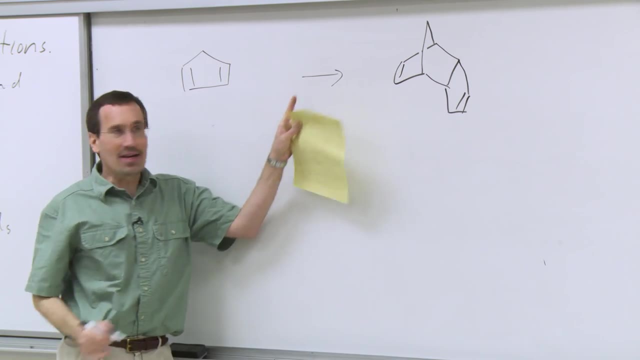 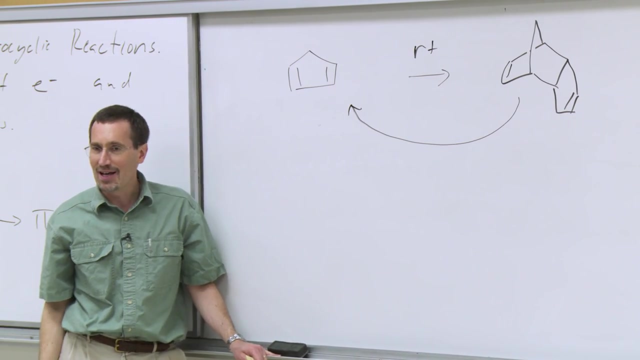 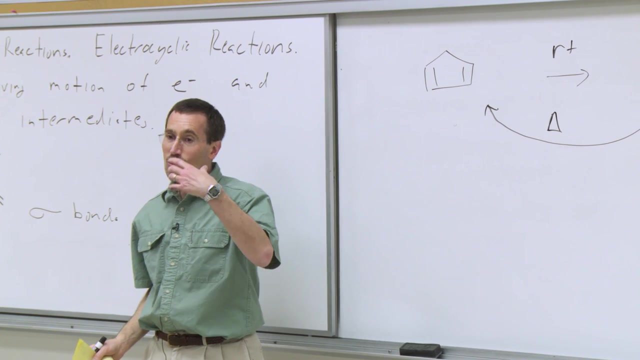 to what's called cyclopentadiene dimer or dicyclopentadiene. This occurs on standing at room temperature, But the way in which you generate- or maybe your TA generated- cyclopentadiene was you heat cyclopentadiene dimer and it cracks. 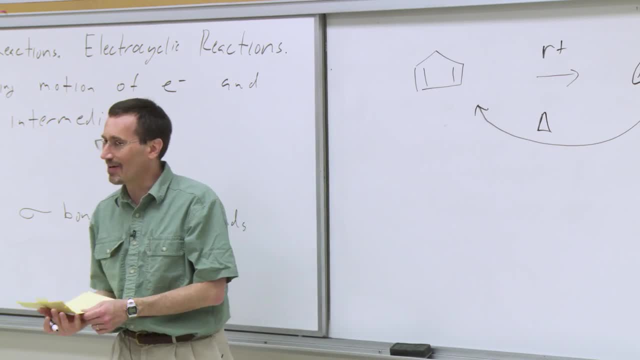 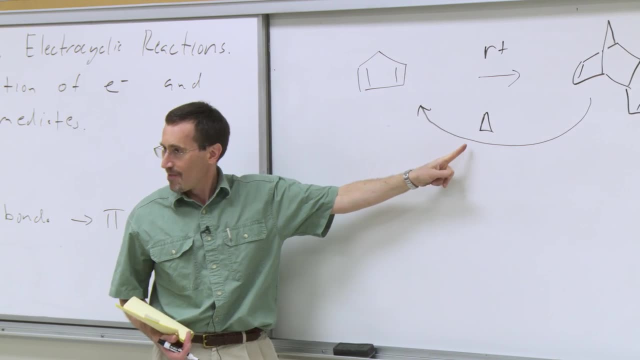 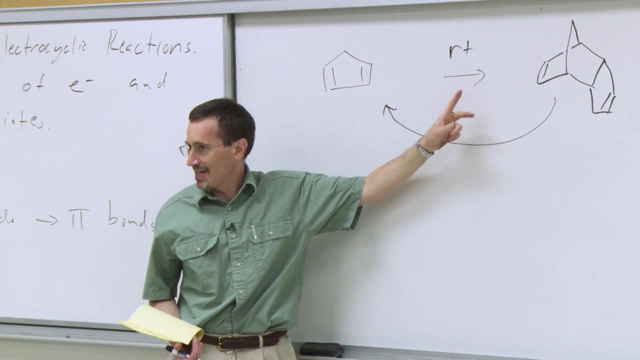 It undergoes cyclo reversion, retro cyclo addition, And so basically that T delta S term, at, say, 200 degrees Celsius, predominates and this equilibrium lies to the left. But at 25 degrees Celsius, your delta H term predominate and your equilibrium lies to the right. 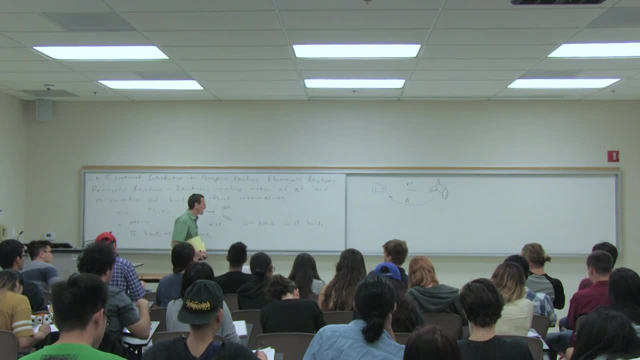 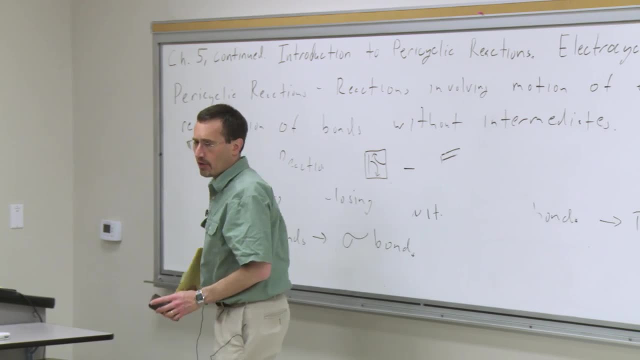 So you just need like enough energy to basically break those bonds. You need enough energy to break those bonds And, in general, sigma bonds are strong. They're stronger than pi bonds. In general, a pi bond is on the order of for carbon carbon. 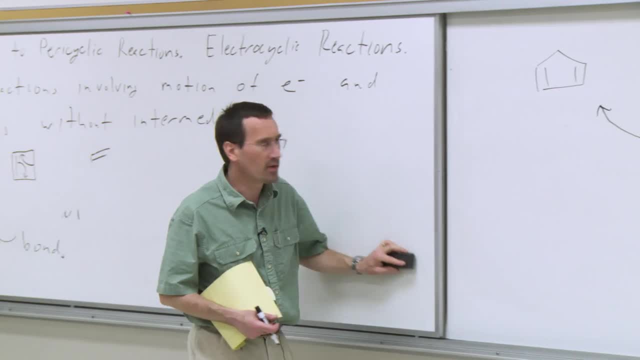 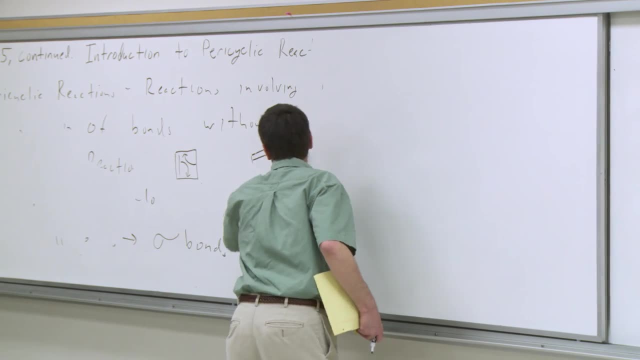 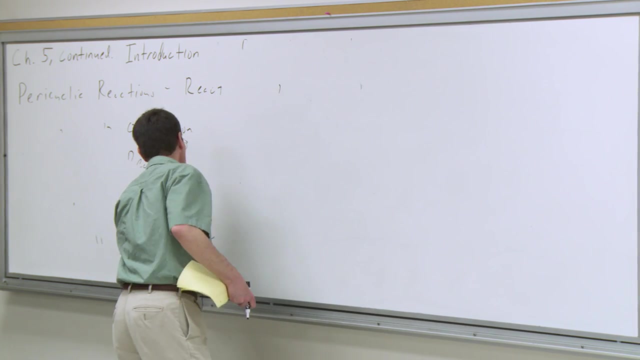 65 kilocalories per mole, give or take a couple, And a sigma bond is on the order of call it 80 kilocalories per mole, give or take a couple. So basically, you normally have a good driving force if you can get over the energy barrier. 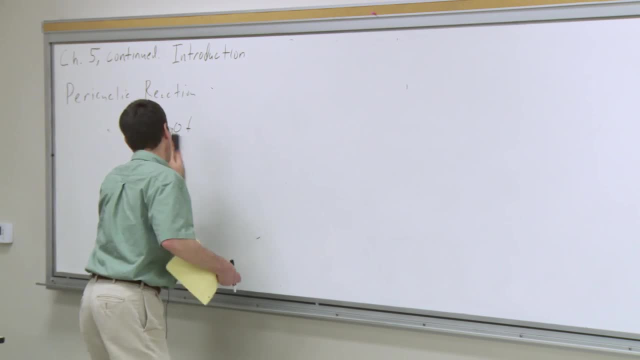 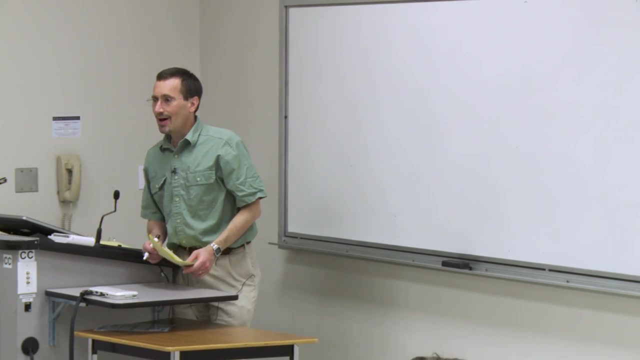 But if you have enough heat, that T delta S term, which is probably about I don't know, 30 EU or so on delta G, that T delta S term is enough to offset it. Other questions: I saw one other hand. All right, let us dive into electrocyclic reactions. 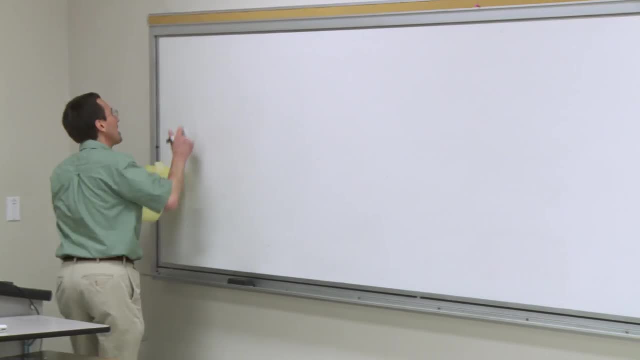 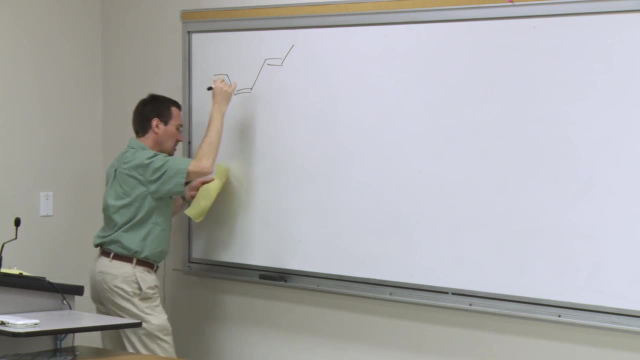 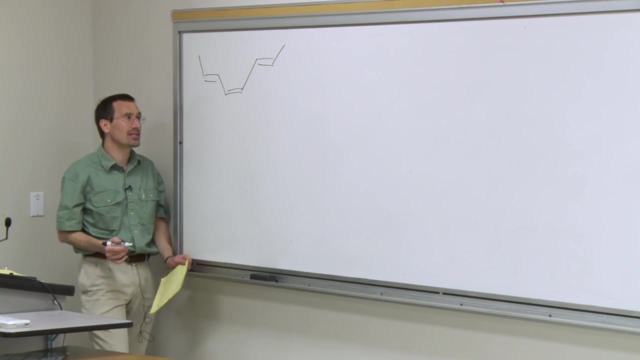 And I want to show you some cool observations and make some sense of them. All right, I'm going to give us two different trienes. These are octa trienes, and the octa trienes, of course, contain this archetypal hexadiene system. 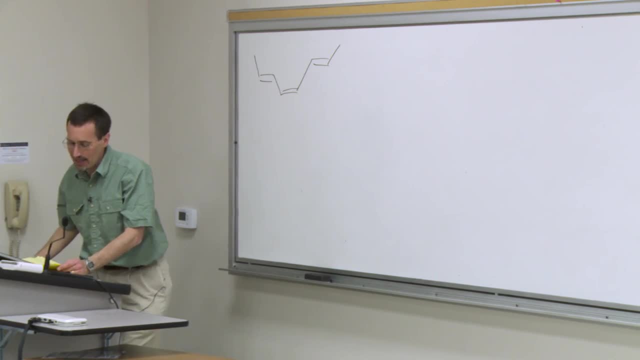 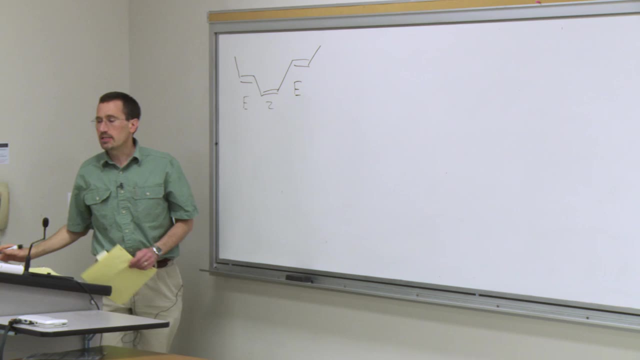 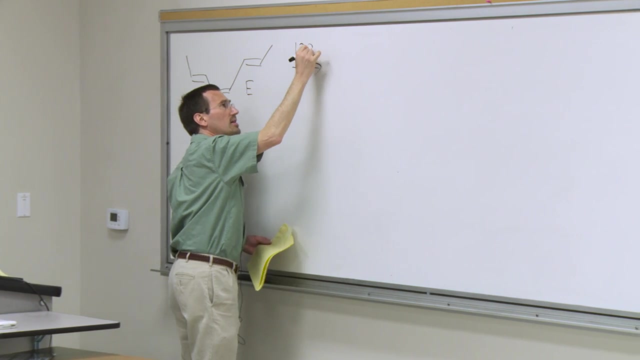 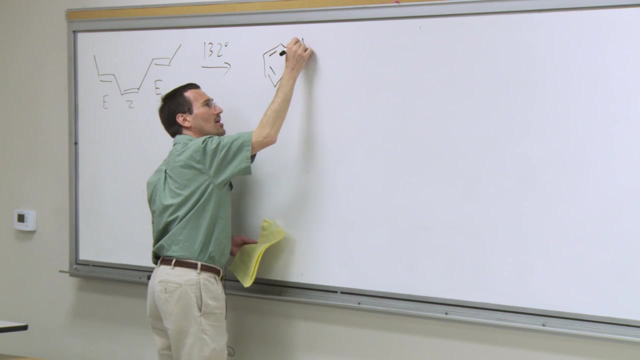 So this is 2,, 4, 6 octa triene and it is specifically the EZE stereoisomer. And when you heat at 132 degrees the EZE isomer, you get cyclohexadiene with two methyl groups. 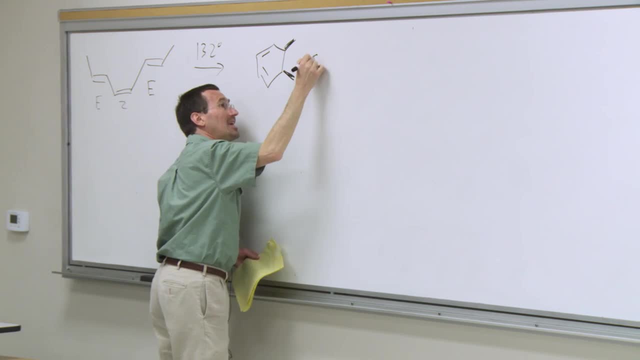 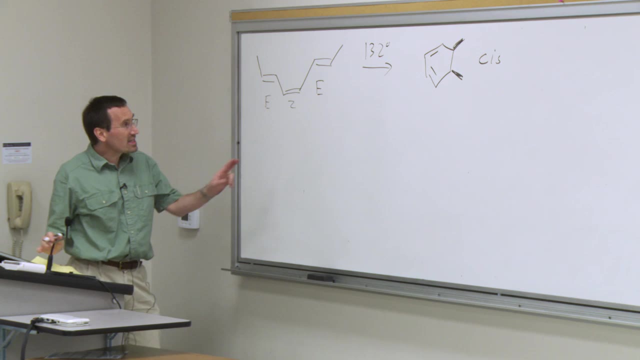 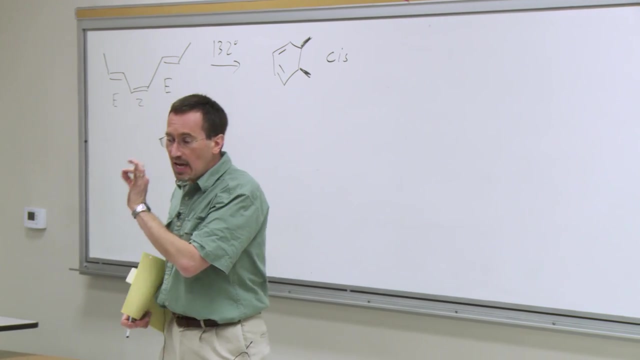 So that's the EZE, And then you have two methyl groups on it, And the key thing here is that the stereochemistry of those two methyl groups is cis. This is what we call a stereospecific reaction, The stereochemistry of the alkene, as we're going to see. 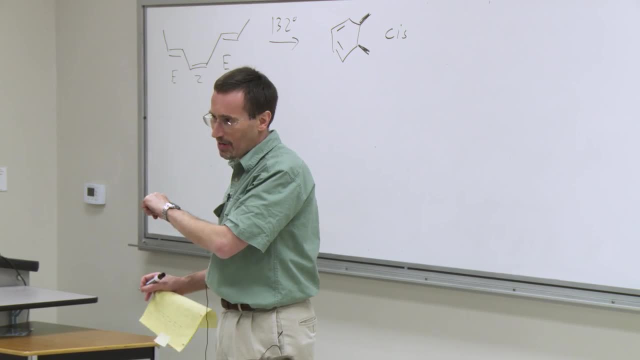 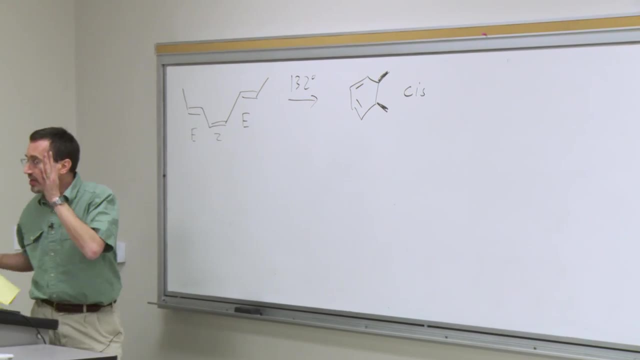 by the mechanism of the reaction dictates the stereochemistry of the product. The aldol reaction I showed you before was what we call stereoselective. There is a steric preference in the example we had for the phenyl group of benzaldehyde to go. 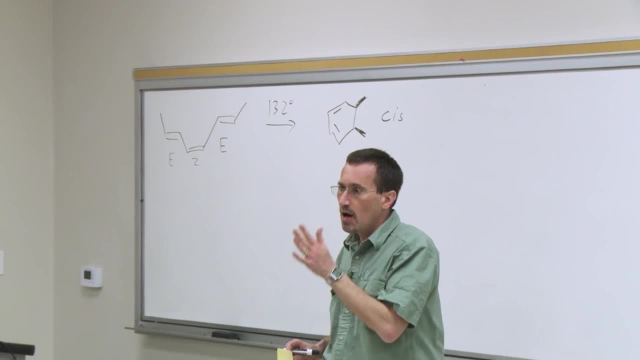 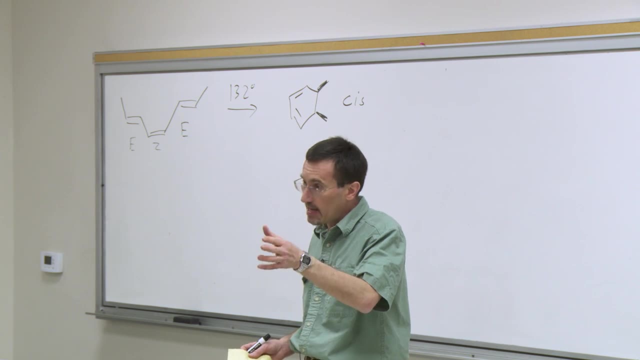 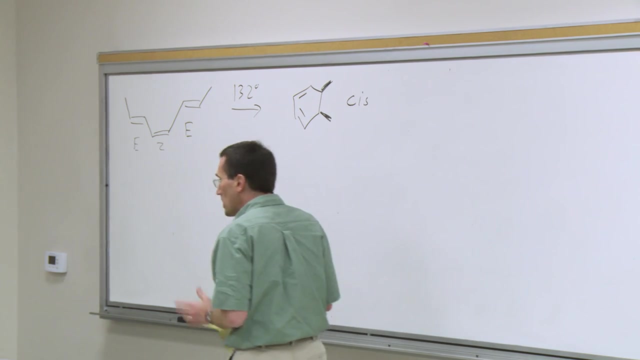 in the equatorial position on the transition state. But that is only a preference. That preference may be 99 to 1, depending on the size of the group you use. We used the tert-butyl group across from it. If you had a methyl group across from it, it would be lower. 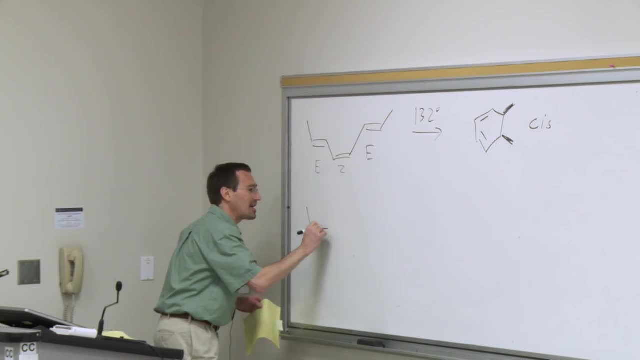 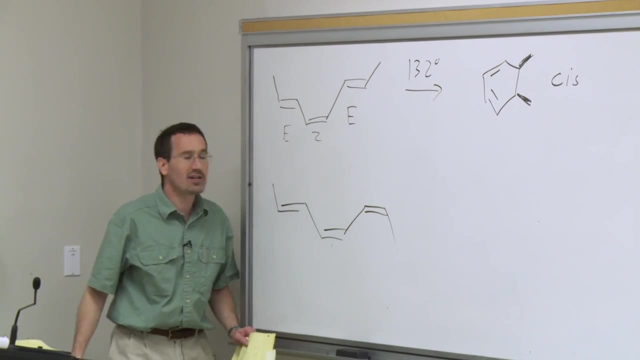 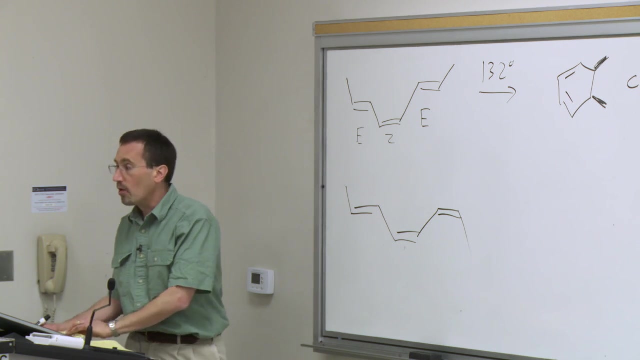 But it's not dictated by mechanism. Here it's dictated by mechanism And this caught the attention. It caught the attention of chemists like RB Woodward and Roald Hoffman, who became interested in explaining this, And Roald Hoffman won the Nobel Prize in 1981, along with 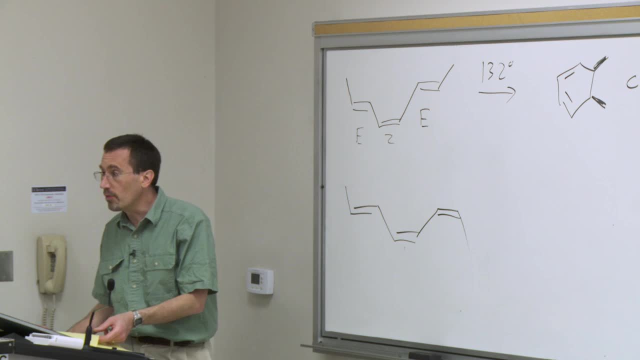 he shared it with Kenji Fukui for this. By that point, Roald Hoffman, RB Woodward, was dead, But the rules that we're about to see in paracyclic reactions are called the Woodward-Hoffman rules. Okay, 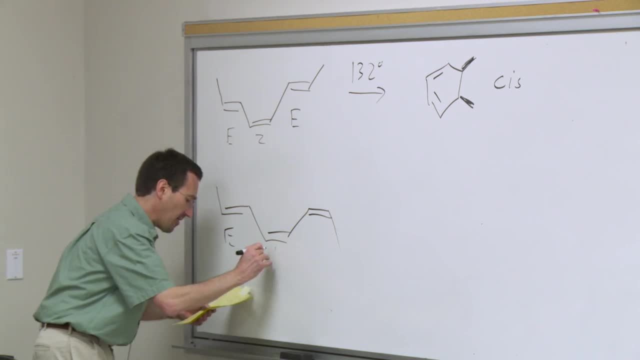 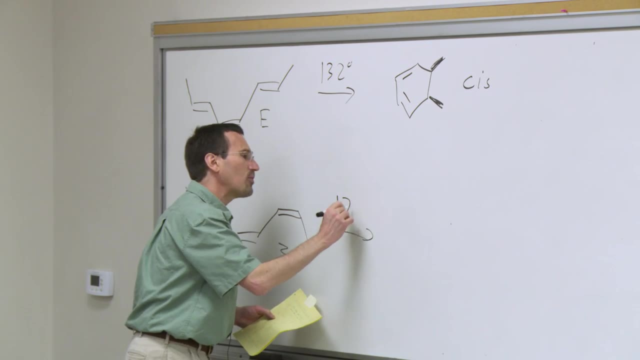 So let's go back. Let's go back to the empirical observations. If we start with the EZZ isomer of 2,, 4, 6-octetriene and we heat it up, we have to heat it a little bit more. 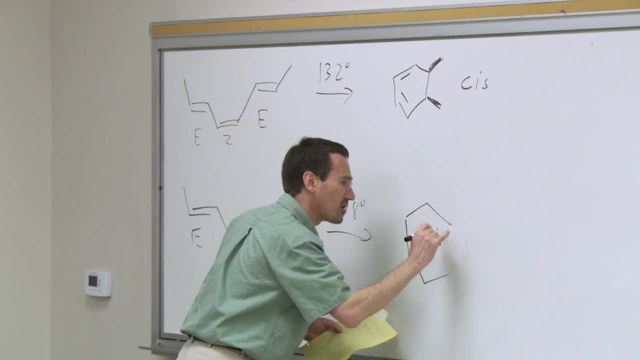 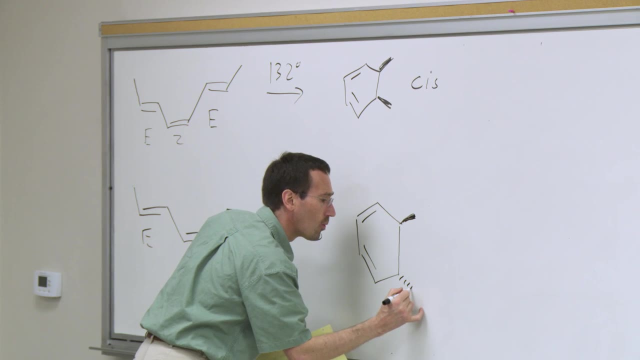 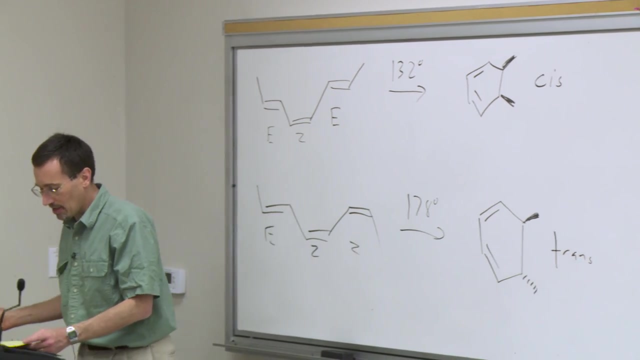 But don't worry about that difference. It's just the harder steric interactions of getting this more crowded transition state. What's key about this is we get the trans-stereoisomer rather than the cis-stereoisomer. Now, empirically, we can explain this in terms: 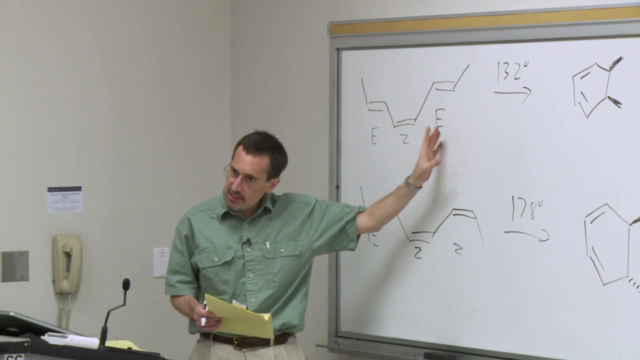 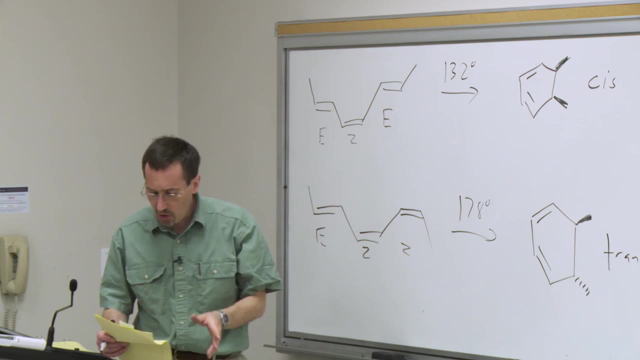 of what we observe. What we're observing, this is a 6.. We're going to come to the Y's in a moment, But what we're observing empirically is what we're going to call a conrotatory process. So I'm going to write this out. 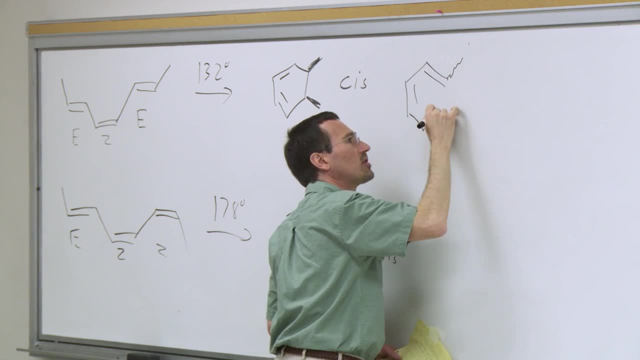 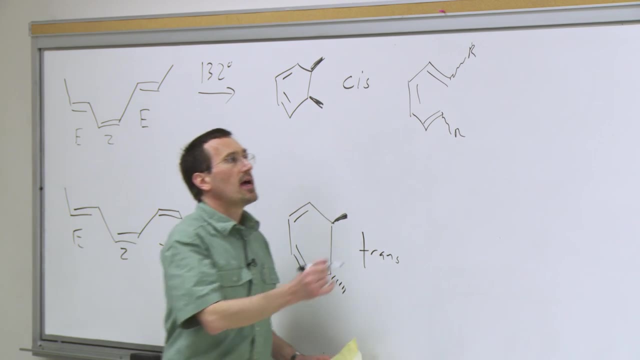 and I'll show you what I mean by the rotation. So let me draw a little squigglies here just to represent that I'm not yet specifying this. I'm just specifying the stereochemistry, And when we do this process, so we're going to call it a thermal. 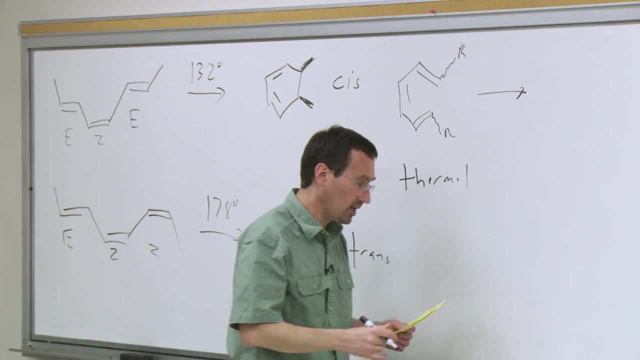 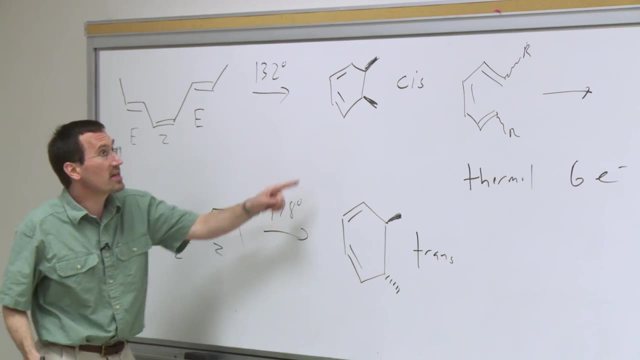 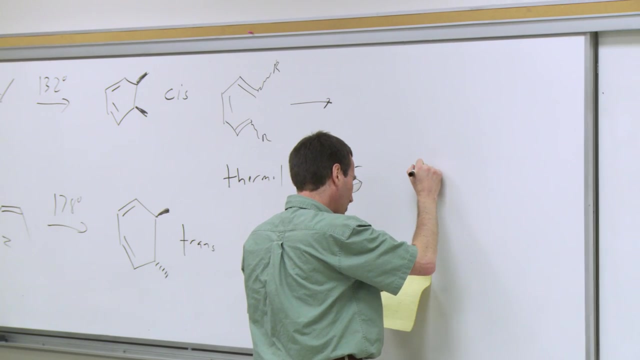 because this is occurring, not with light. We'll see photochemical in a moment. Six electrons, because we've got the 6 pi electrons here becoming the 4 pi electrons, and 2 sigma electrons, Thermal 6 electron. electrocyclic ring closure. 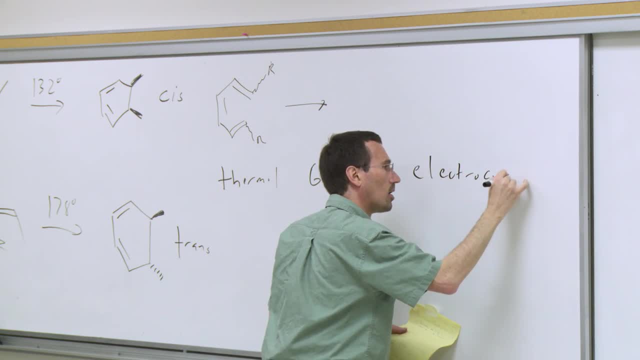 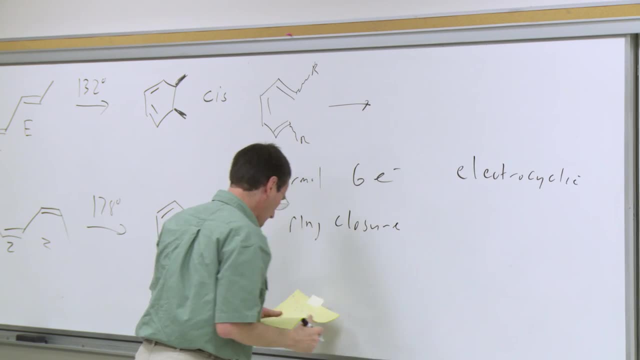 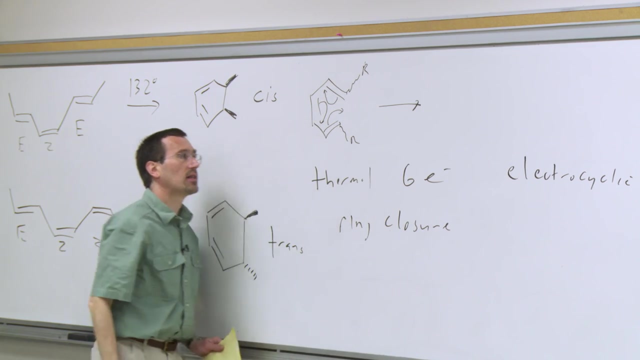 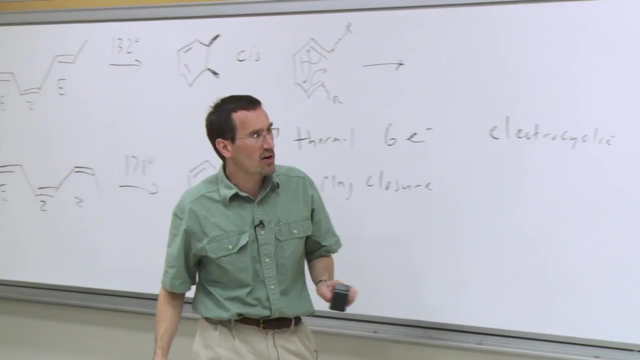 And what we're having here is our electrons moving in a ring like so. Now let us go to the specific stereoisomers. So that's the curved arrow pushing that I wanted to show you. Now we're going to go to the specific stereoisomers. 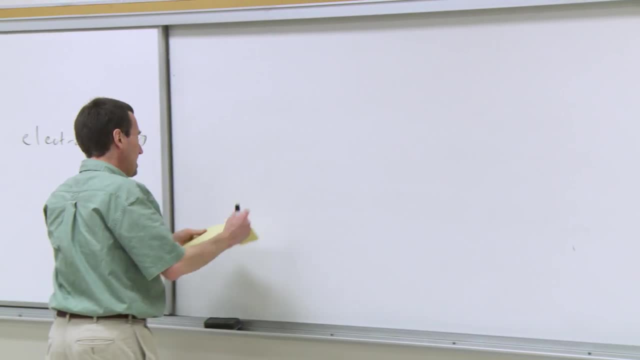 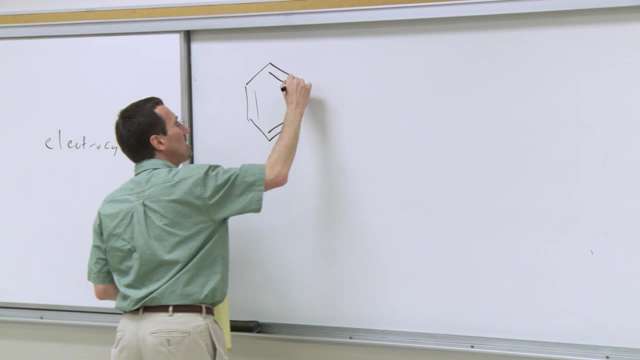 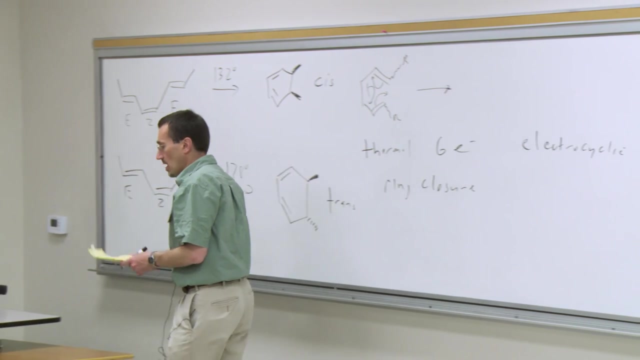 Now let's go to the specific stereoisomers and see what's happening in terms of motion. So we'll start with the EZE isomer, the EZE stereoisomer. And now what I want to look at is not the flow of electrons. 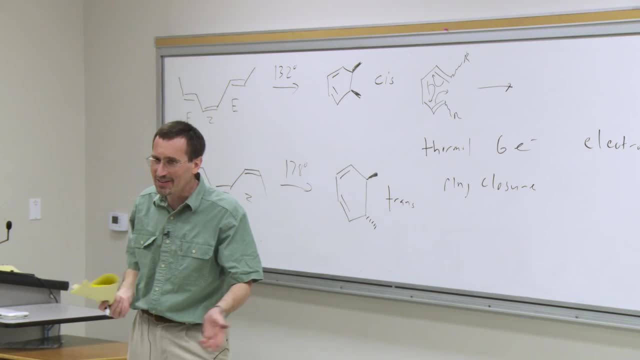 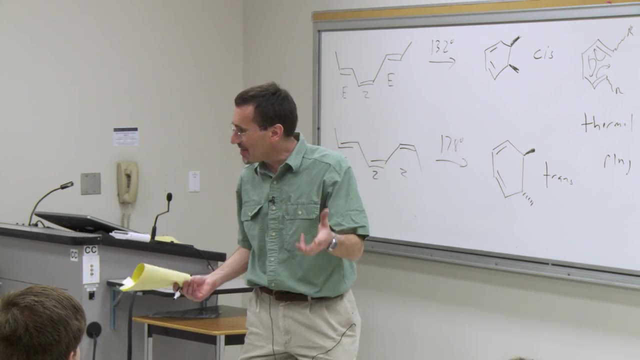 Organic chemists have arrows. We use arrows to show synthesis. We have arrows to show flow of electrons. We have arrows to show thinking backwards And we've got a lot of different arrows. We have arrows to show free radicals, But we don't have enough arrows to have a distinct arrow. 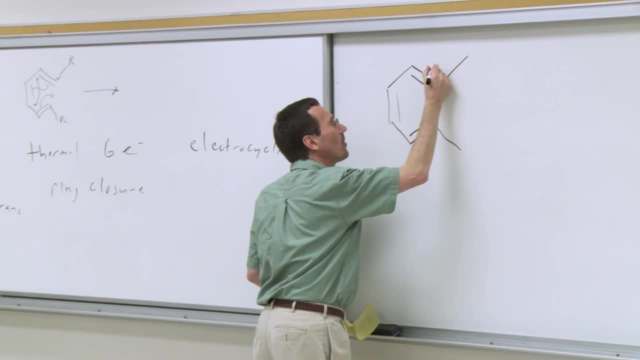 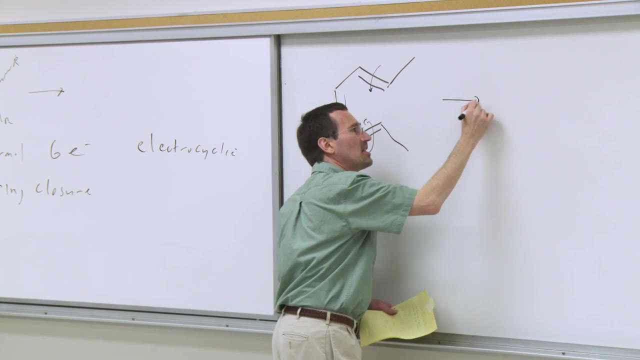 So I'm going to have to use the same curvy arrow, But what I'm going to do is now use it, alas, to mean motion, not flow of electrons. So we had the EZE, and that's becoming the cis. 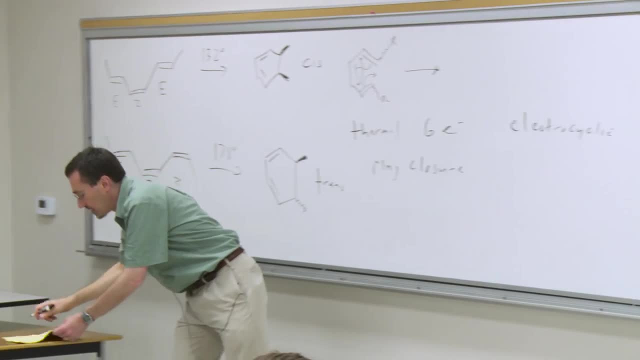 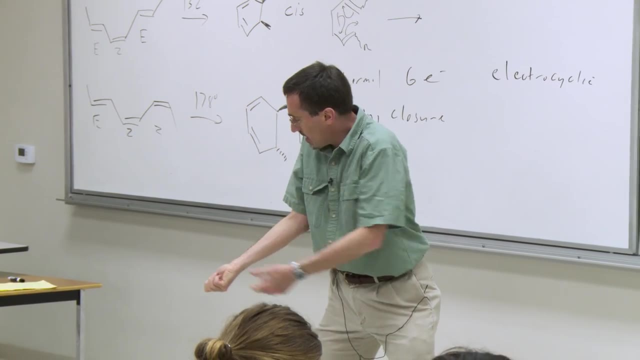 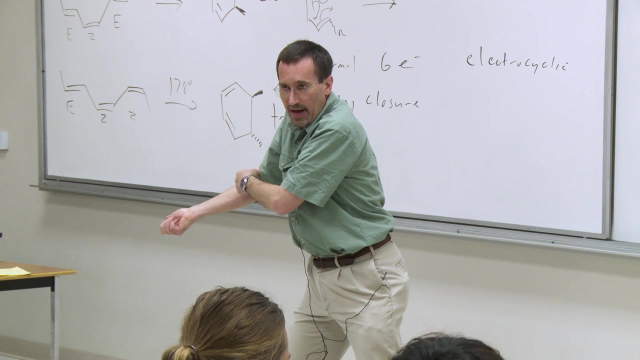 Now let us look for a moment And pretend that my hands and my torso make up that diene. In other words, this angle here, from my arm to my, from my shoulder to my arm, represents the single bond here and my thumb represents the methyl group. 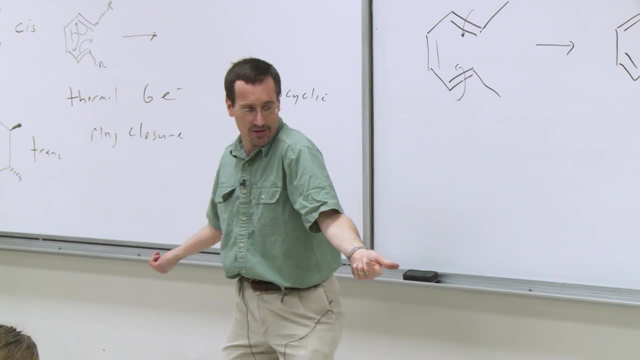 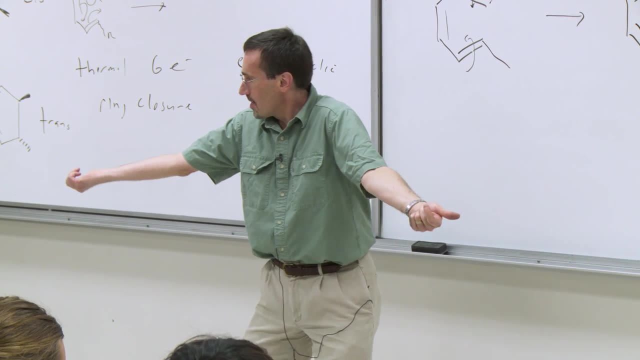 So I'm doing basically this one here And I'm going to do the same here. So these are our trans double bonds, our E double bonds. at the end- And I'm going to now bring my hands up- Remember, my thumbs- are the methyl groups- 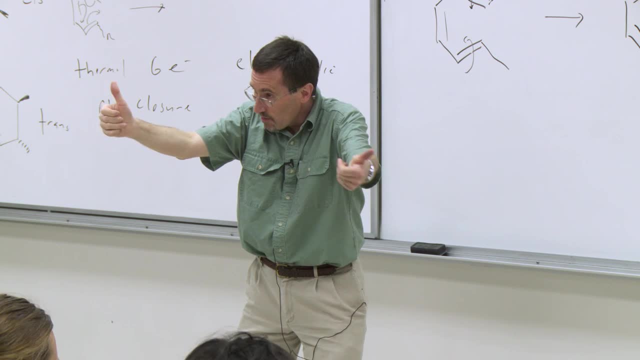 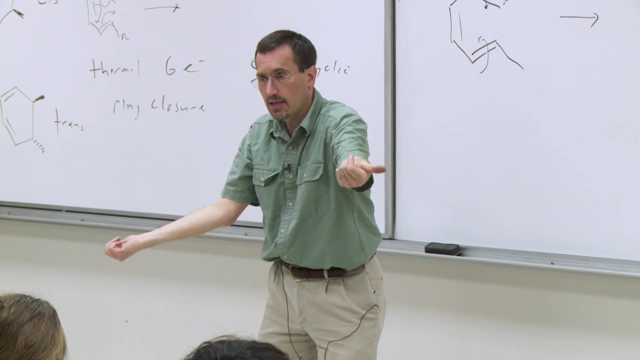 And we're going to rotate this hand as we form the bond And I'm rotating this hand counterclockwise for me And I'm rotating this hand as we form our bond And you notice that brings the two methyl groups to the same side. 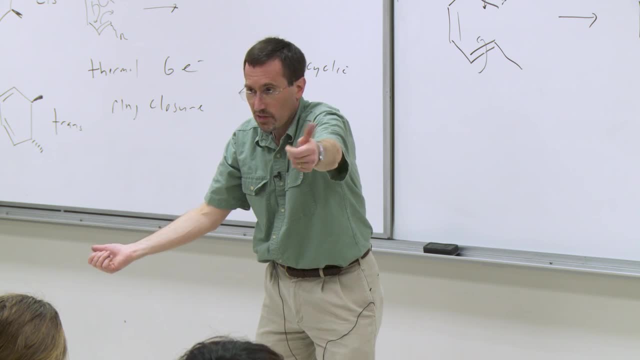 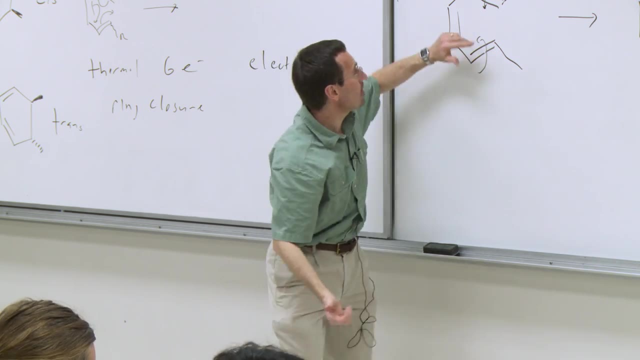 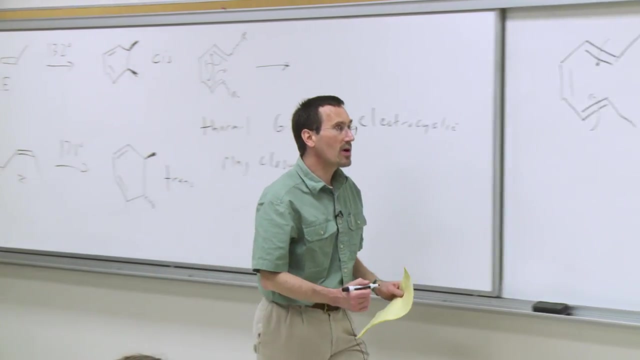 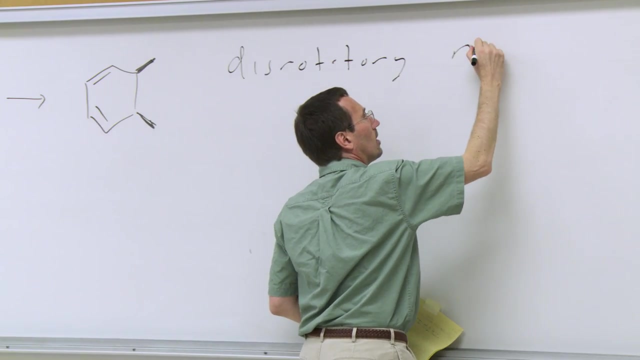 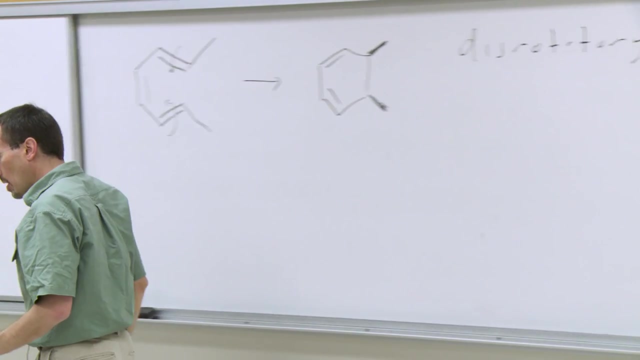 I rotate this hand clockwise for me. I rotate this hand counterclockwise. They're rotating in opposite directions as we come together. We call this a dis-rotatory process. So if we have a dis-rotatory process, then we end. 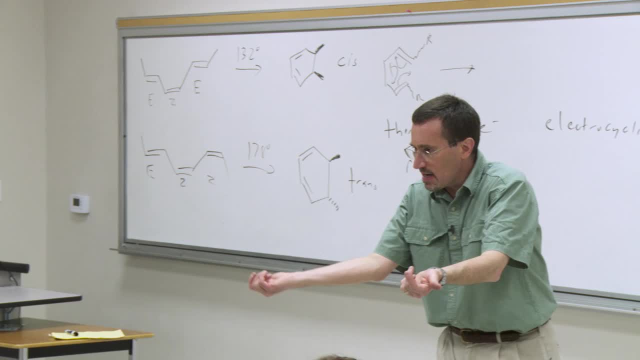 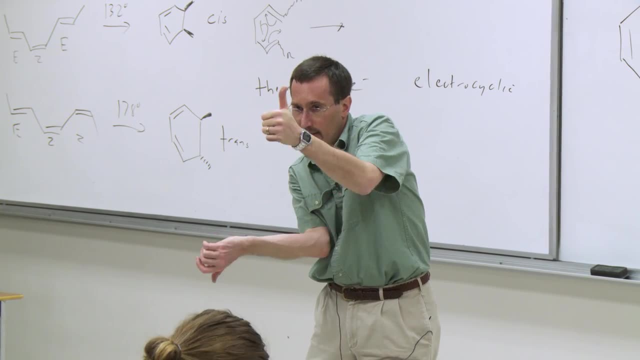 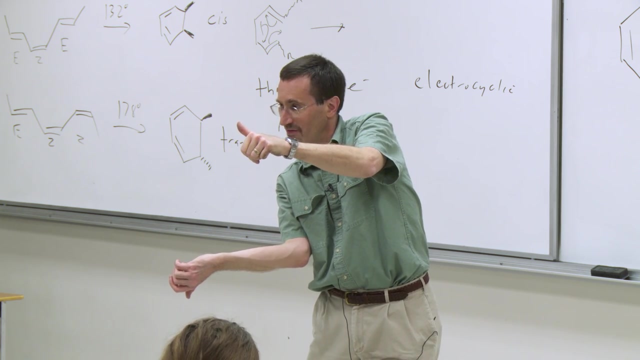 up with this. We end up with that cis geometry. If I had rotated both of my hands clockwise now, I would have ended up with one methyl pointing up on the cyclohexane ring and one methyl pointing down, So con-rotatory would have led to trans. 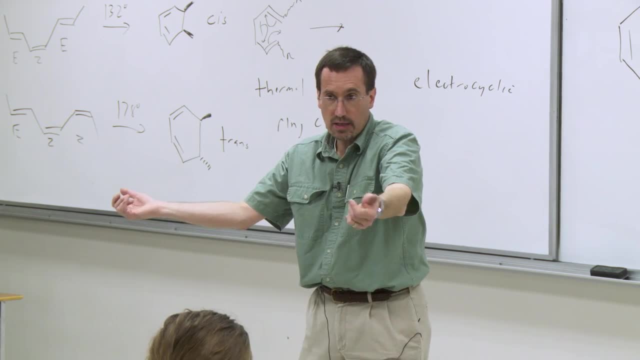 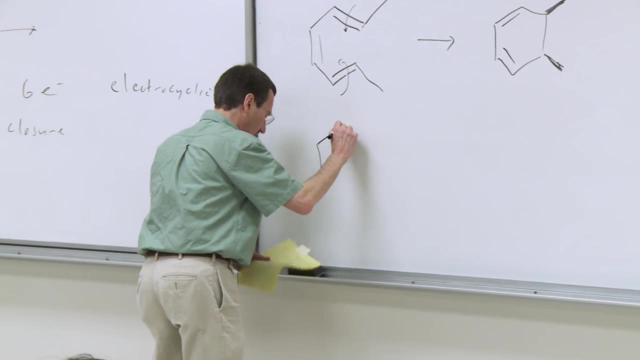 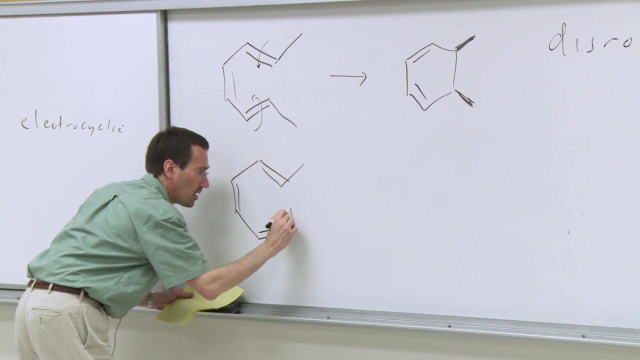 but we're seeing dis-rotatory clockwise and counterclockwise, And we see that exact same principle in the other stimulus. So I'm going to now start with the other stereoisomer. Now I have to point this methyl group inward. 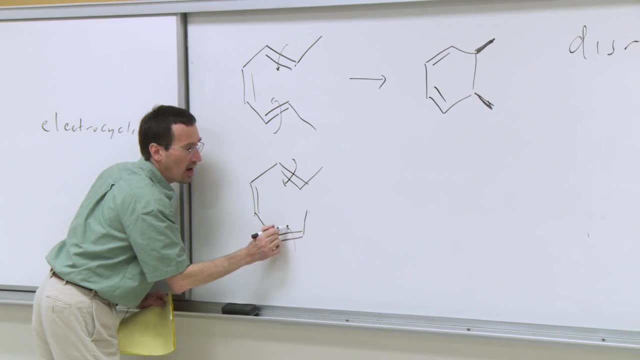 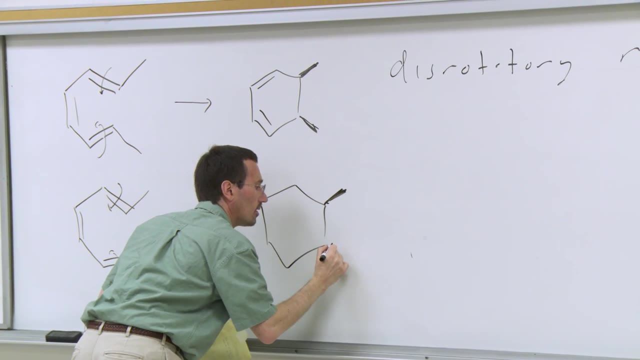 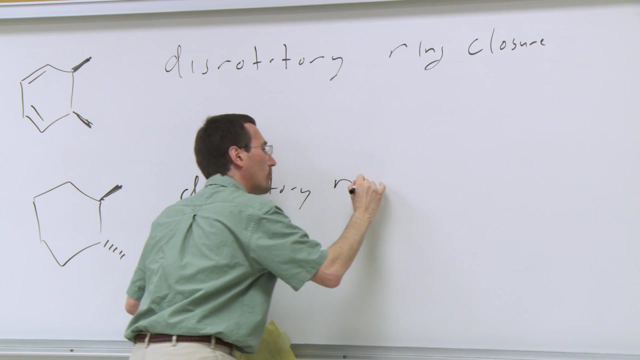 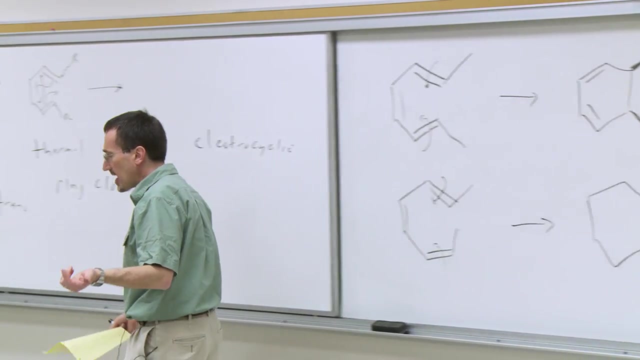 And again we're going to do: one rotates clockwise, one rotates counterclockwise, And again this is a dis-rotatory. So I'm going to try to show you that And I'll try to show you that as best as I can with my arms. 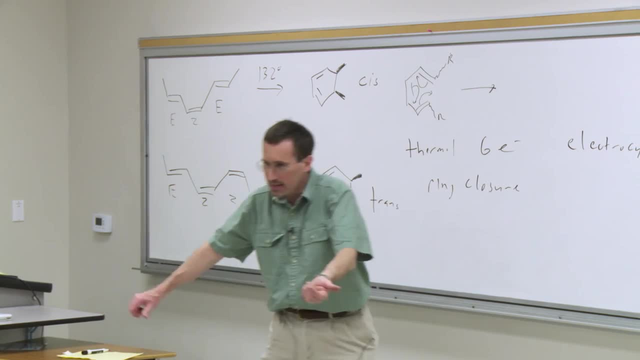 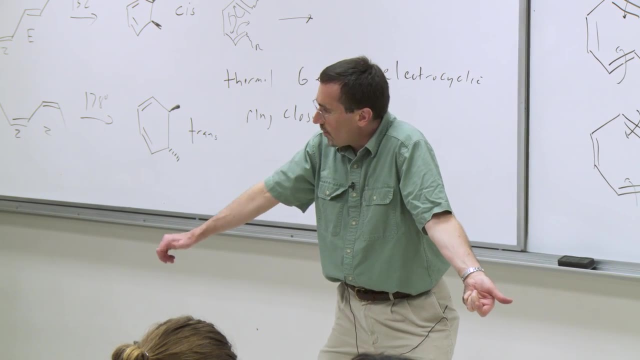 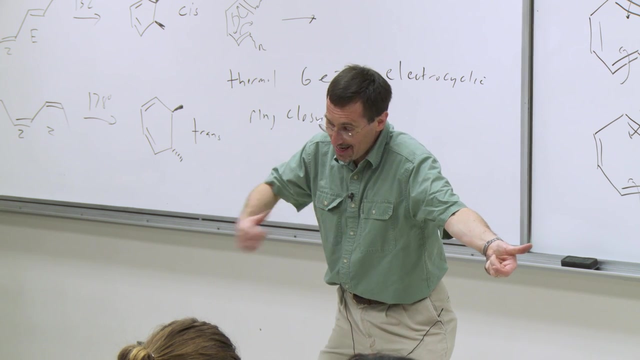 I may end up getting some sort of wrist injury in the process. All right, So before here was the EZE, Now I'm going to make one of those Z. So we have the E over here, the Z here And the Z. 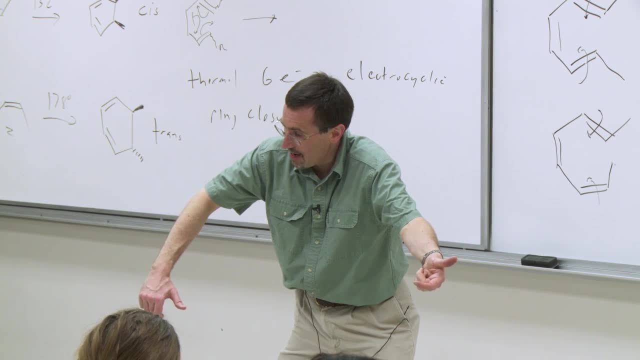 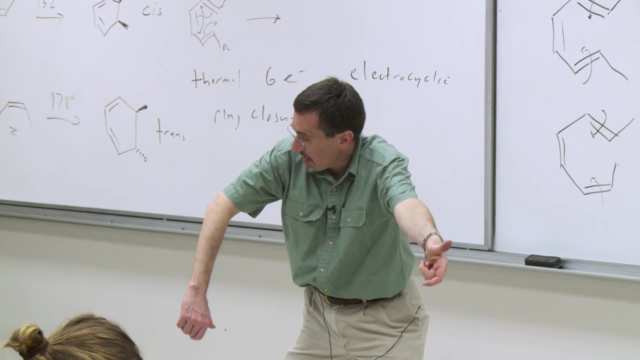 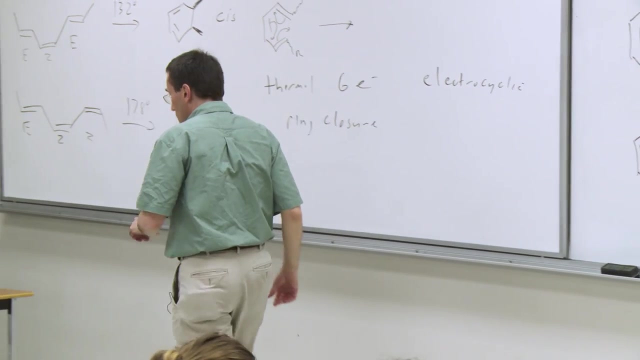 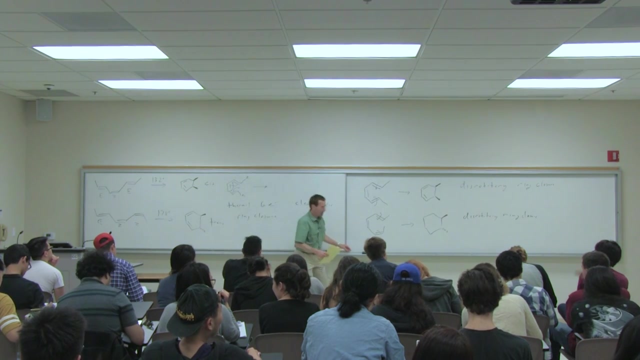 And now, when we again rotate in opposite directions- this hand going clockwise for me, this hand going counterclockwise. now those methyl groups end up on opposite sides. So that's your dis-rotatory motion. Yeah, Going back to that EZE and the Z. 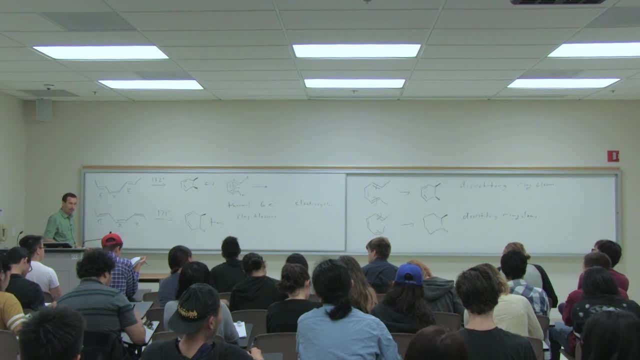 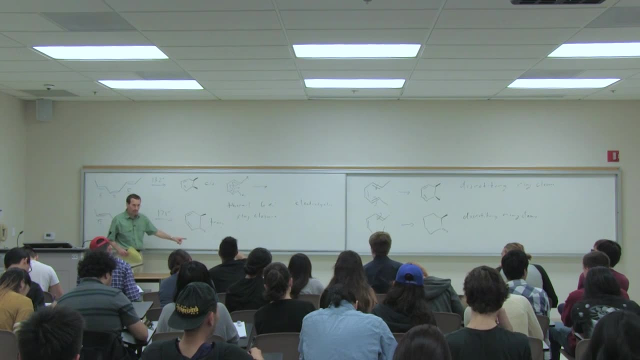 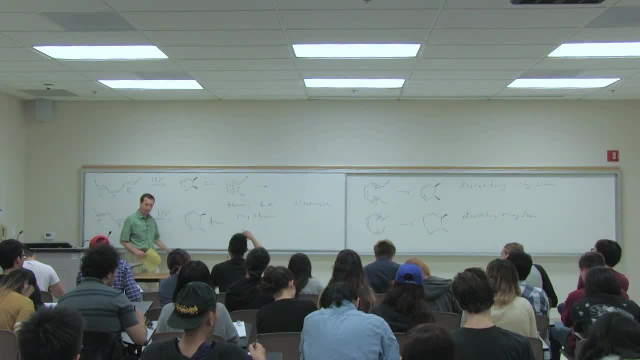 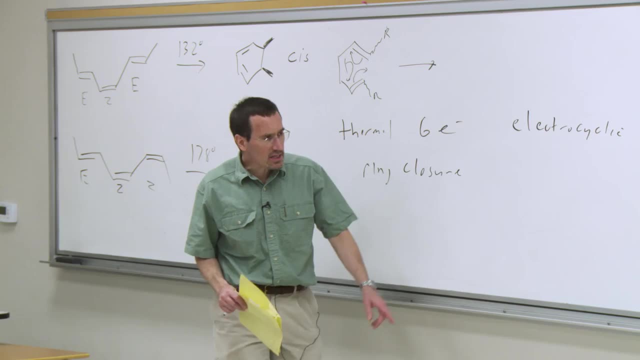 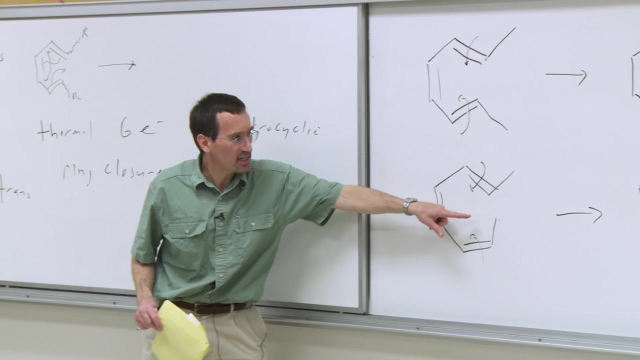 because, like, if you look at the chair confirmation, like one would be going down and one would be kind of going up. You know the easiest way, of course, when chair is sort of more the archetype for SP3, the easiest way to see it is: 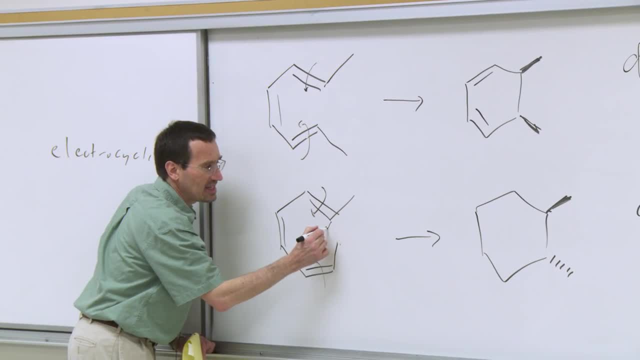 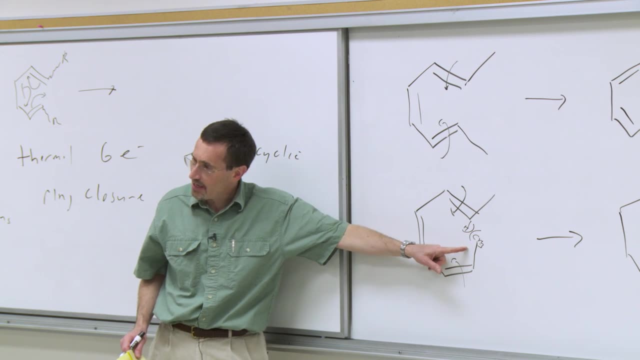 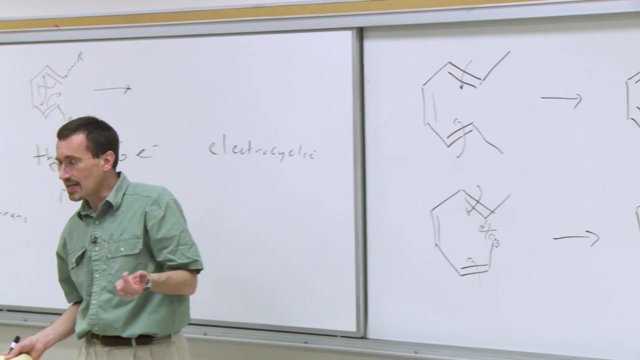 to configure like this: So Yeah, we've got this hydrogen banging into the methyl, So there's more steric hindrance in forming this cyclic, basically the pre-transition state, the ground state. So it is simply that that methyl brought in here is banging into the hydrogen here. 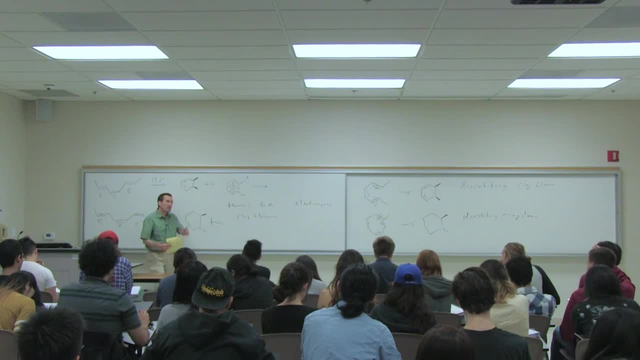 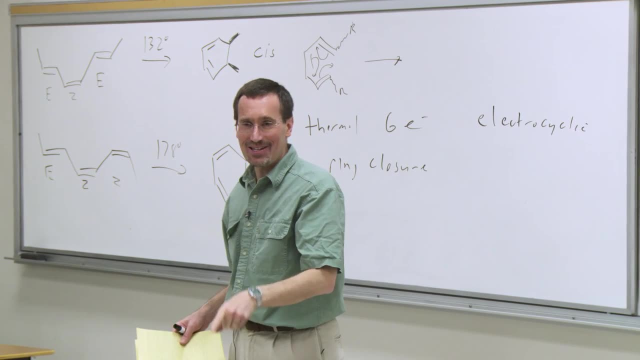 So that's why I said: don't worry that much about the differences in temperature. Is there a reason? it's disreputory as opposed to kind? Ah, and that's what we're going to get to, And that's the Nobel Prize. question is why. 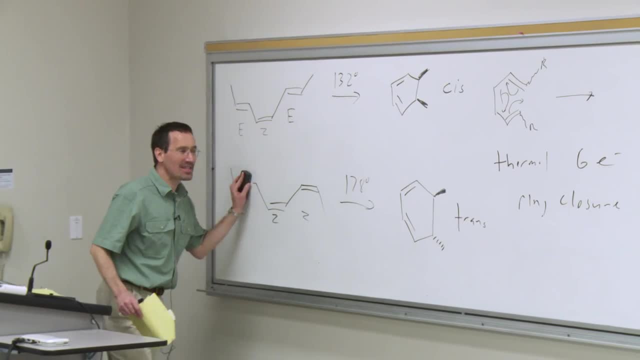 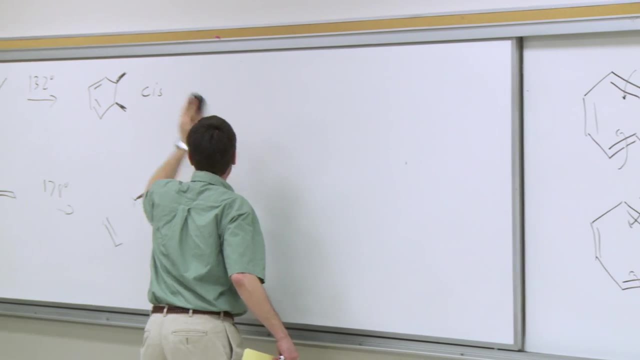 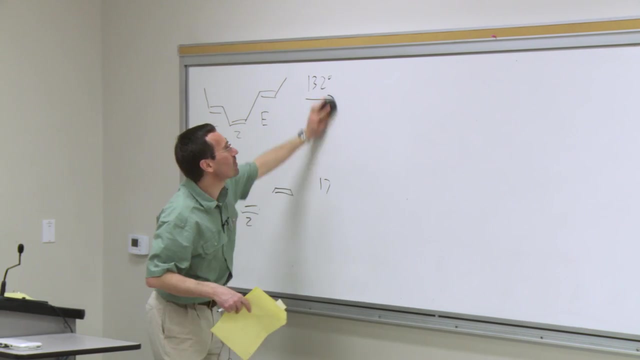 And I want to build to that. Okay, So we're going to see the extent of observations that led Woodward and Hoffman to formulate their understanding, based on molecular orbitals, which we developed last time and which I have suggestively put on the sideboard. 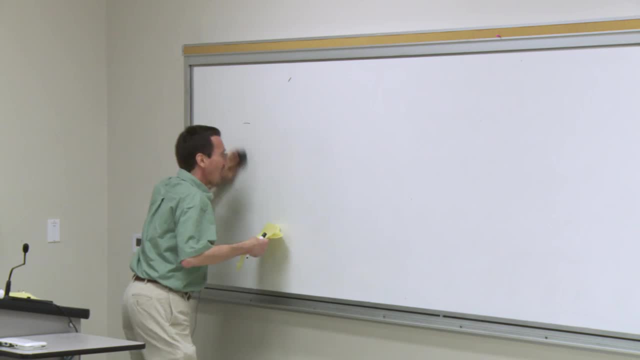 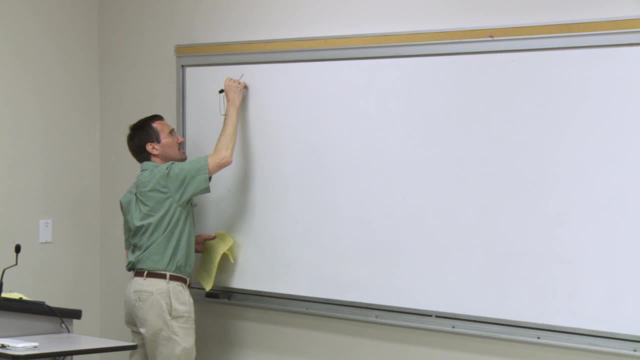 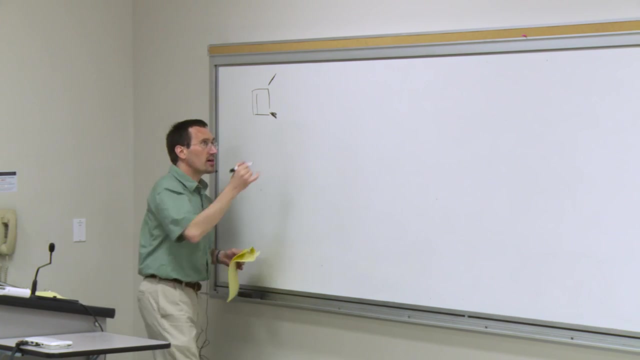 Some drawings that we had in your notes last time. All right, So I don't have an exact analogous system to show you, but remember I said all these reactions can go, be thought of in forward and reverse. So I'm going to give us a cyclobutene system. 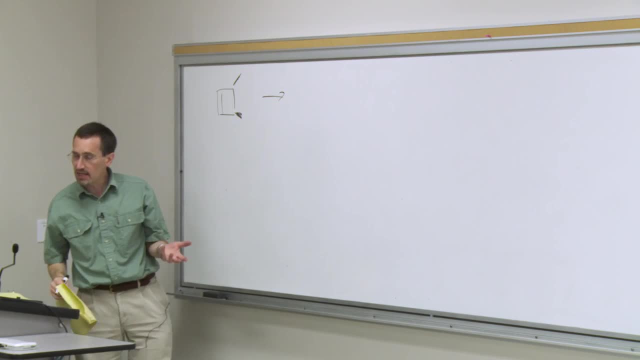 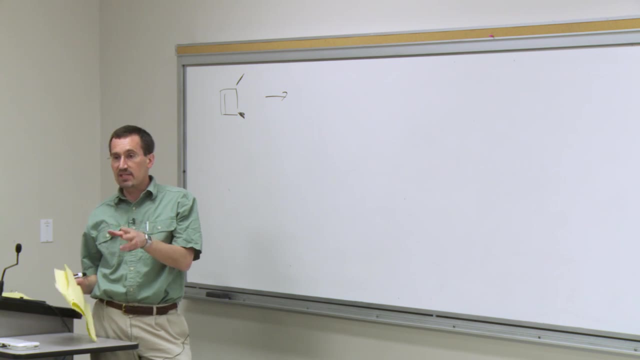 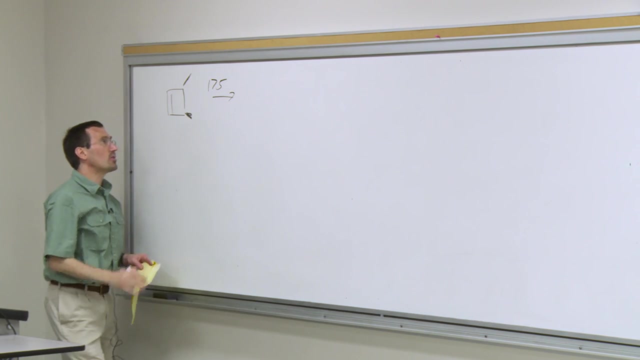 Now cyclobutene is strained. Cyclobutane itself has about 27 kilocalories per mole of ring strain. That's about, About enough to offset the loss of energy in forming pi systems. So when you heat cyclobutene with two cis-methyls on it, 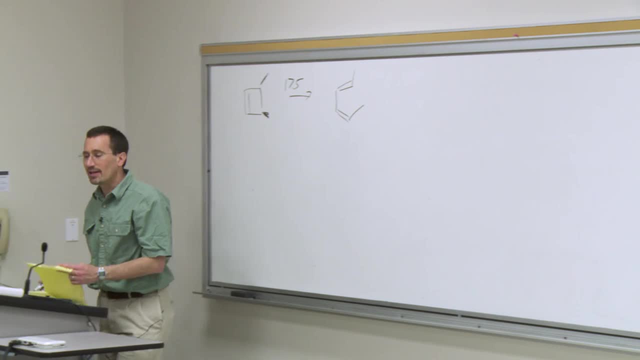 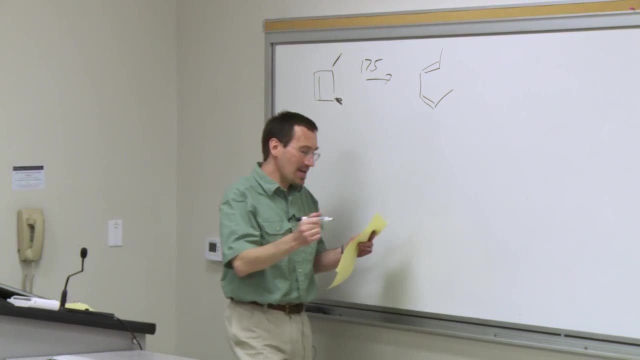 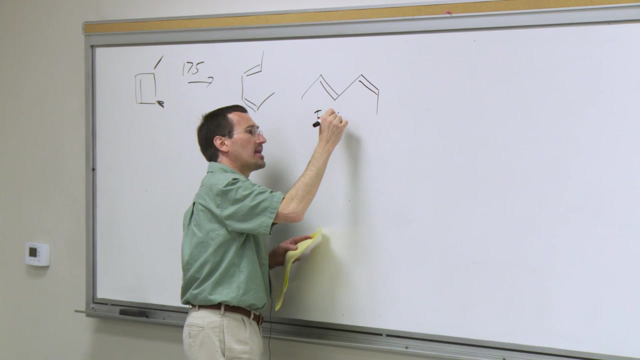 you get a diene and the diene, so technically it's a 2,4-hexadiene. The 2,4-hexadiene has one E and one Z double bond, So it's a double bond. It's a double bond in it. 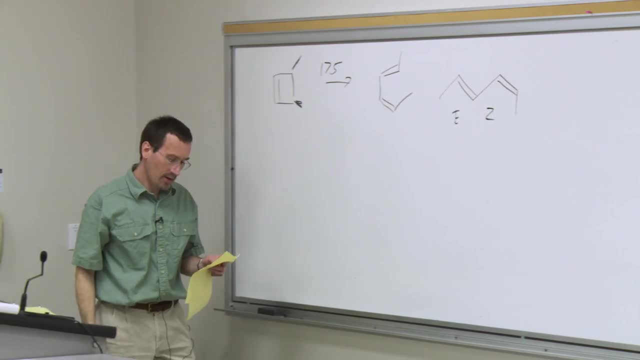 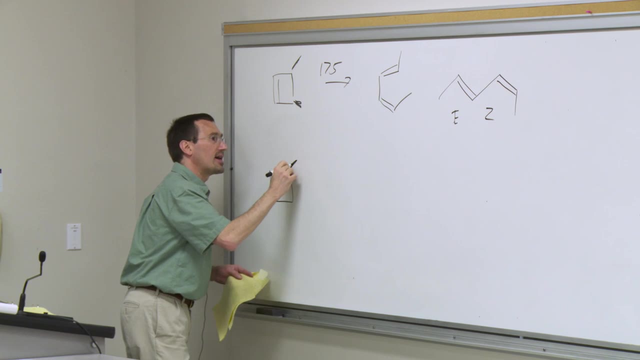 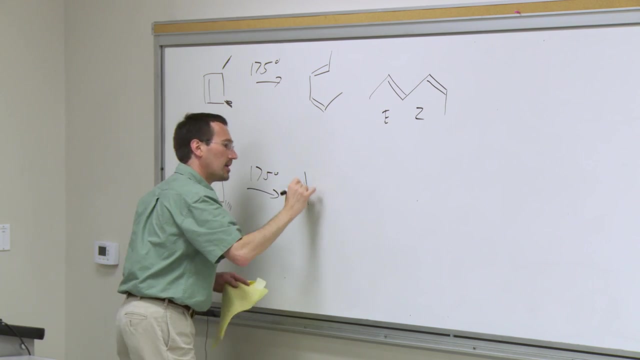 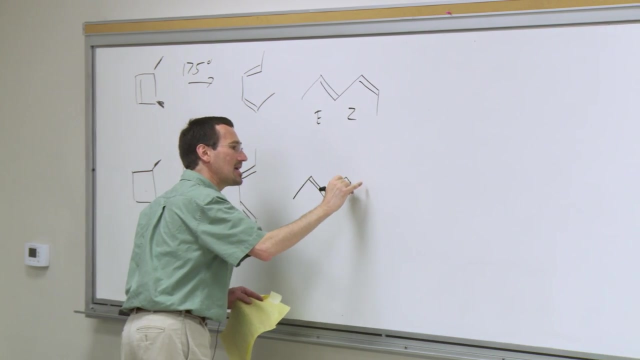 I've just gone ahead and unwrapped it like so And, conversely, if we take the other stereoisomer and heat it at 175 degrees, now we get the alkene, the diene, that is the EE stereoisomer. 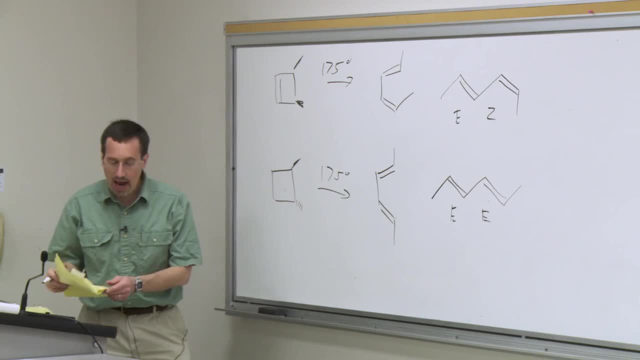 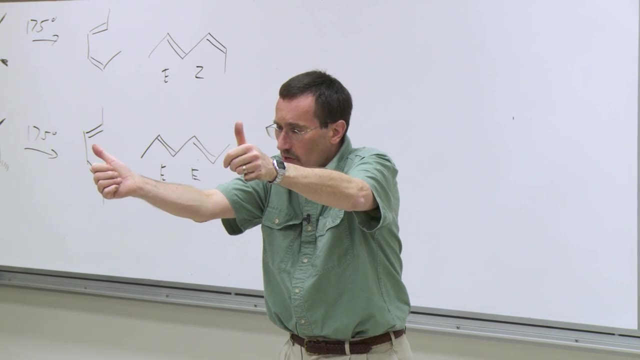 All right. So that's what we're going to do. All right, Now we can kind of do the hand thing again with the closed cyclobutene. So my thumbs are up. We'll start with the first one. My thumbs are up. 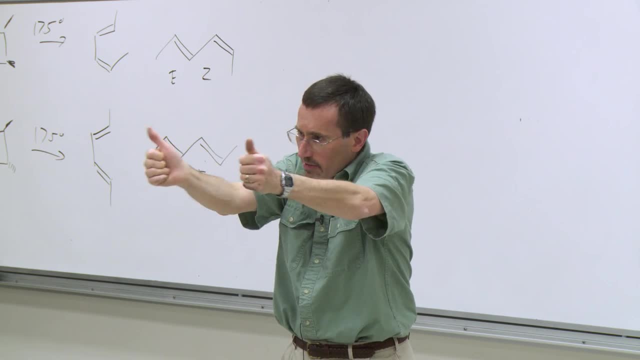 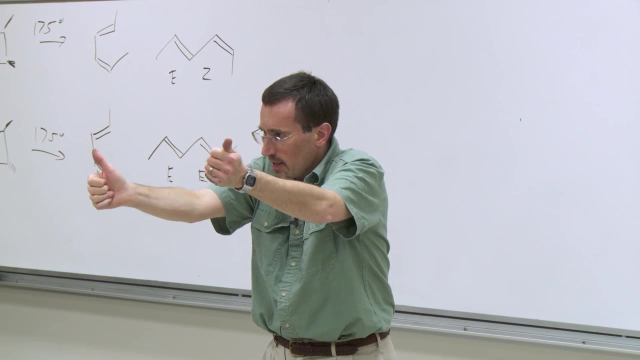 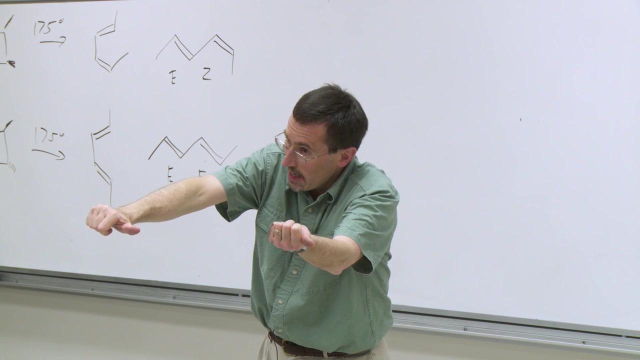 And as we break the sigma bond, here's the sigma bond in the cyclobutene that's going to get broken. As we break the sigma bond in the first example, I rotate one hand Counterclockwise And the other hand counterclockwise. 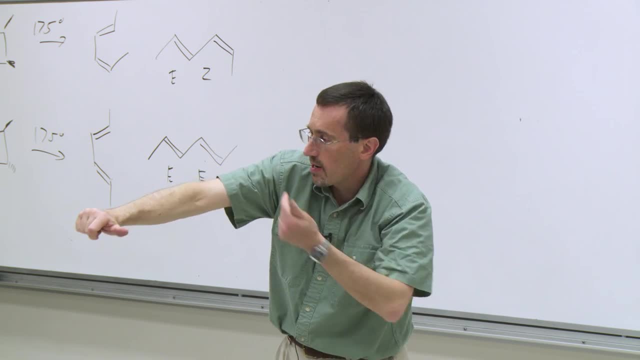 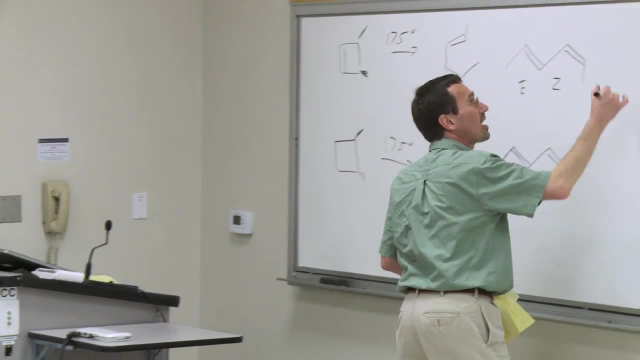 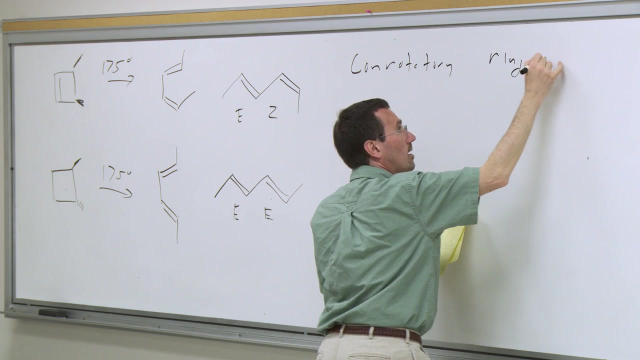 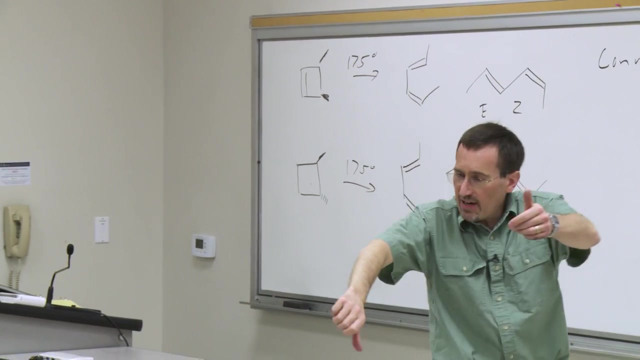 And that gives the E configuration over here and the Z configuration here. They rotate in the same way. So we call this conrotation or conrotatory ring opening. And you can convince yourself that if we have- and I think I'm going to really do some damage to my wrists at this point- 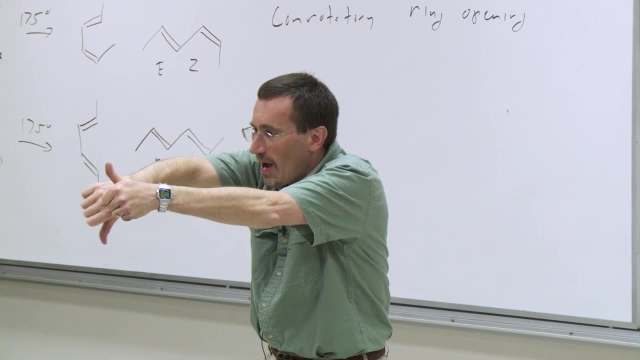 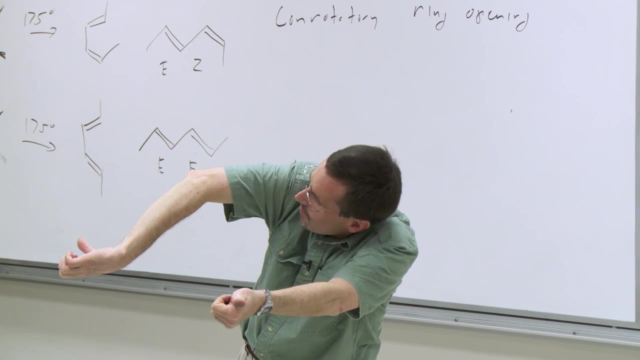 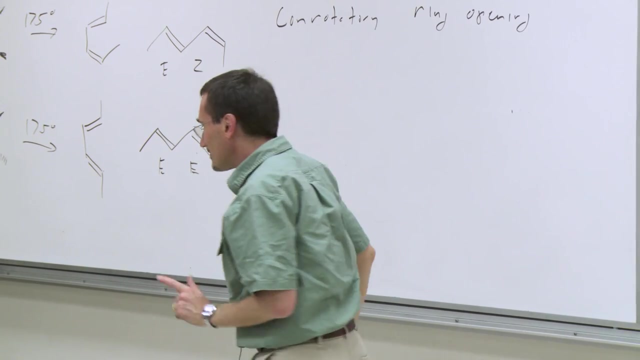 but you can convince yourself with your own wrists if you have the methyl groups trans to each other. And again we do conrotation. Now we get a trans double bond here and a trans double bond here. So here we see an example of a four electron process. 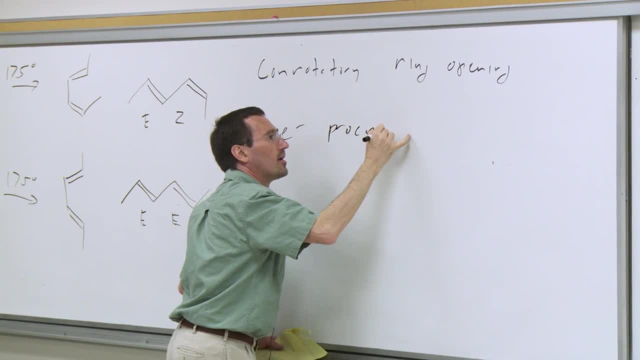 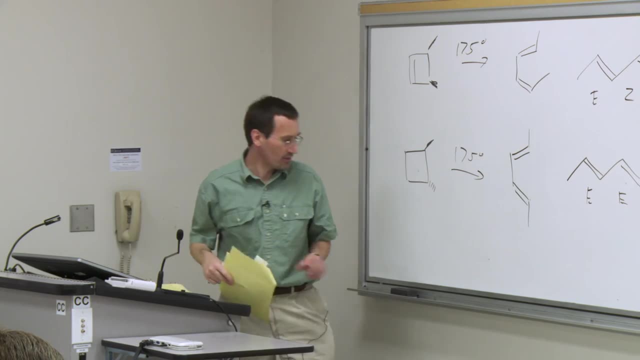 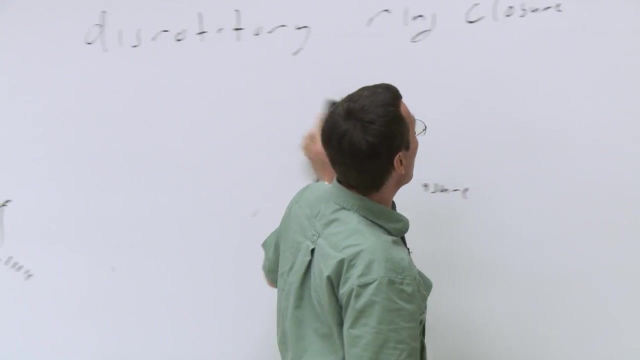 All right. So we have a four electron process That is conrotatory, And before we saw a six electron process That is disrotatory. Now this brings us to the whys on this And the easiest way to think about. 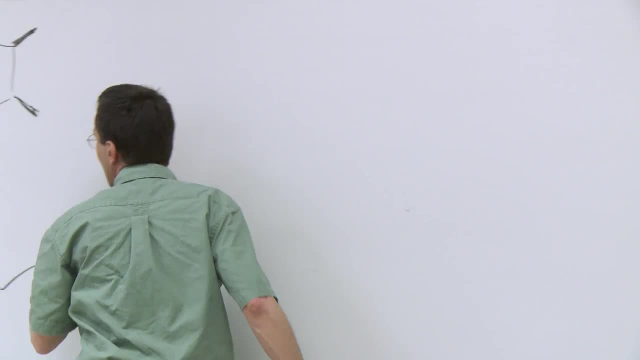 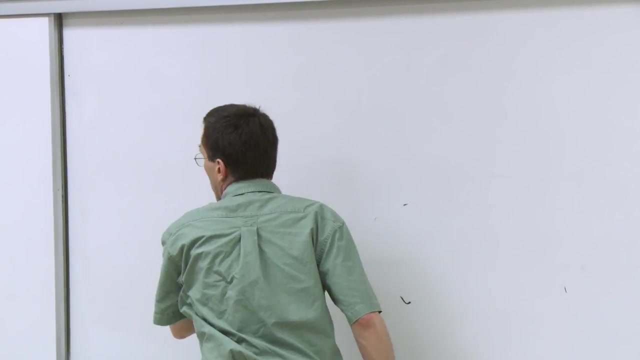 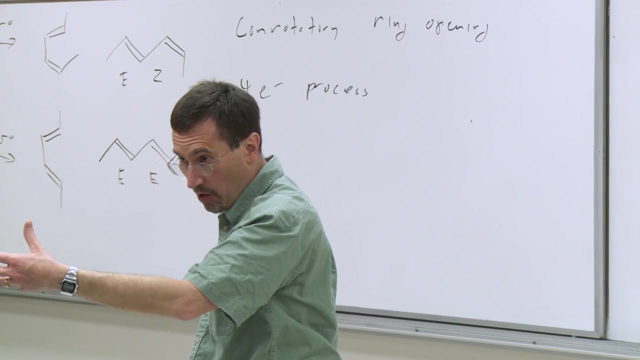 that's a little bit of a simplification, but the easiest way to think about it is that the pi electrons in the reactant are getting transformed to the sigma bond And the sigma electrons in the product in the case of ring closure, or the sigma electrons. 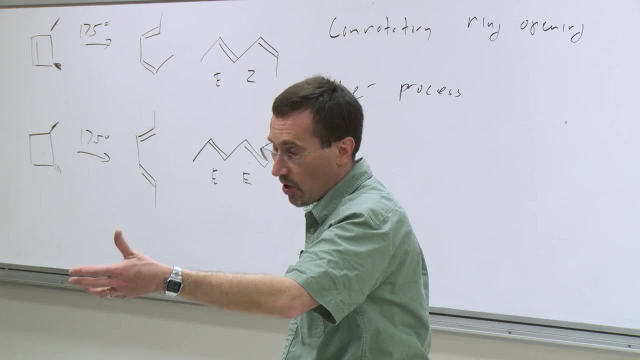 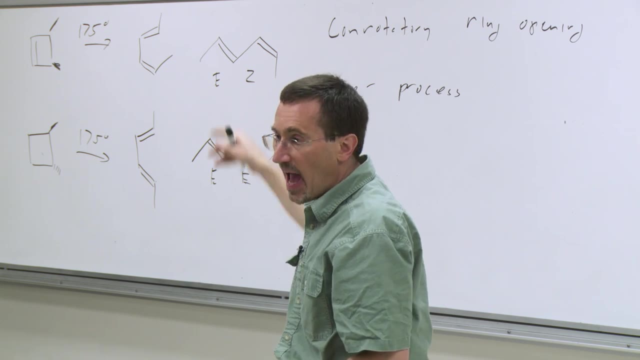 sigma orbitals, I should say in the product, are getting transformed into the pi orbitals of the reactant in the case of opening, And it doesn't matter whether you start one way or you start the other. You can think about it in the same way. 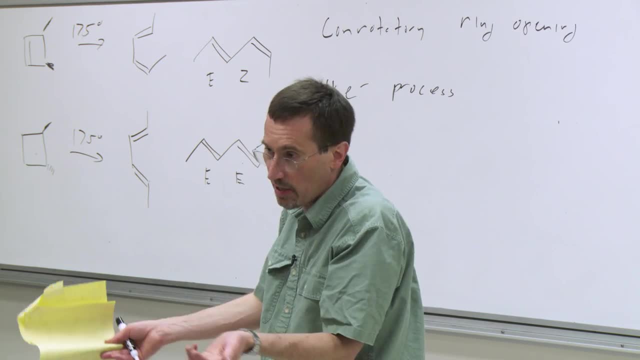 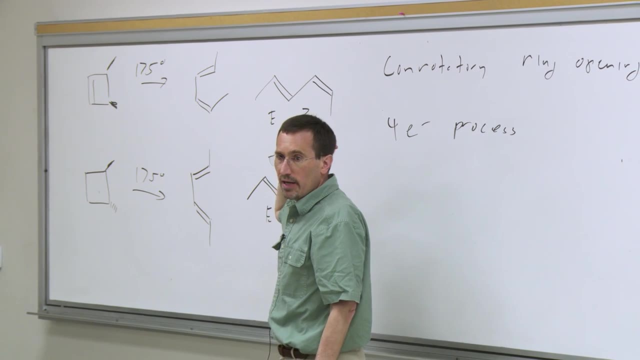 Whether you start with the diene and get the single bond or you start with the single bond, you get the diene. In other words, I can think about the electrocyclic ring closure in a forward sense. I can think about the electrocyclic ring opening here. 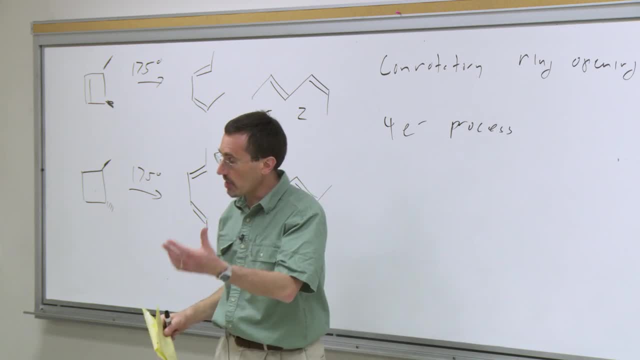 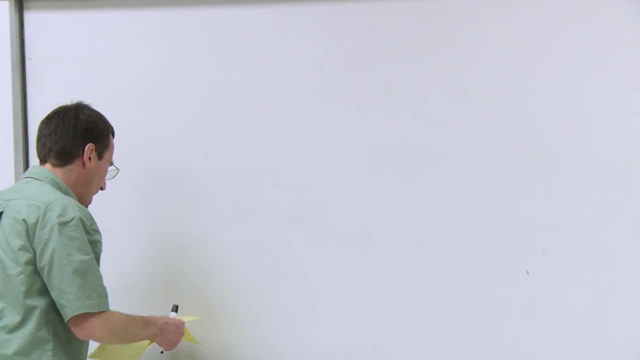 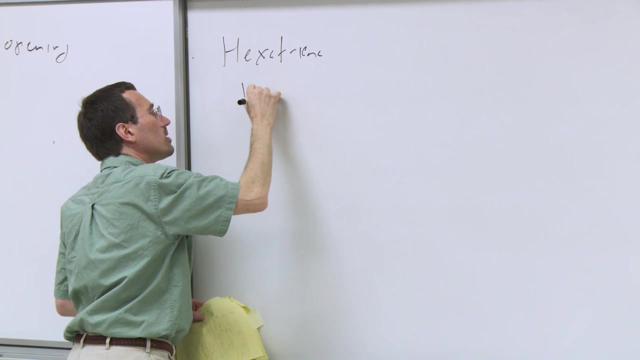 in the reverse sense and think about starting with the diene, and it's the same skill set. So let's start with the ring closing And I want to come to the hexatriene homo. So you can think of the hexatriene homo. 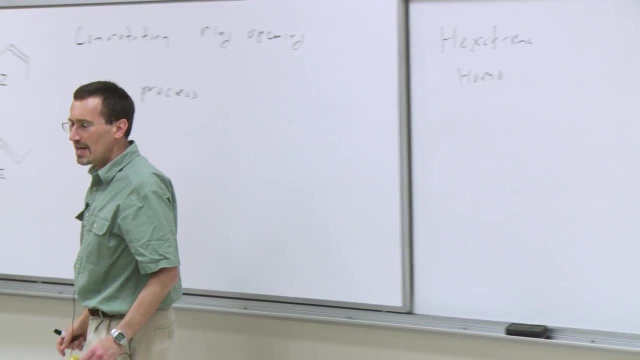 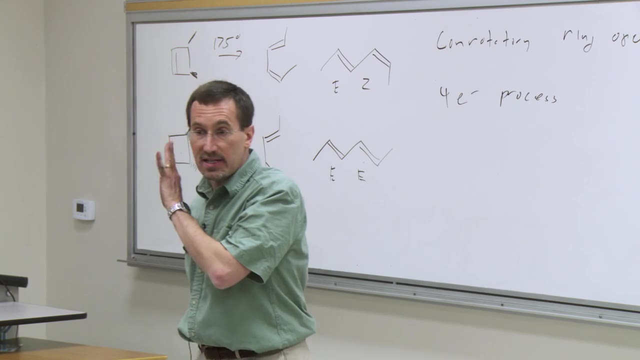 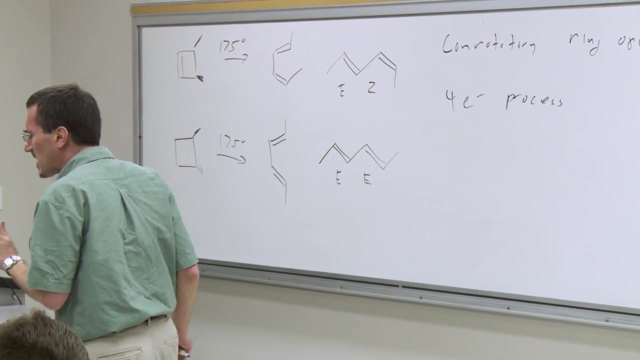 as a single bond. Think of the hexatriene homo as being transformed into the new sigma bond. Now remember, we said that the hexatriene had six pi type molecular orbitals, six psi orbitals: psi one, two, three, four, five, six. 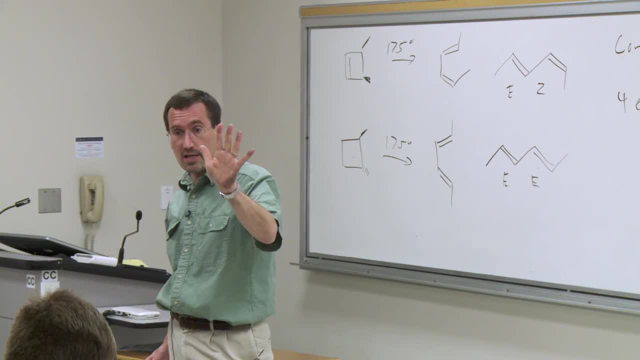 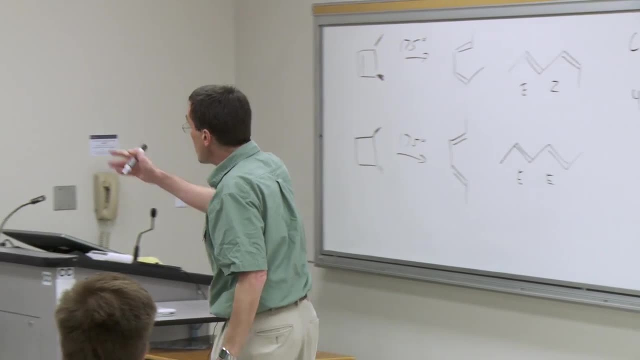 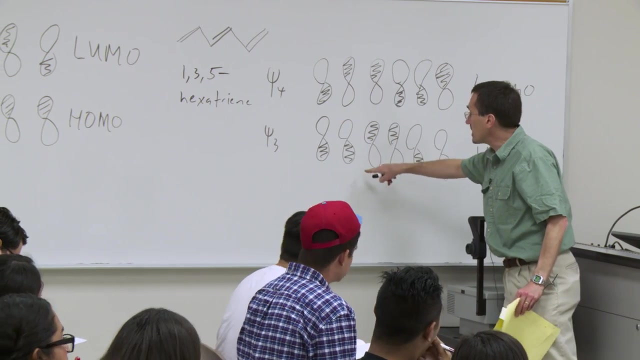 Psi three: we had six pi electrons, So psi three was the homo and psi four was the LUMO, And I've written them out. This is what we wrote. Psi four: remember we talked about the linear combination of p orbitals and the increasing number of nodes in the plane. Psi one had no nodes except for the node associated with the p orbitals. Psi two: we get one node, meaning these orbitals here on one side are on the same sign, These over here are opposite. Psi three: we get two nodes. 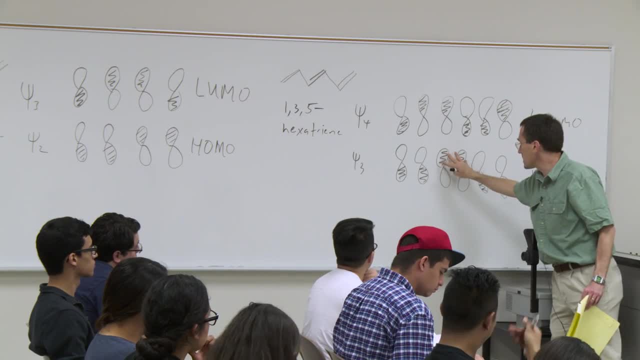 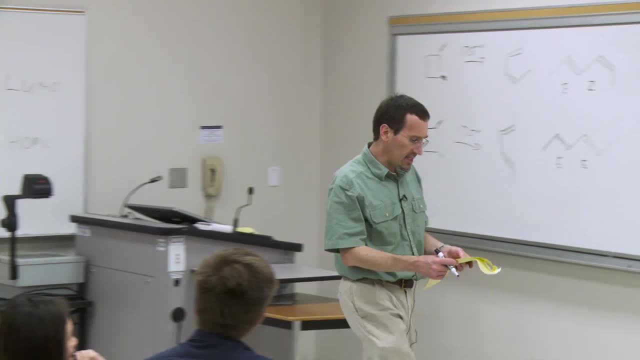 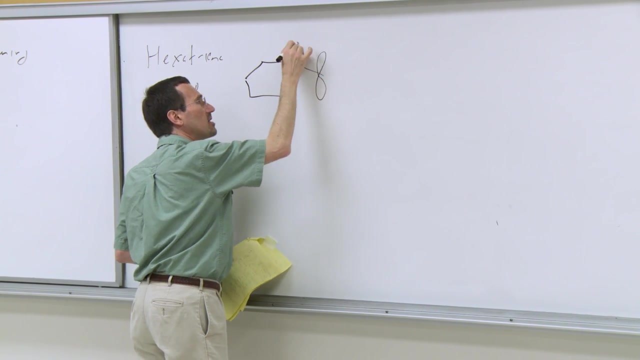 So these two are the same sign. Then we get these two the same sign, and these two the same sign. We get a nodal plane here and here I'm just going to draw psi three, the hexatriene homo, in perspective, in a ring, as best as I can. 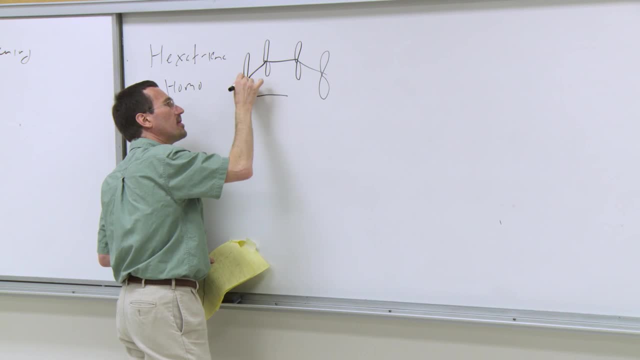 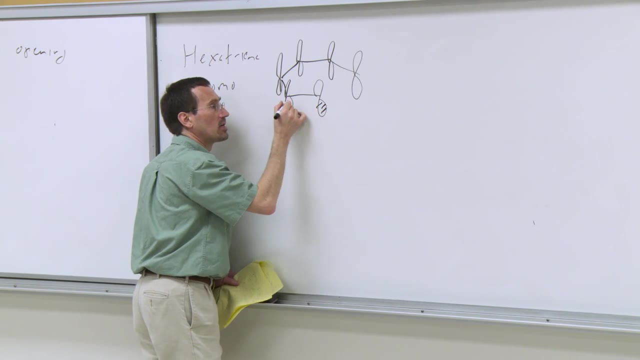 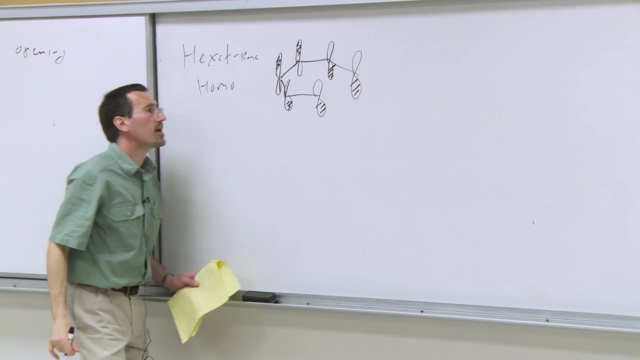 So I've sort of drawn this ring obliquely and I'm now taking my orbitals, my six orbitals, and I'm now going to shade those orbitals to show the shading, And in transforming so I've sort of made a big ring here. 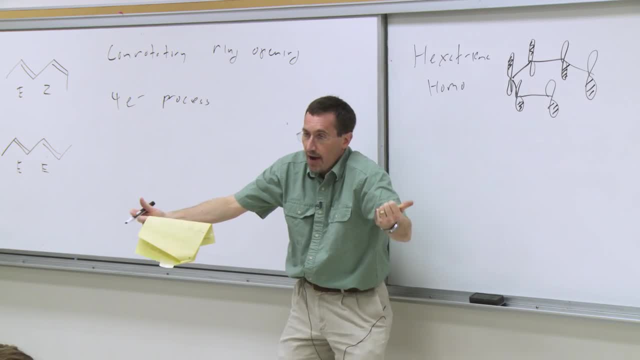 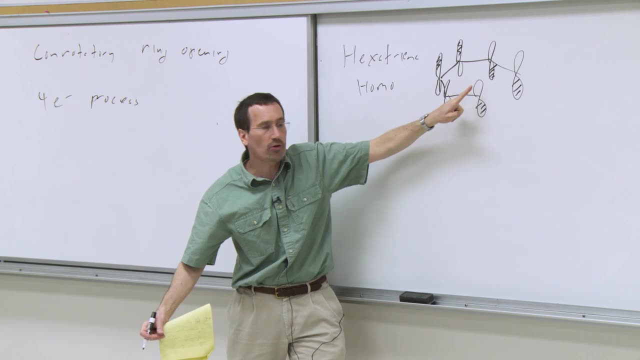 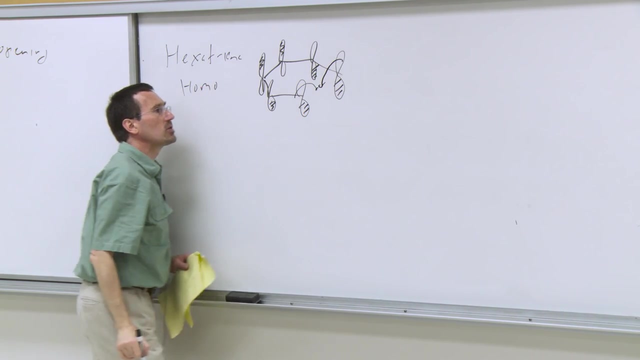 with my orbitals coming up and down like this. Now, in transforming the pi orbital, the homo, into the sigma orbital, we need to create a positive overlap. In other words, we've got to rotate this in and rotate that in, so positive overlaps with positive. 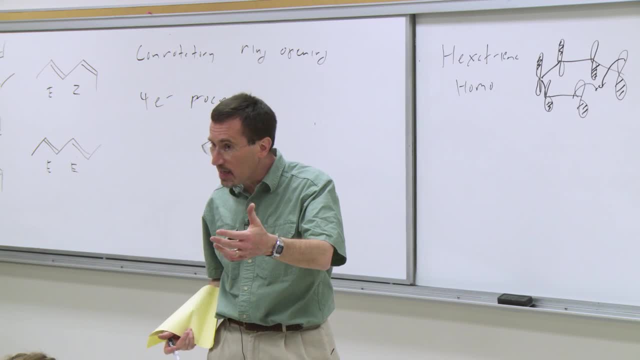 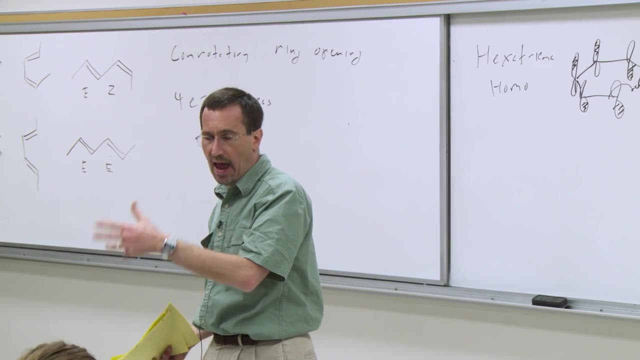 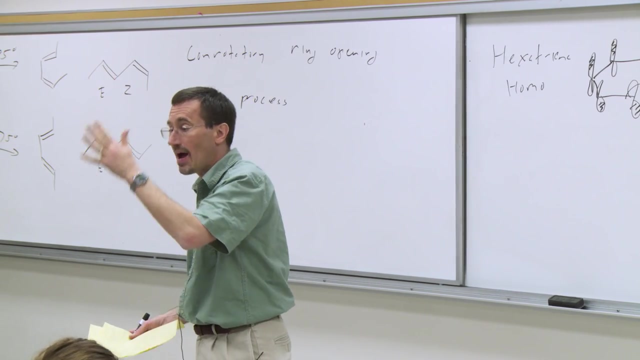 Remember: white overlapping with white is a bonding interest. It's a bonding interaction. Black overlapping with black is a bonding interaction. White overlapping with black is an anti-bonding interaction or a non-bonding, where you have no net electron density between them. 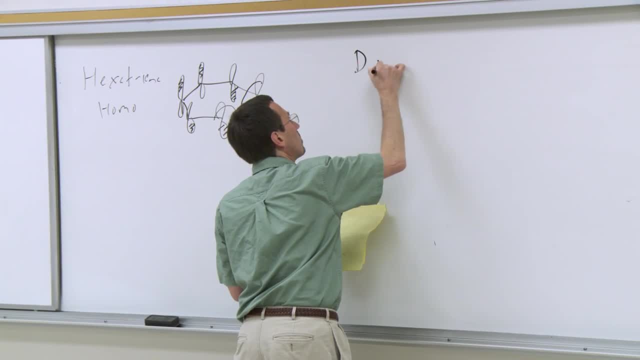 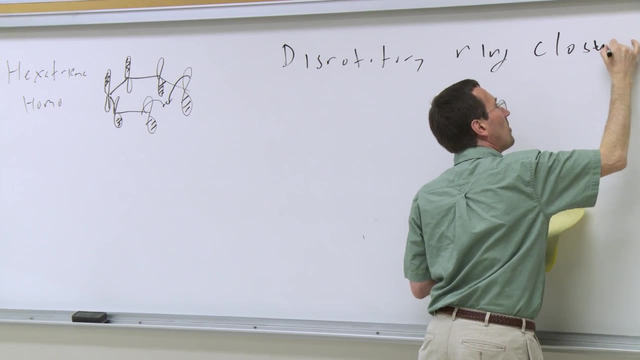 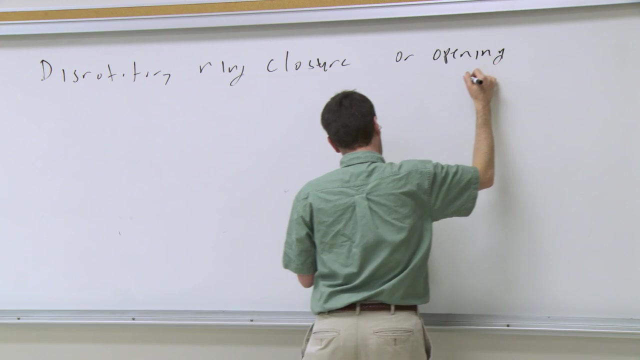 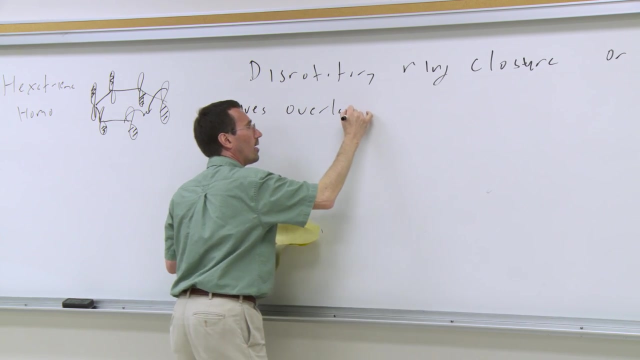 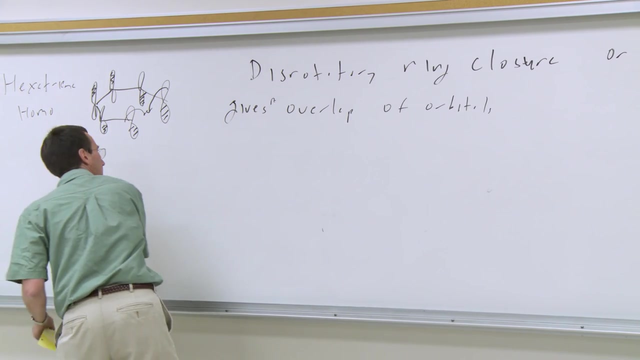 And so basically what we see is that disrotatory ring- remember, we can think about it in forward or reverse. So disrotatory ring, closure or opening- gives a net overlap. We'll say net, or I'll call it a favorable overlap of orbitals. 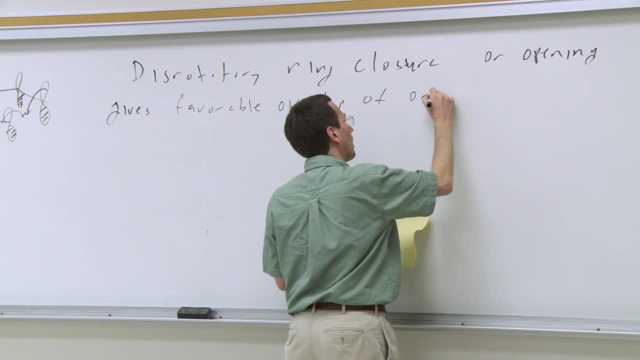 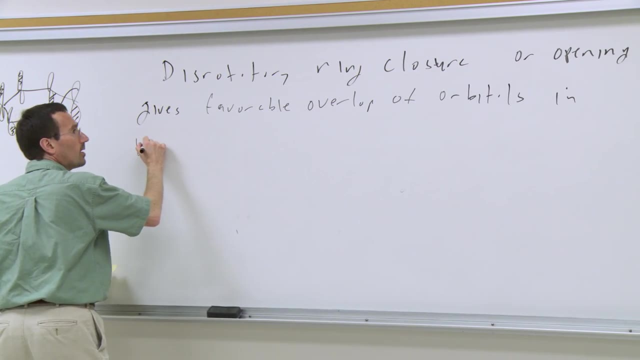 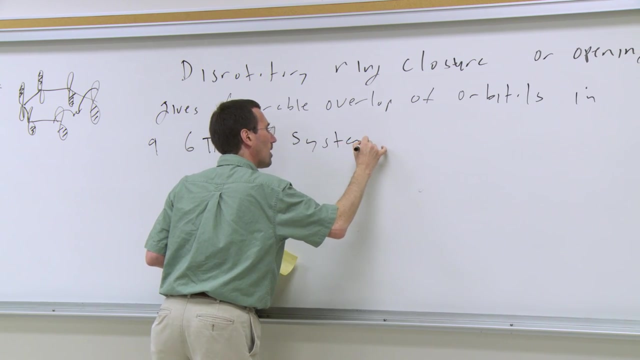 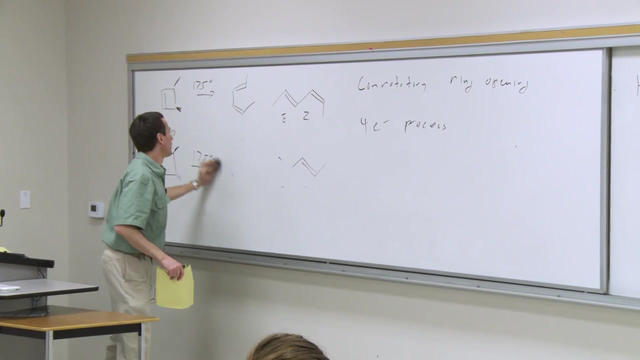 Now here you can see the in the 6 pi electron system. So we've got this in the 6 pi electron system. OK, All right, OK, All right, OK, OK, OK, All right, OK, OK. 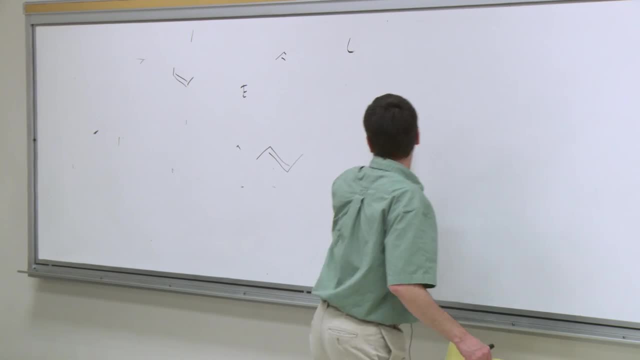 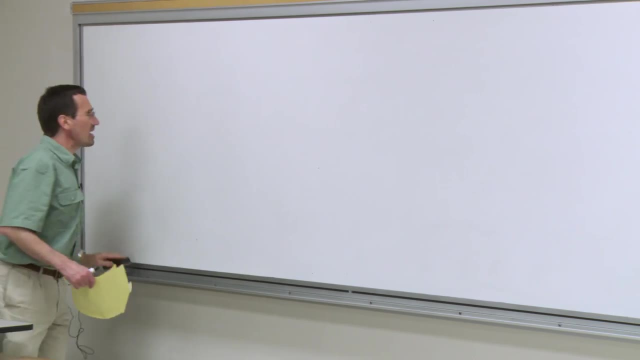 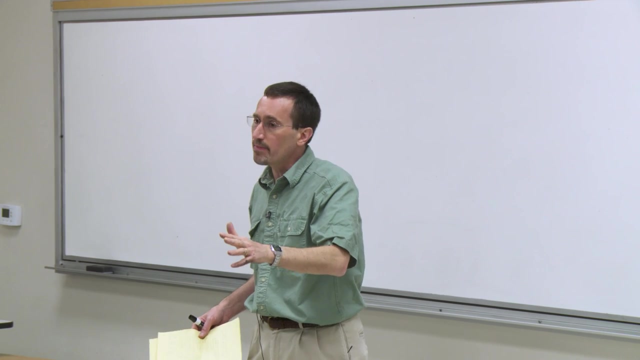 OK. OK, We can do the same thing with the butadiene system And remember we can think in terms of closing or opening being the same. It's much easier to think in terms of closing because we've already worked out the pi orbitals. 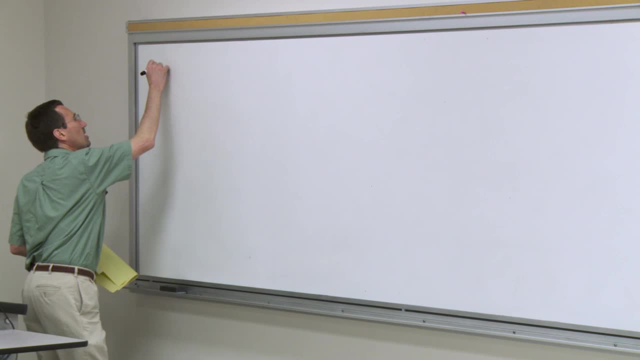 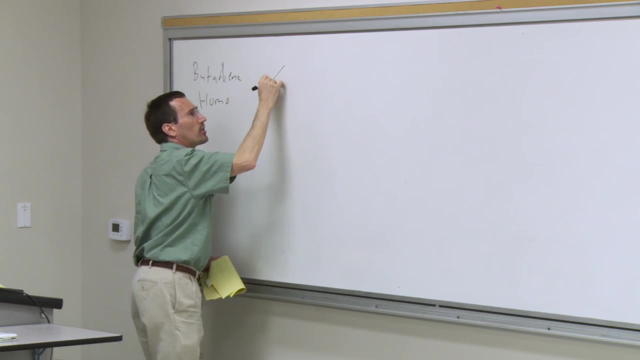 So let's start with the butadiene HOMO, and then again, I'm going to write it as best as I can in perspective. So that's psi 2 that I've sketched out for butadiene there. We already worked that out last class. 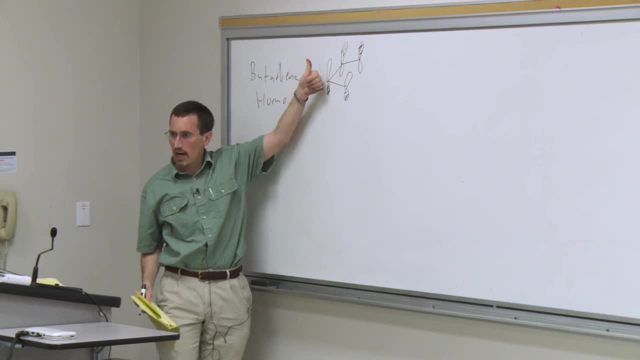 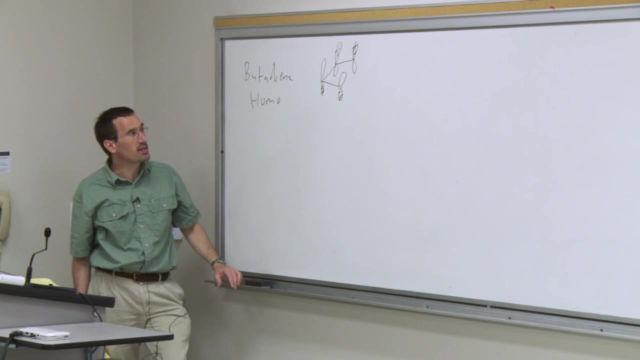 So there's psi 2. We have 2 or 3. We have 2 orbitals in one sign and then 2 in the reverse sign of our p, orbitals that we're combining in a linear fashion to make the pi type orbital. 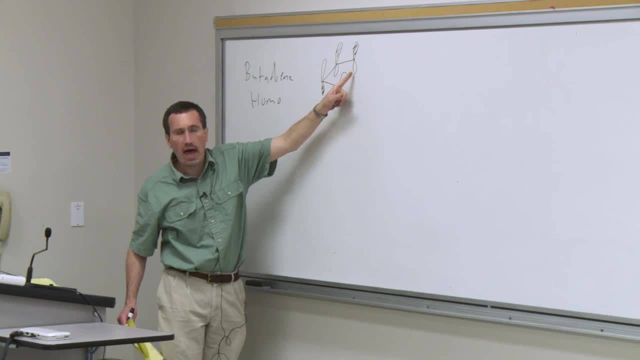 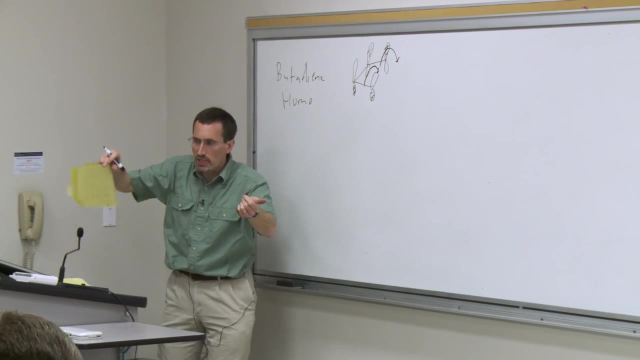 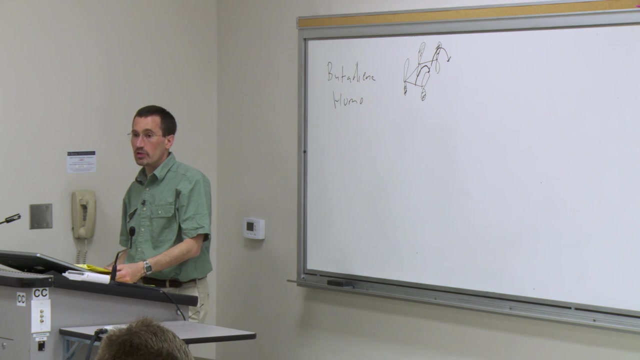 And now we want to overlap white with white or black with black. And now, if I show my rotation, they have to rotate in the same way in order to get that white with white overlap. In other words, we have to have a conrotatory ring. closure or opening. 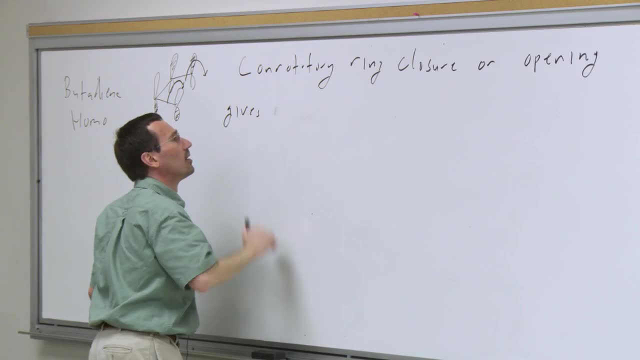 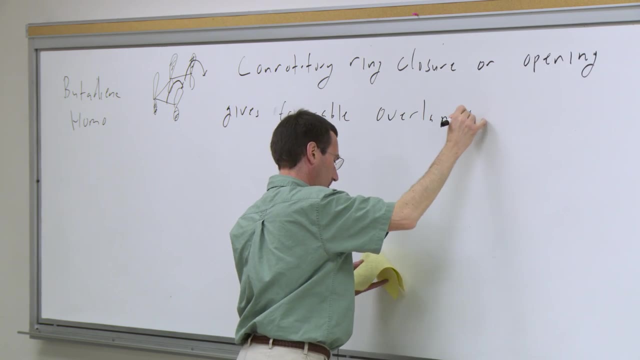 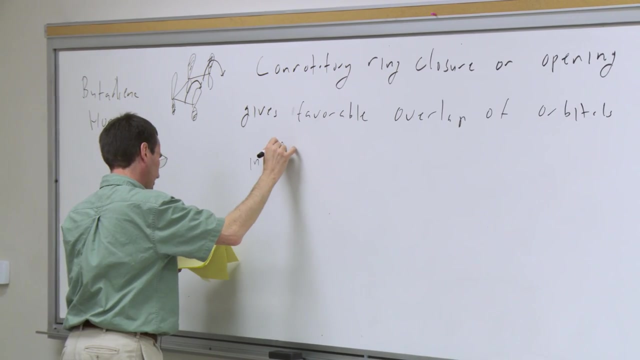 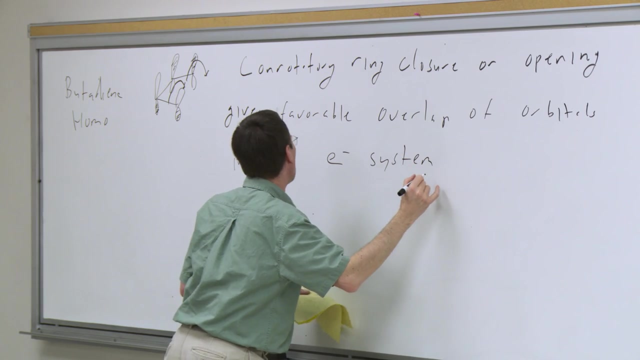 I'll say favorable, And then we can show you a little bit of a closer look. Now this is called a uniform pi electron system. I'll show you a little bit of a closer look. You see the right side. You can see that. 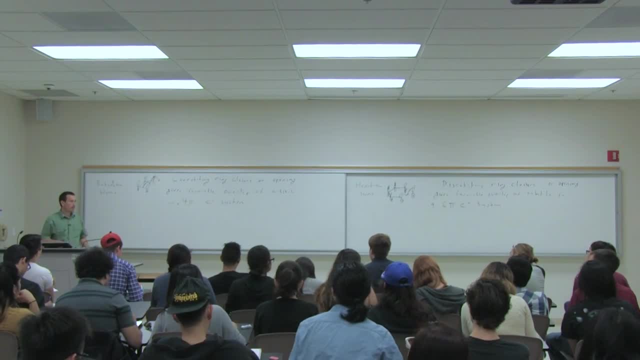 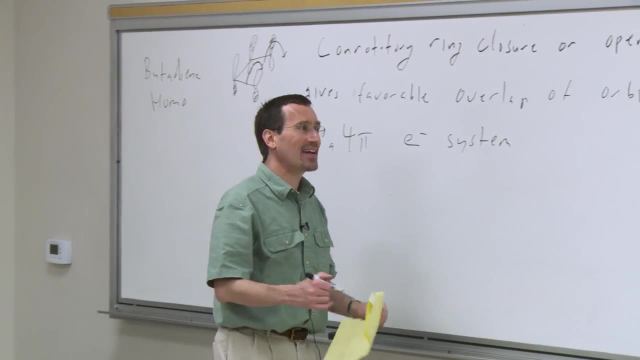 I don't want to go too far. You can see that I don't want to. You can see that I don't want to. You can see that. Yeah, Yeah, Yeah, Yeah, Yeah. Well, all right, I will add that you are getting us to the next slide. 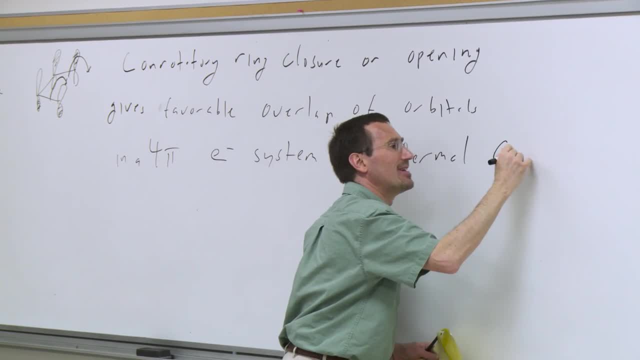 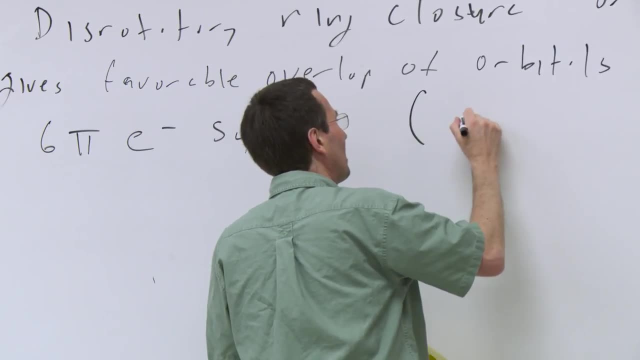 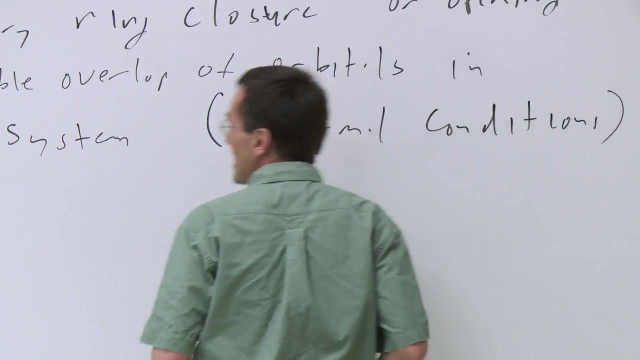 This is what we call thermal conditions. we're going to come to photochemical in just a second, and then we'll sum it up with a little table at the end. In other words, in a heat driven reaction rather than in a light driven reaction. 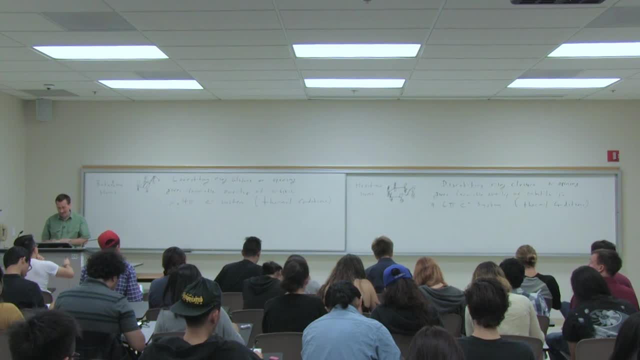 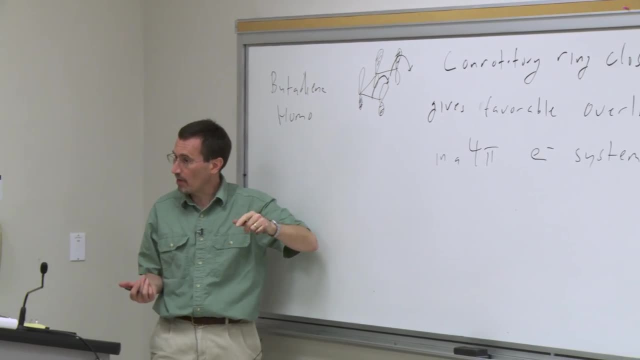 Everything is reversed in a light driven reaction. Yeah, question. Just to be certain, though. both are being rotated clockwise right, And it doesn't matter, they could go clockwise or counterclockwise. Remember, black with black is as good as white with white. 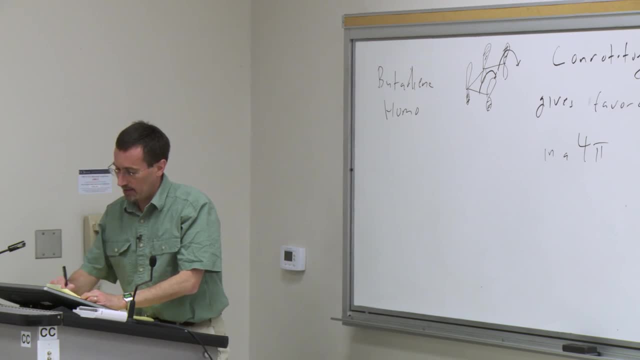 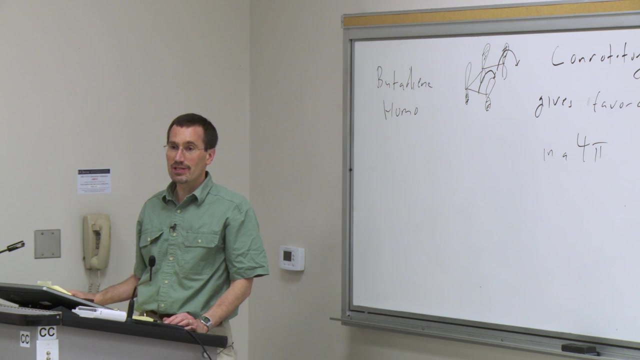 Black and white are arbitrary, it's only relative. But you don't want white with black, Exactly. That would be an unfavorable. That would be an unfavorable and anti-bonding interaction Questions, Other questions. These are good ones. This is the conceptual stuff here right now. 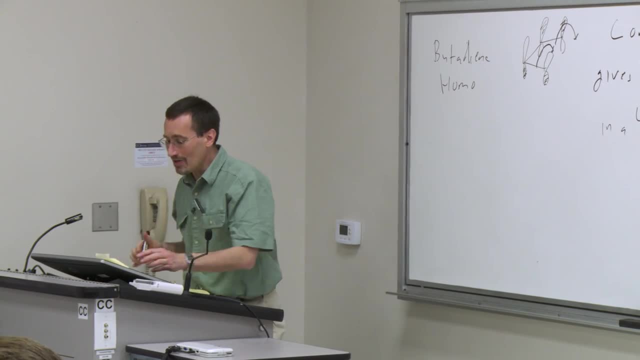 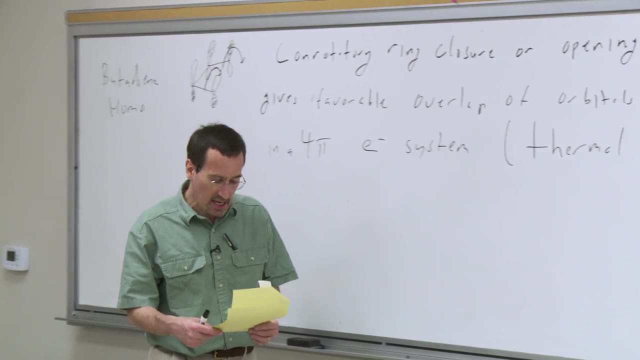 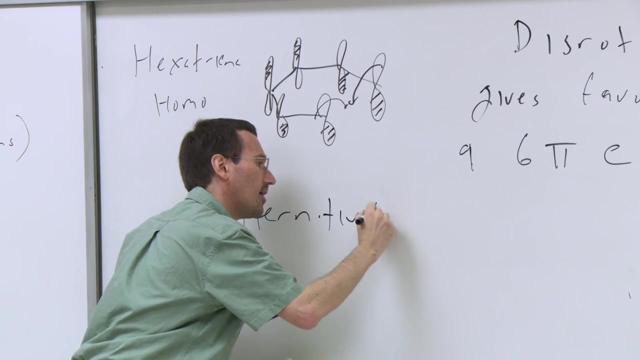 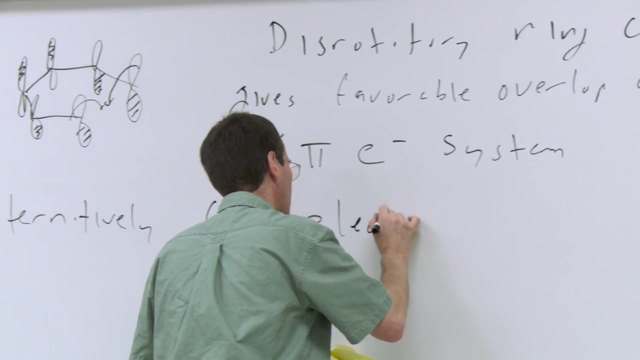 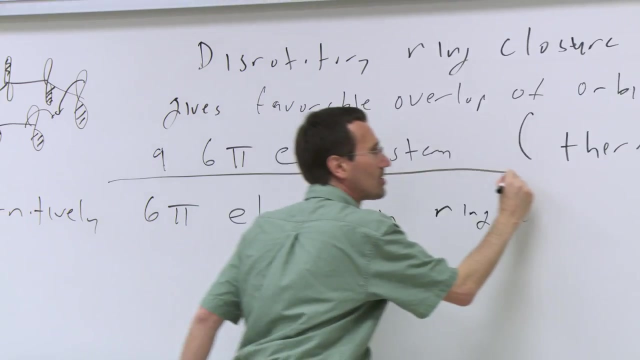 Thoughts. All right, there are two ways of thinking about this. Your textbook presents this as the primary way. The other way that you can think of it is alternatively. you've got six pi electrons in a ring, so I'll just draw a line here. 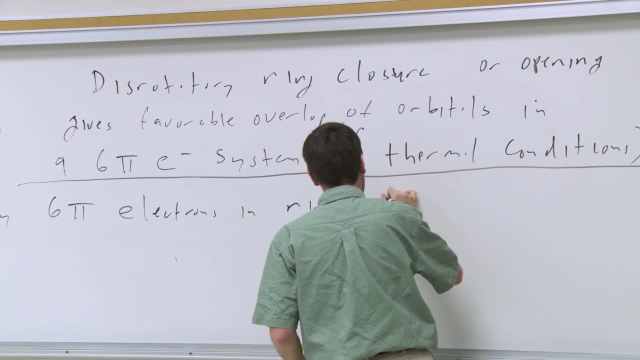 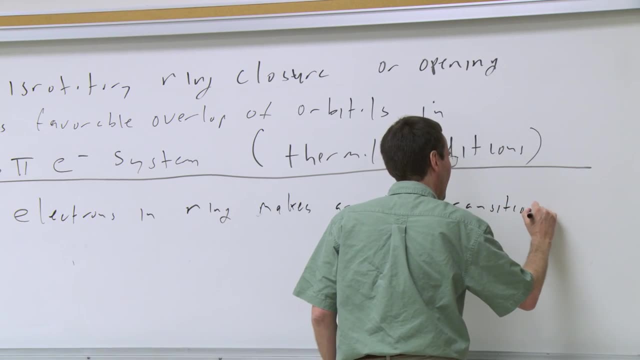 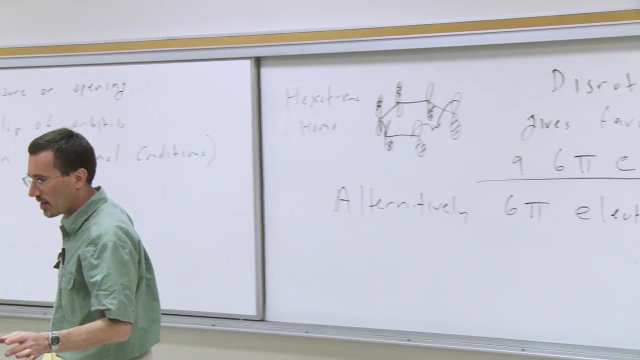 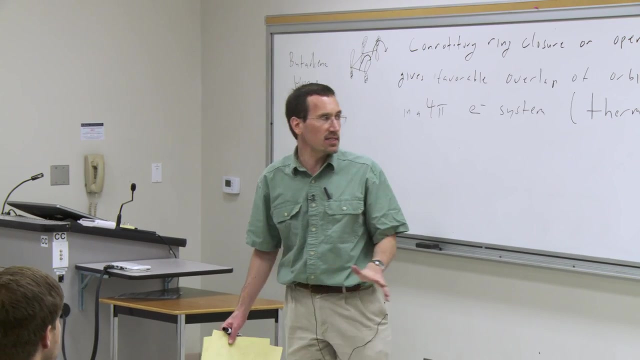 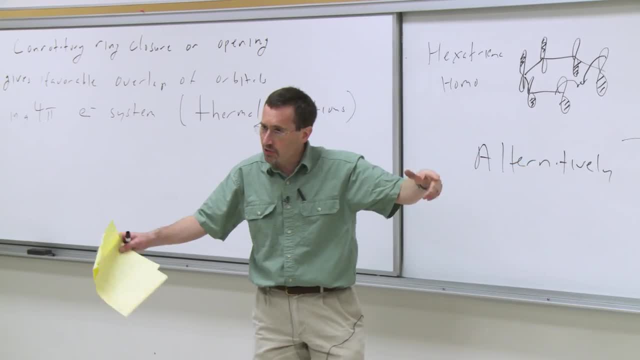 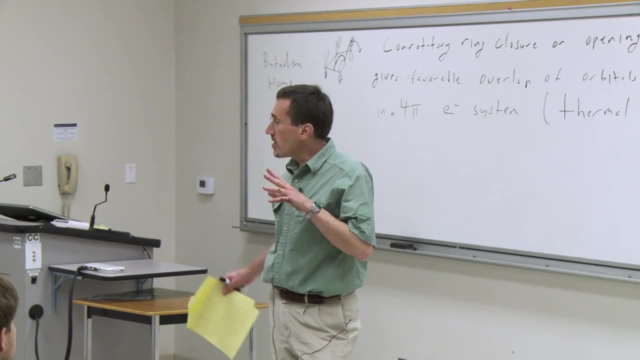 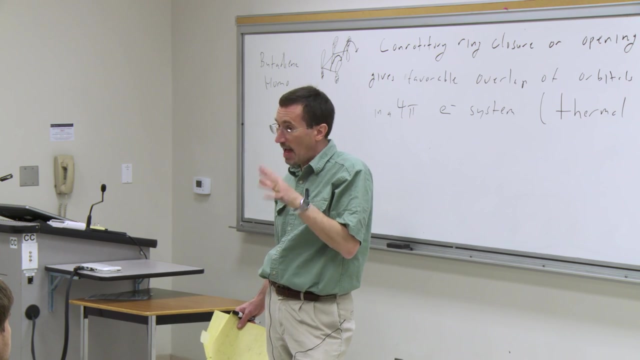 So one way to think about this is, as we go to the transition state and we bring those pi electrons together, we start to make an aromatic state. It's an aromatic transition state and therefore it is more favorable than it would be otherwise. We're having this reaction occur under relatively mild conditions. 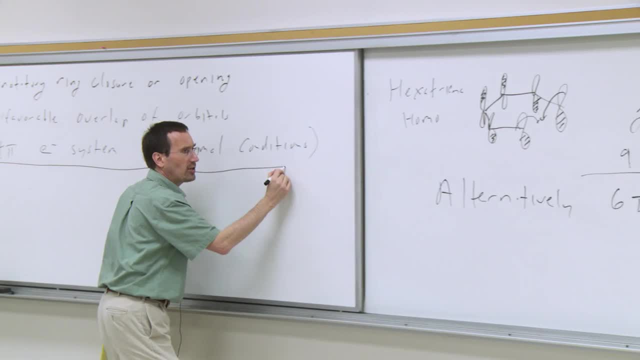 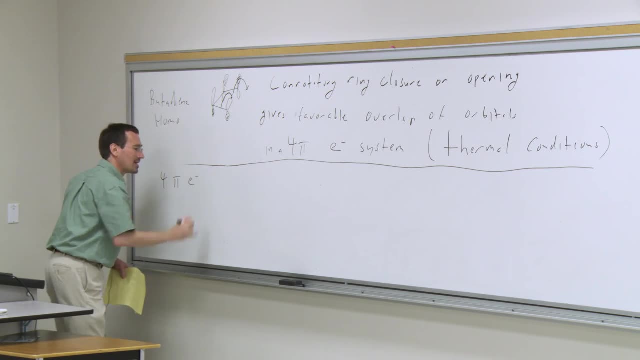 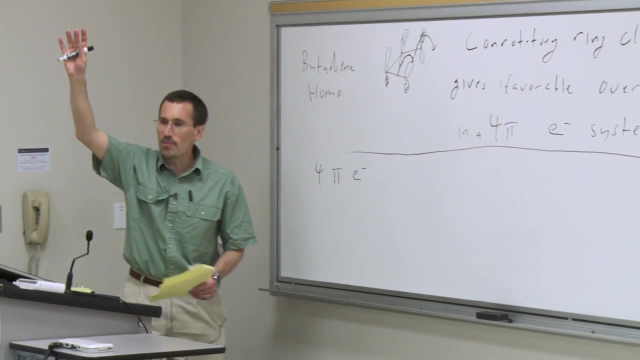 Now, by the same thinking: four electrons, four pi electrons, is disfavorable in a ring, but in a Mobius strip. Who knows what a Mobius strip is? Mobius strip is what Mobius strip is, where you take a piece of paper, you know. 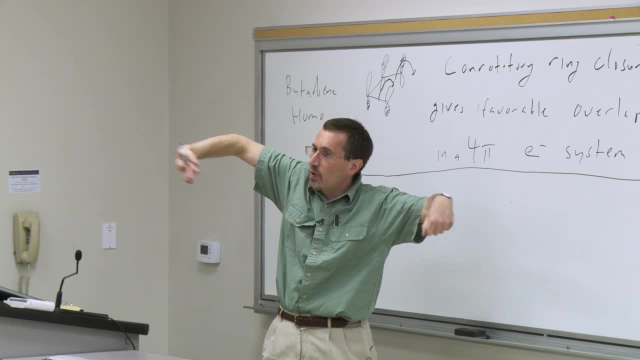 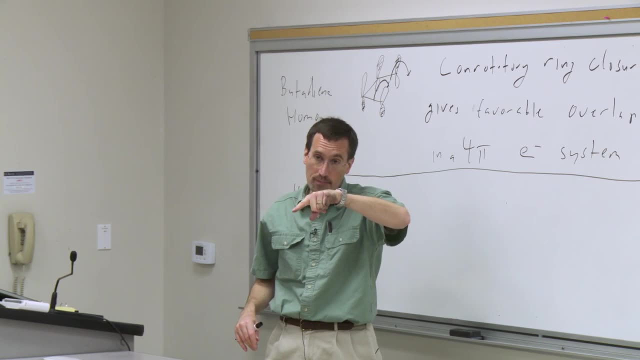 a long strip and you basically give one half twist and tape it on its end and it's got a half twist to it and now that's called a Mobius strip, And if you go ahead and you actually cut it open, it becomes a bigger ring, which is sort 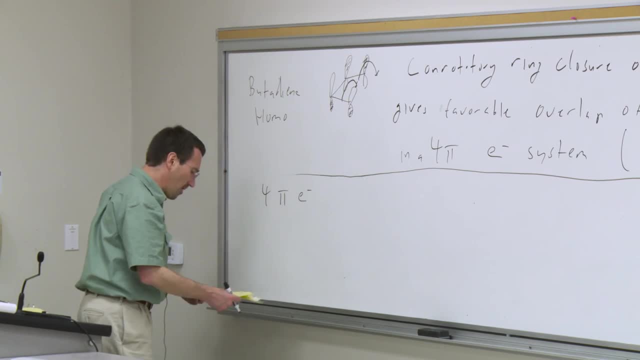 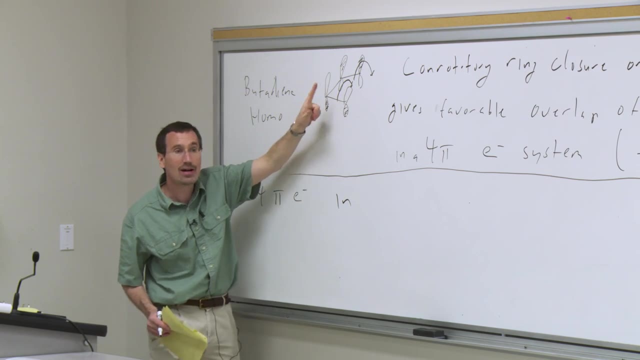 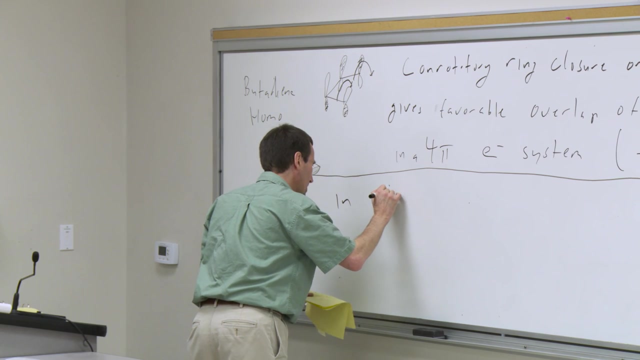 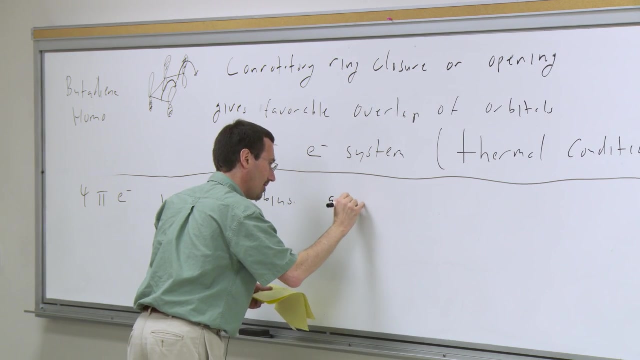 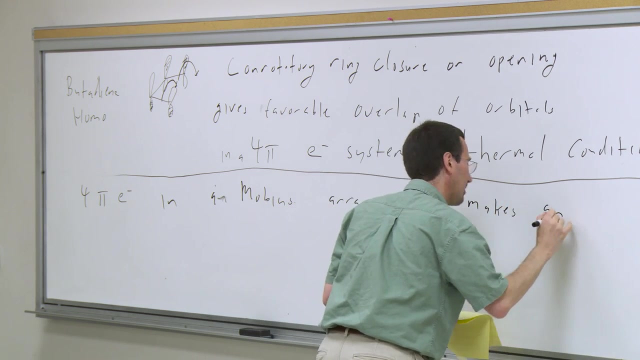 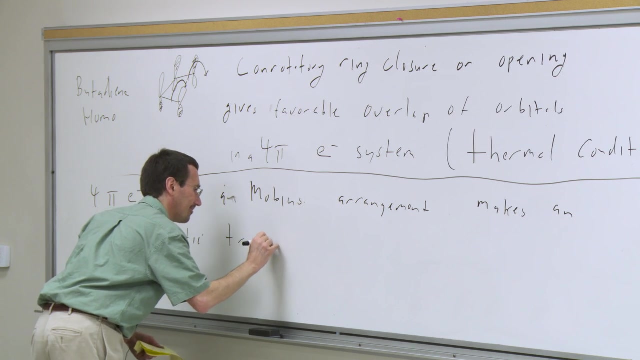 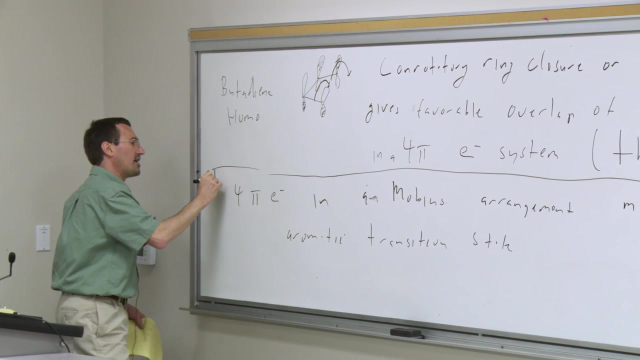 of an interesting topological thing, But anyway, four pi electrons in a Mobius rearrangement, which is what you get when you put that twist in here and you have a conrotatory process that makes for an aromatic transition state. And again, I'm going to write this as an alternative way. 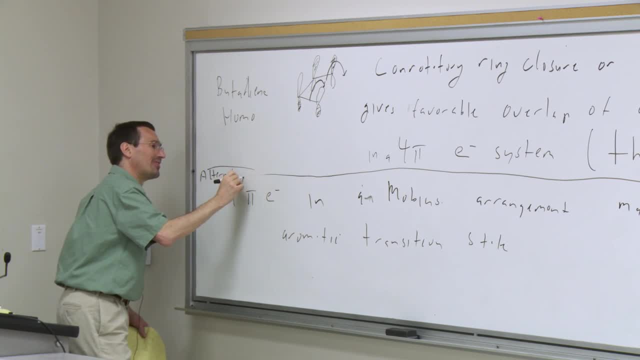 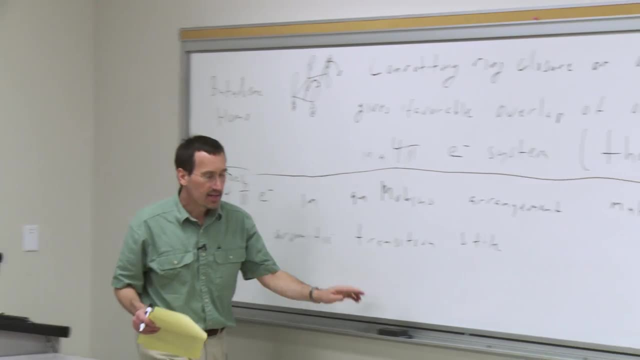 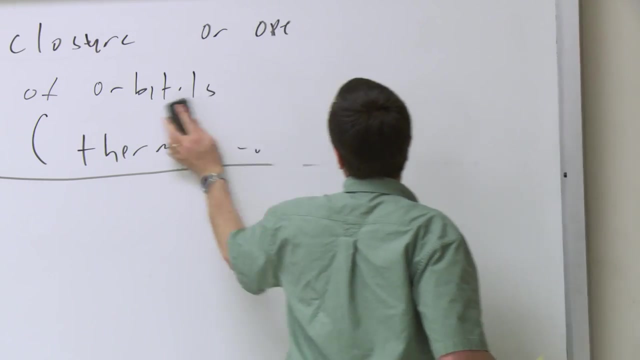 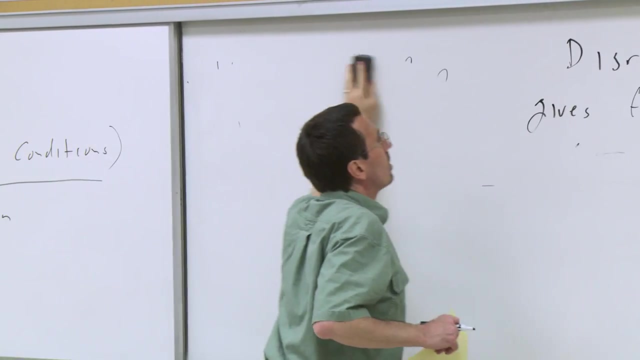 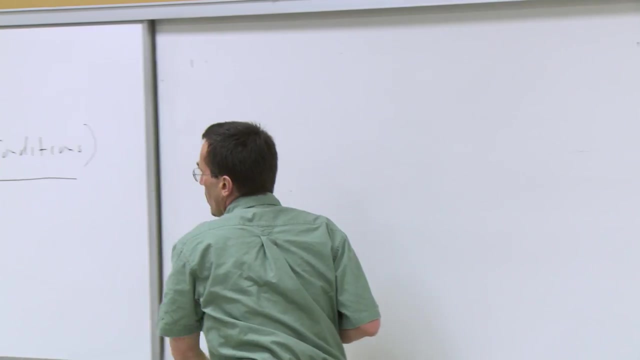 of saying the same thing, So I'll write alternatively, just to let you know that you're basically saying the same thing in a different way. So what is interesting, what is fascinating about all this is these are rules. These really come from the orbitals. 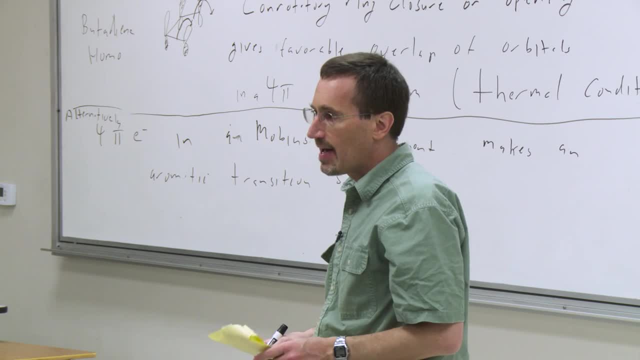 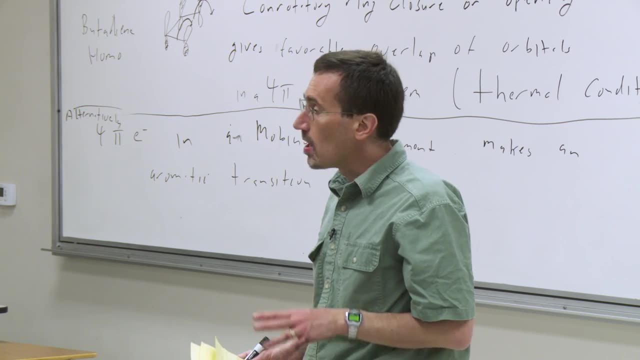 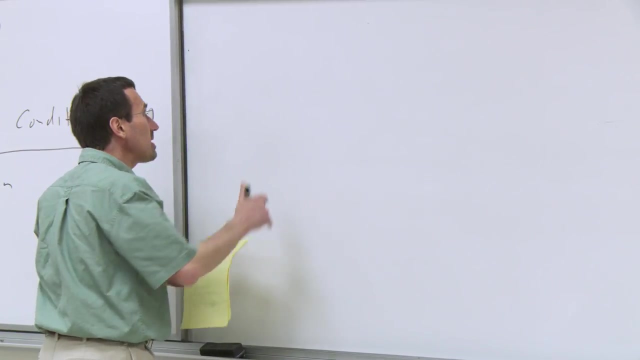 This is why the reactions are stereospecific And without changing the mechanism, say to a bi-radical mechanism at very high heat, you can't go ahead and break those rules And of course people poked and prodded. I mean this is. 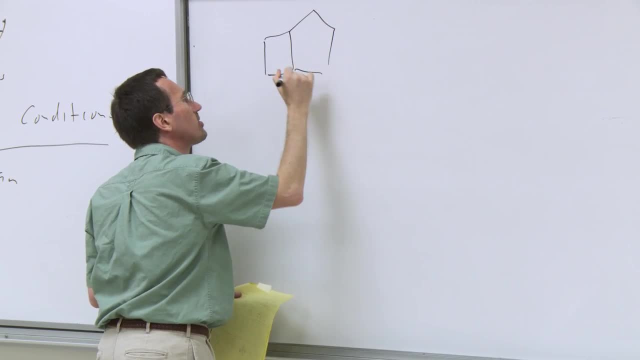 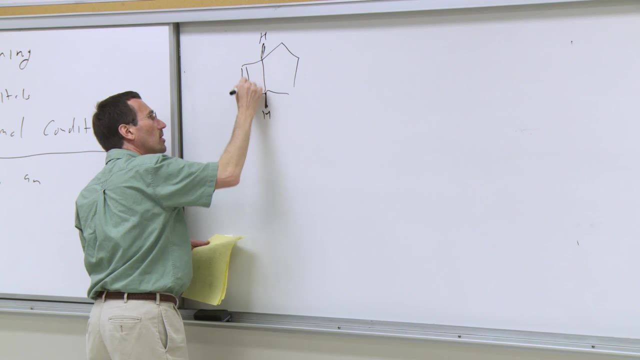 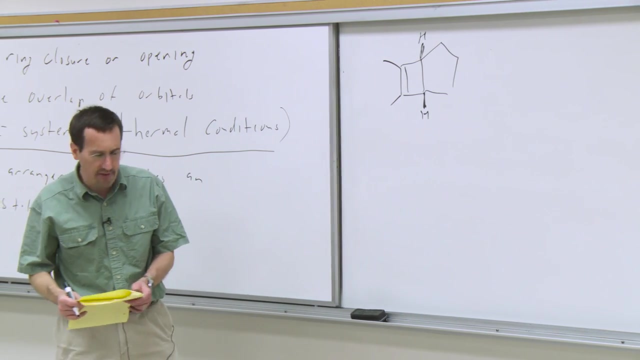 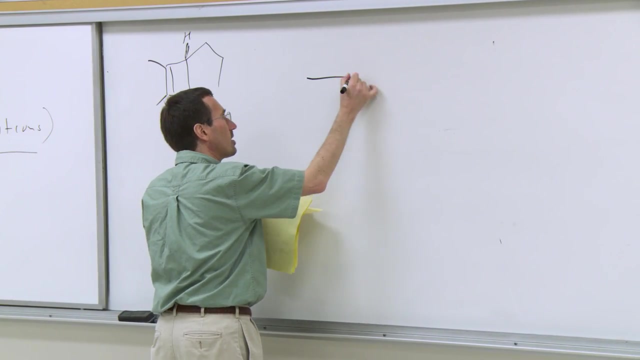 This is how organic chemists have understood, come to understand structure and bonding is through poking and prodding at reaction mechanisms and saying, well, what if I challenge it? What if I only give an alternative of doing something? So let's take this bicyclic system with a cis-ring fusion. 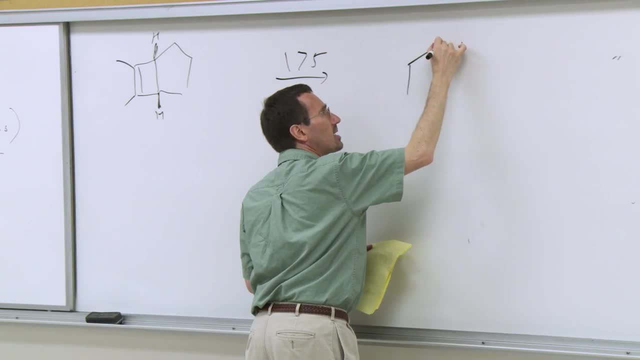 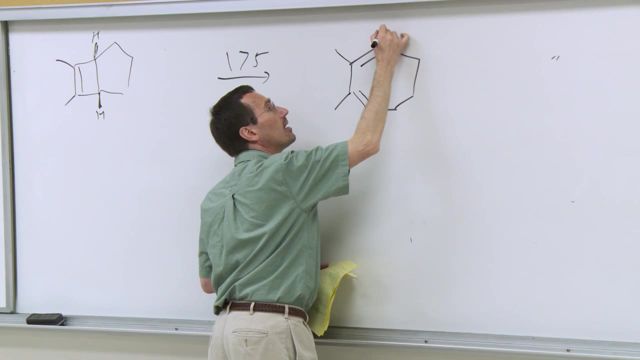 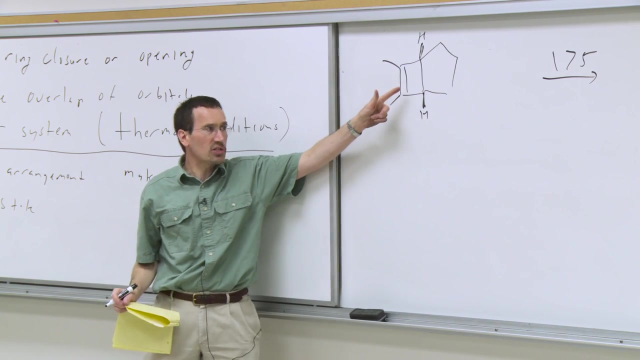 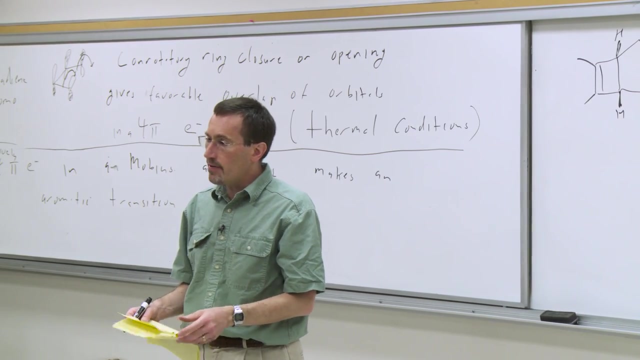 If you heat it to 175 degrees, it does not go ahead and open up like so. And the reason for this? it would like to. You've got a strained four-membered ring- cyclobutene opened up, But in order to open up it would have to go ahead and open. 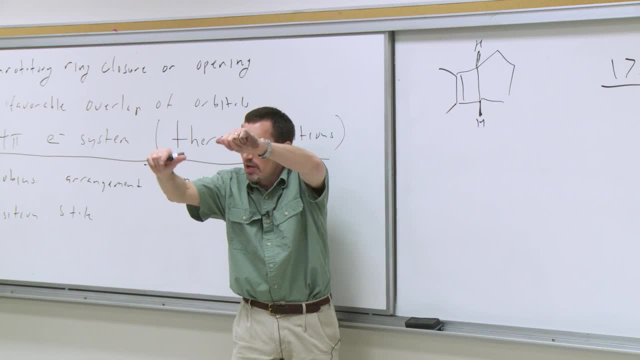 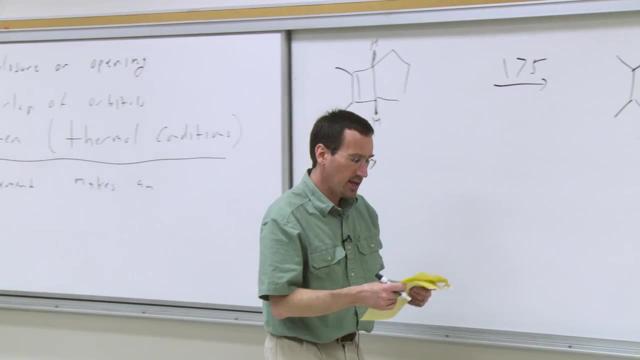 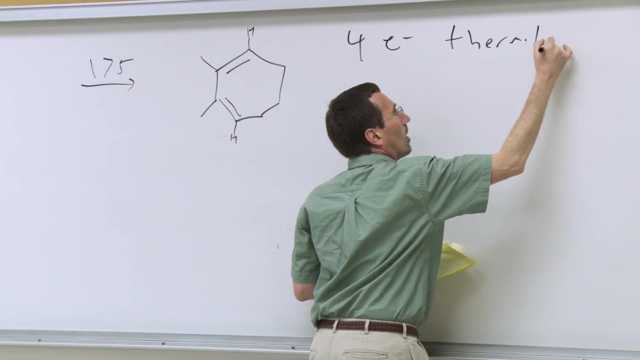 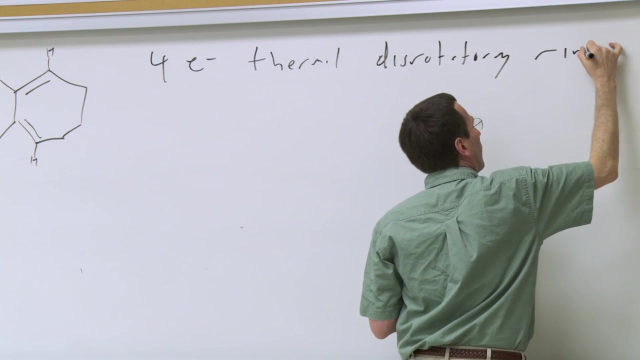 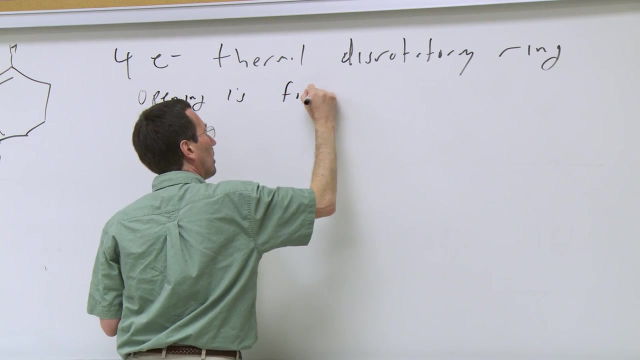 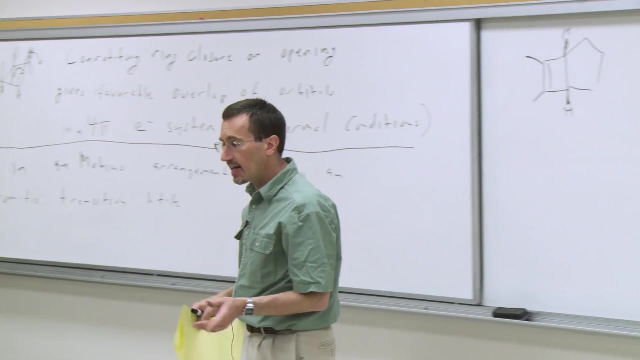 in a dis-rotatory fashion. In other words, those two hydrogens would have to come outward And dis-rotatory ring opening is forbidden. Consider the mechanistic reverse because, as I said, 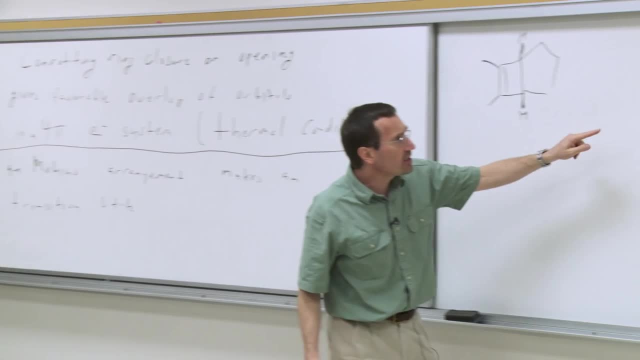 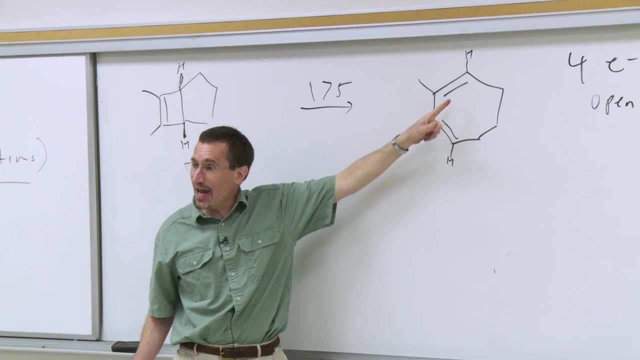 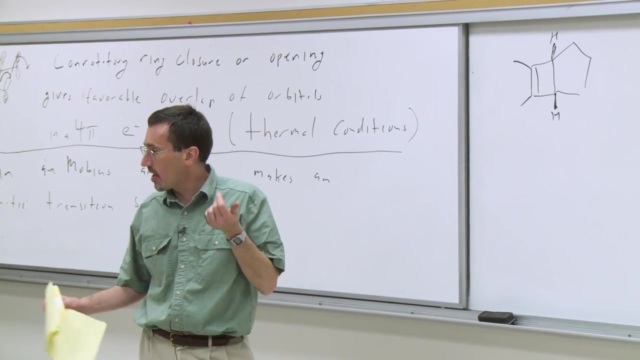 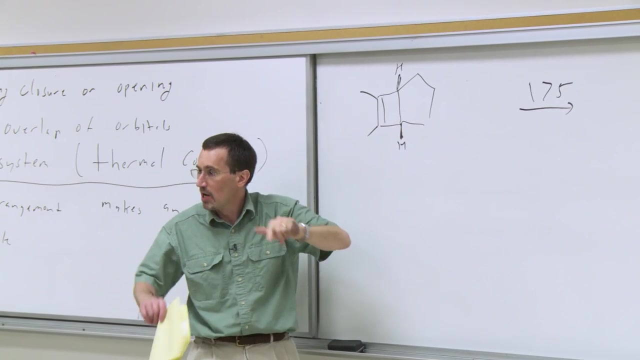 you can think forward, you can think backward. Trying to close this cyclohexadiene in a disrotatory fashion would result in a positive and negative orbital overlapping. In other words, it would result in antibonding interaction. Same thing applies in the forward direction. 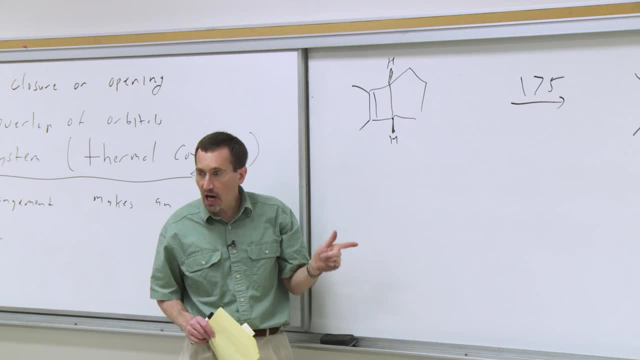 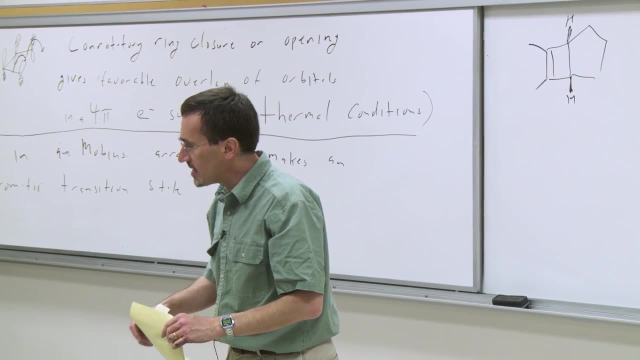 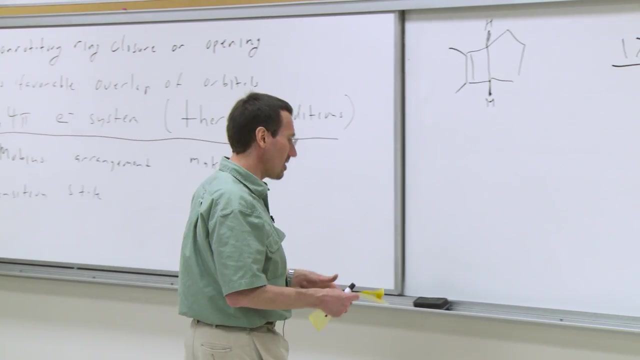 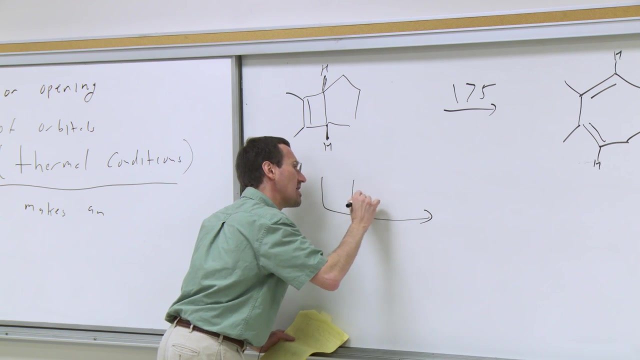 You cannot have disrotatory, And conrotatory would be impossible because that would put a trans double bond in a seven-membered ring and that's just too strained to occur. So basically, this molecule is stuck unless you shine light on it, And if you shine light on it, UV light on it. 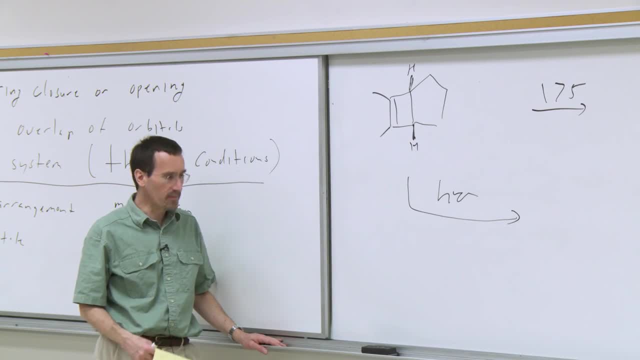 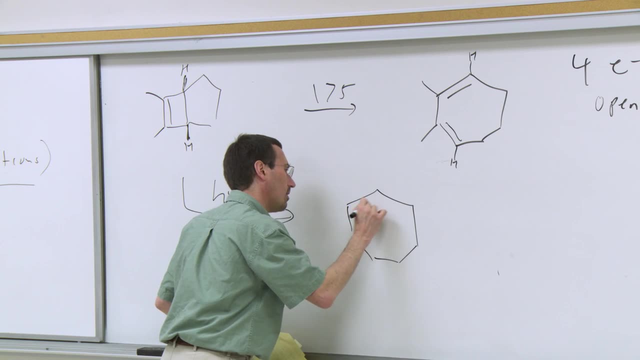 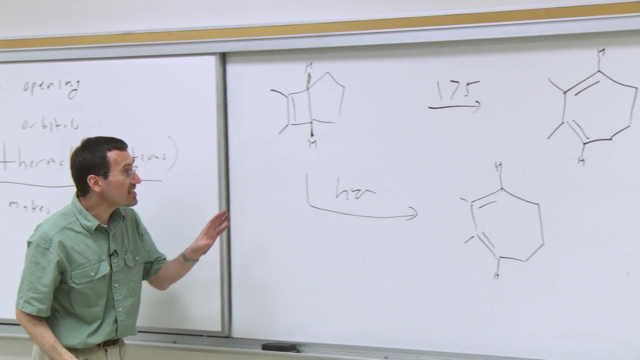 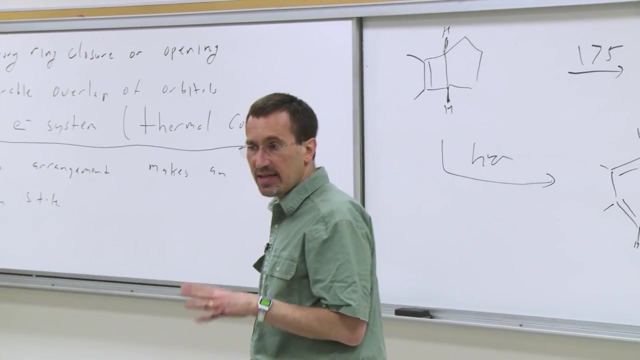 so now we're talking about near 200, 100 nanometers to be absorbed by an alkene. Then it happily opens up, And so we see that the rules now change and in fact, more specifically, we see that in general, a 4 pi electron process. 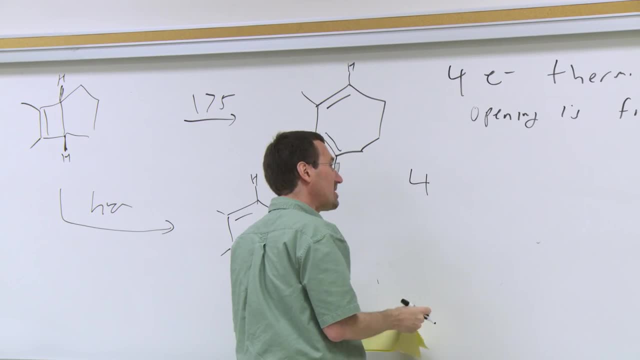 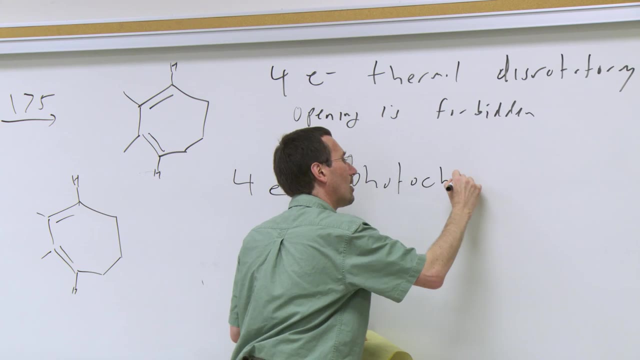 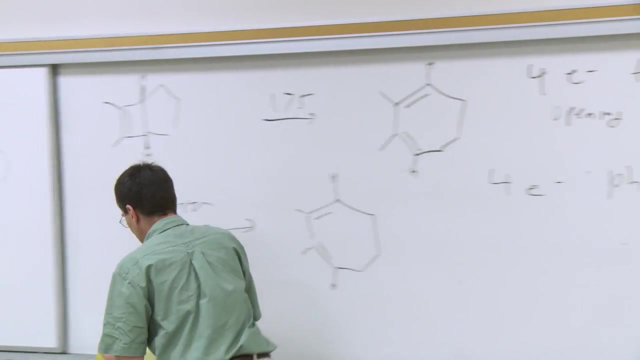 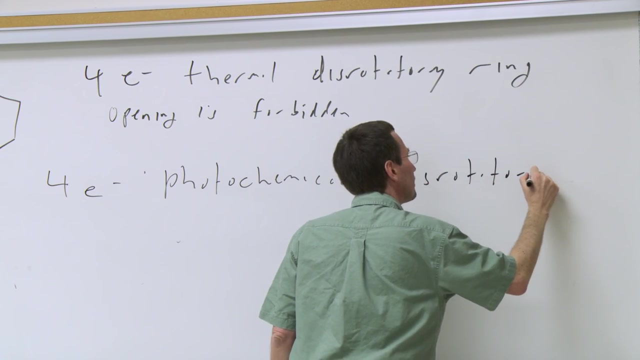 in the photochemical stage we're going to have a 4 pi electron process, And that's the same thing as we have to do in a bi hype delineation with the two other molecules in this case. so we have the two more protons. 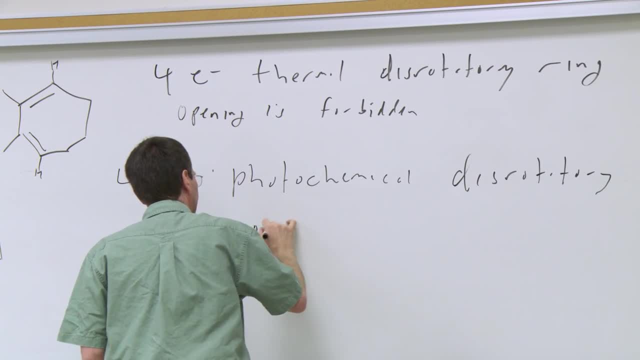 and we can now. Kontinuum state is disrotatory, Okay, So we can have the one we're looking at here, but we're going to have one final state. is this rotatory? So we want to have one final state. So let's just wait a second here, Okay, So if we have this one part, so what we're going to do here? we're going to find out what the condensate we're going to lay out into a pot. 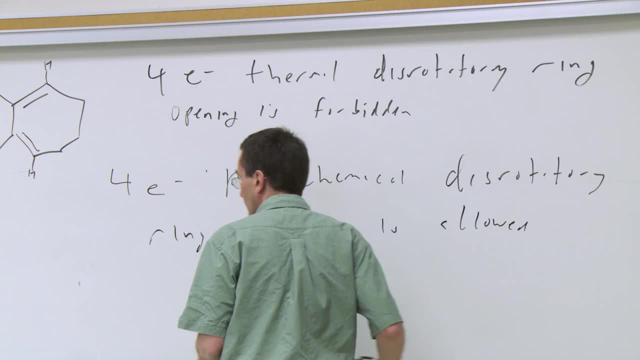 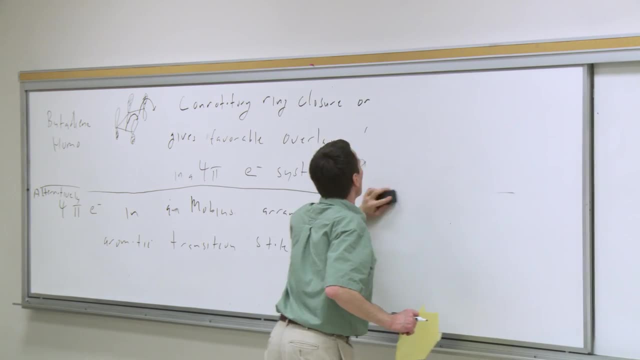 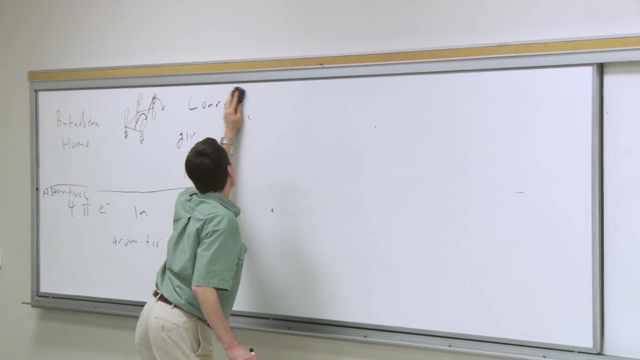 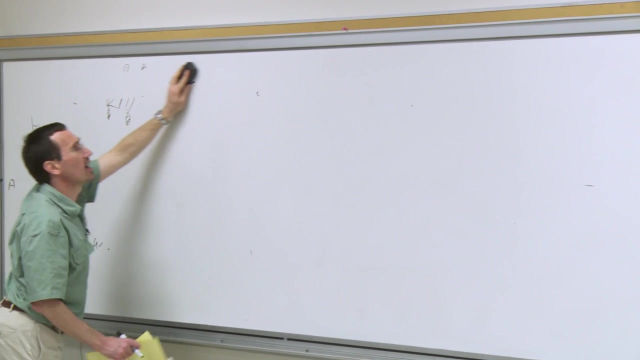 and we're going to take the radicals. Now. let's think about what's happening and see what's changed here And again. we're going to think about this from the point of view of the diene, because it's easier to conceptualize the reverse reaction rather than the forward reaction, but it's 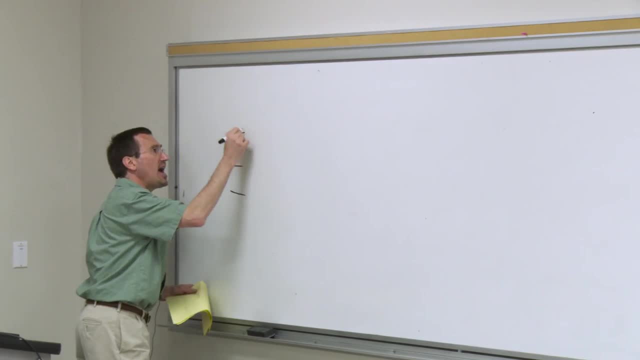 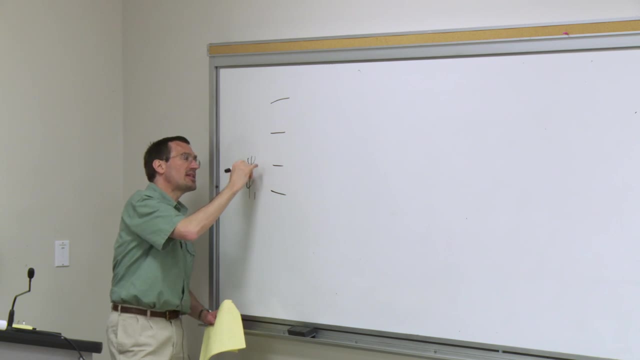 the same rules either way. Alright, so we have in the product because we're going to just think about it. in the reverse reaction we have our butadiene type of pi molecular orbital system: Psi 1, Psi 2, Psi 3, Psi 4.. 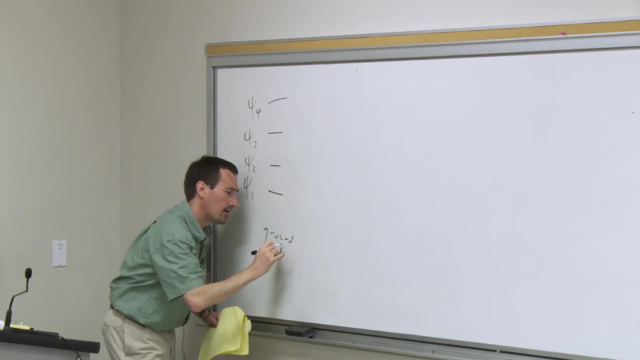 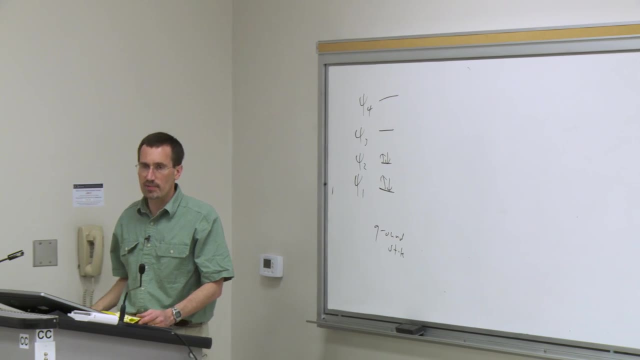 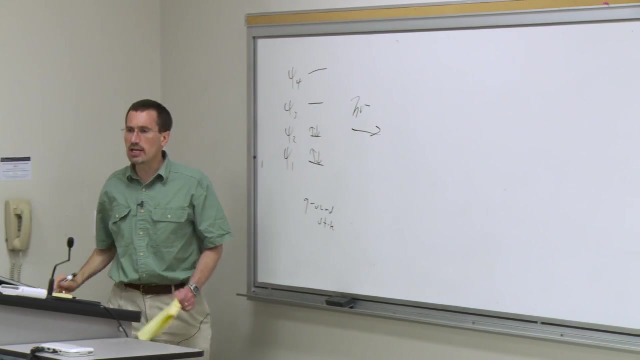 And in the ground state we have: Psi 1 is filled and Psi 2 is filled, The two bonding orbitals. The two bonding orbitals are filled When we shine light on the molecule. when we shine UV light, we have a pi to pi star. 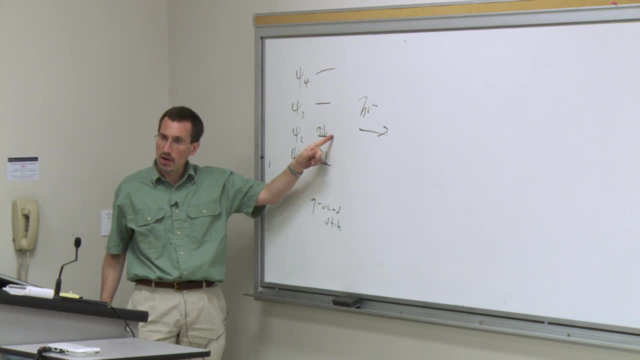 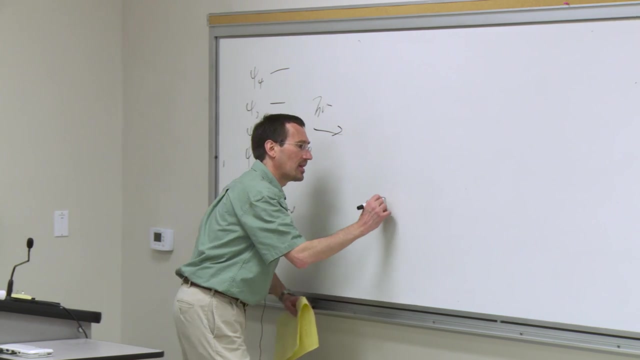 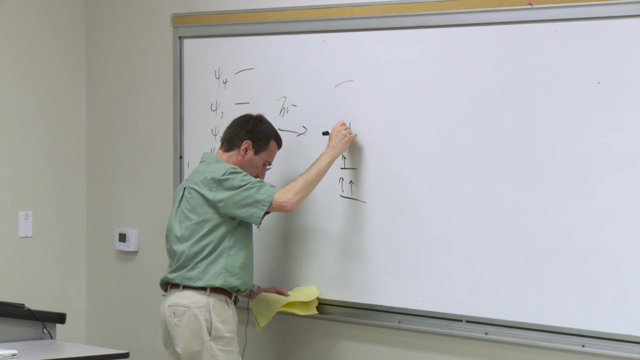 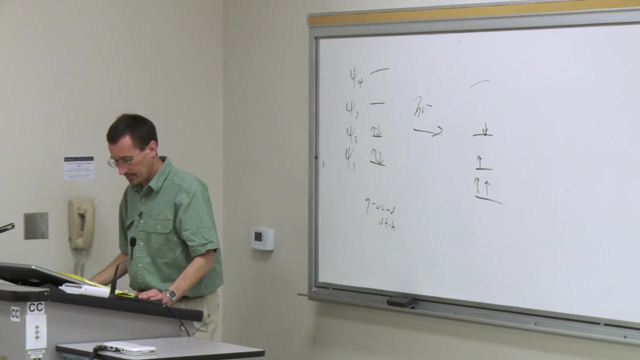 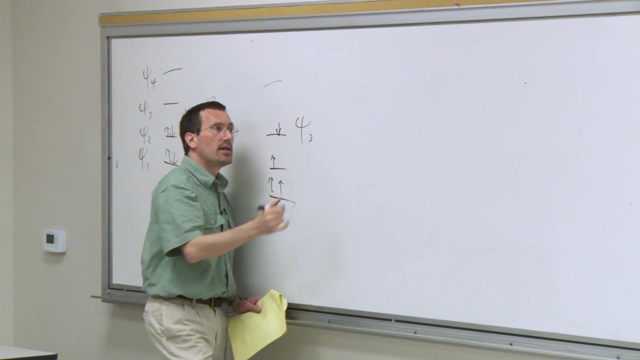 transition. In other words, we have the homo and we have the lumo, and we excite an electron from the pi molecular orbital, from the Psi 2 molecular orbital, to the lumo, the Psi 3 molecular orbital, And now, so this is our Psi 3.. 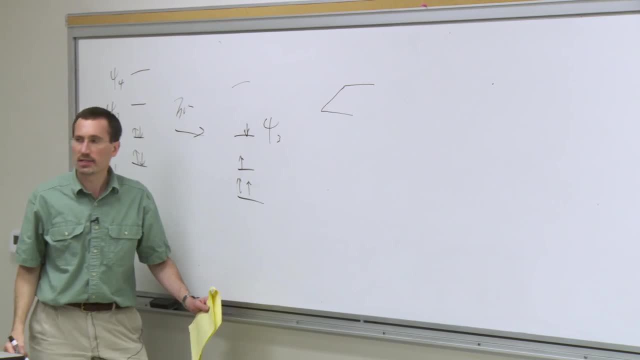 Now we can think about the action as occurring in Psi 3.. And in Psi 3, for butadiene, we have one more node And I'm going to draw this, And I'm going to draw this, And I'm going to draw this. 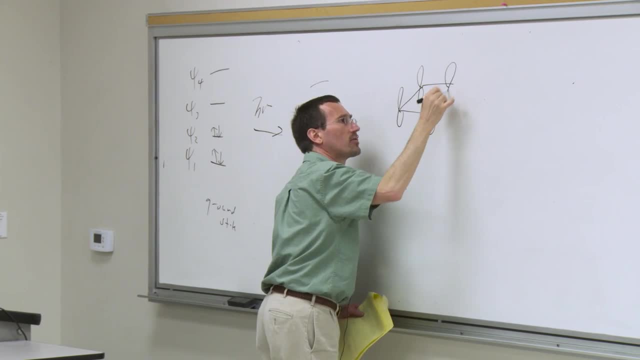 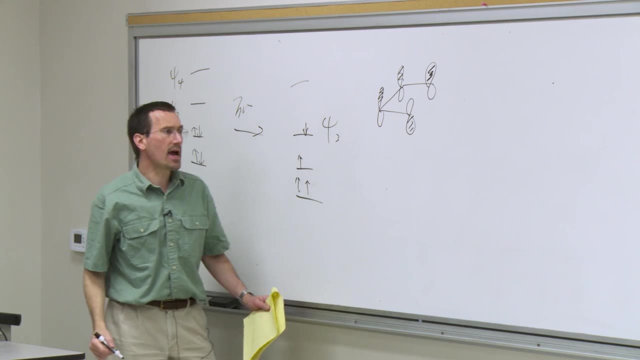 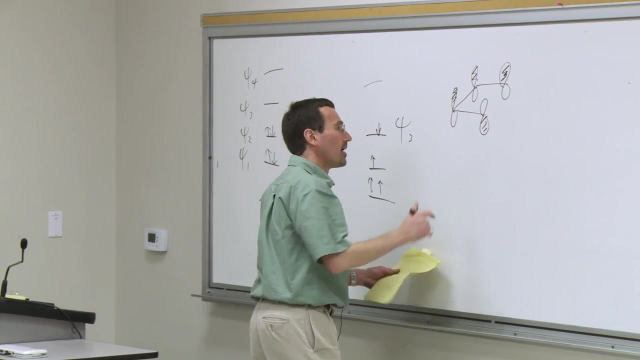 And I'm going to draw that. So here's our Psi 3.. And again, I'm drawing it in my little pigeon perspective drawing. And now in our Psi 3, we have an example where we can go ahead and have a disrotator, a. 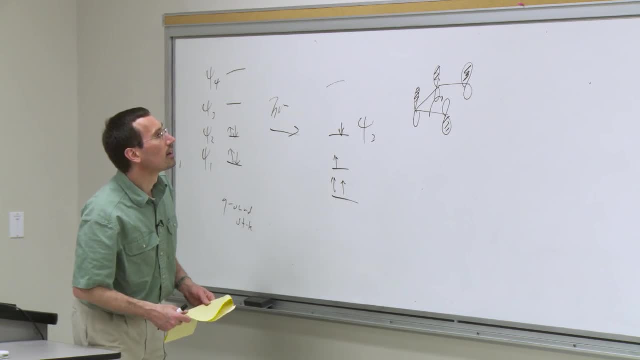 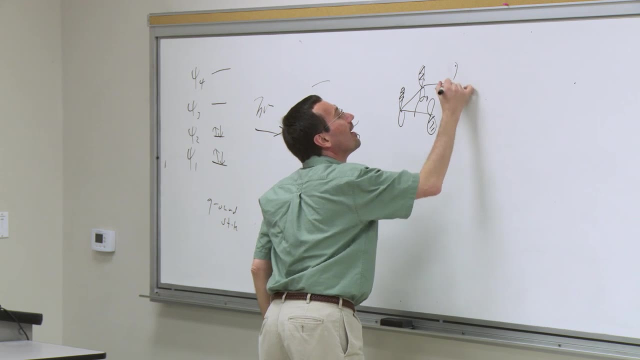 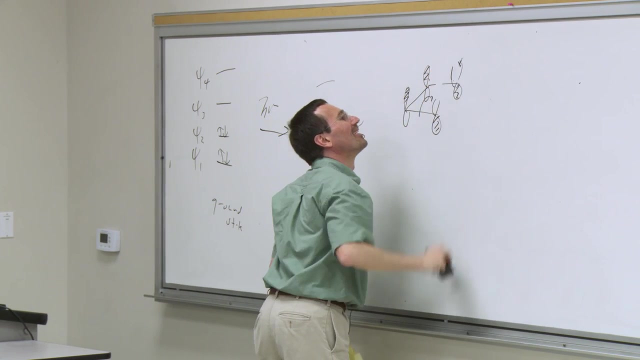 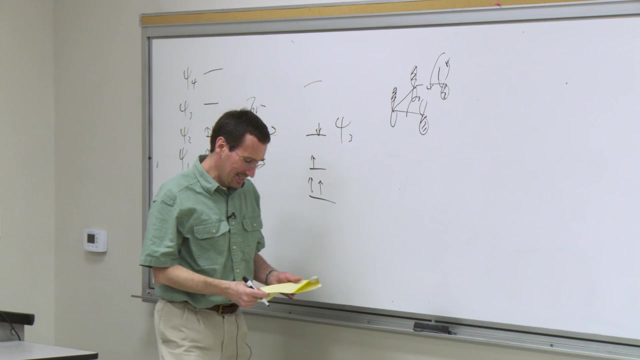 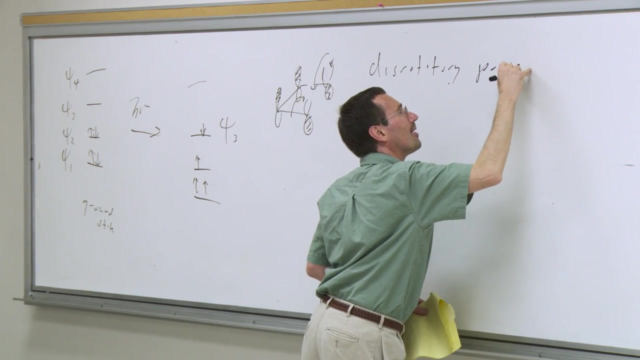 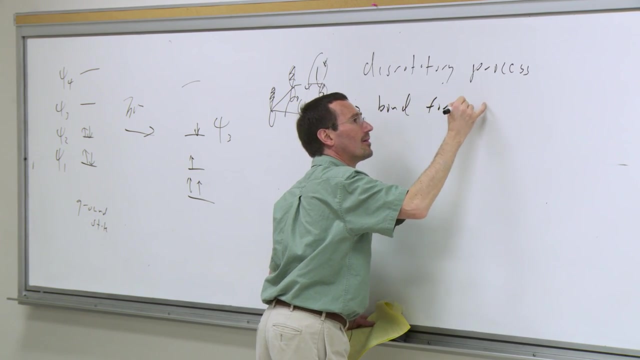 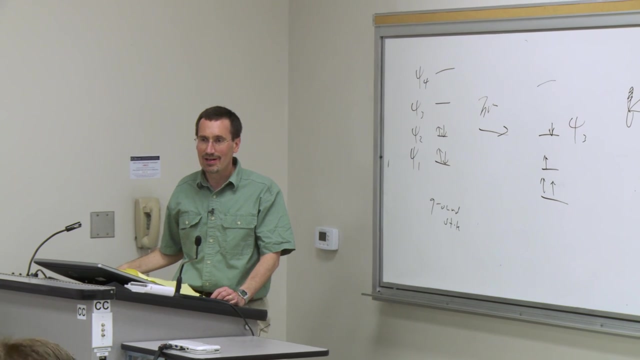 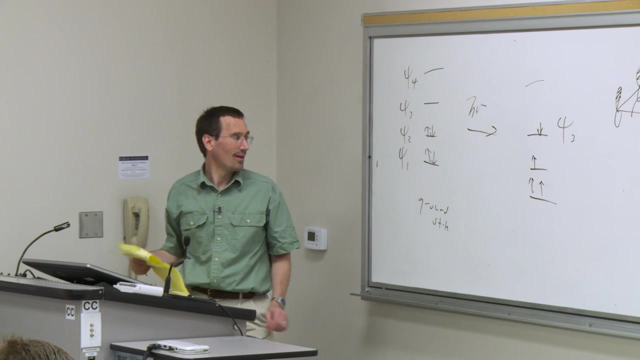 And let's take one, OK, so now. Oops, So now we can go ahead and have a disrotatory process. Subtitles by the Amaraorg community leads to bond formation. Alright, I saw a question. Oh, thank you. Now, that is my. 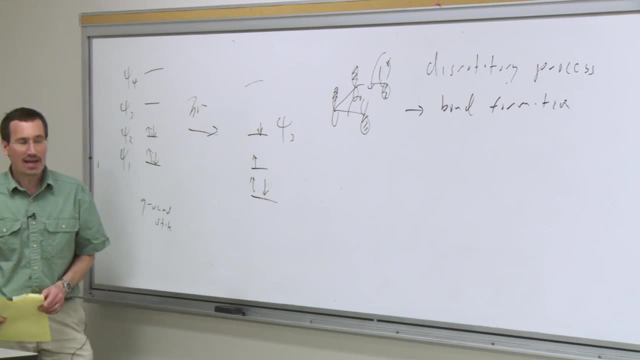 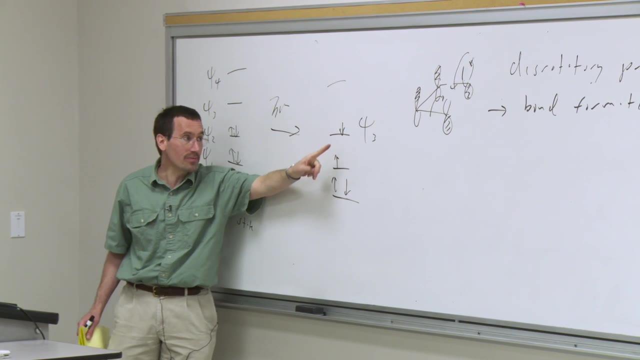 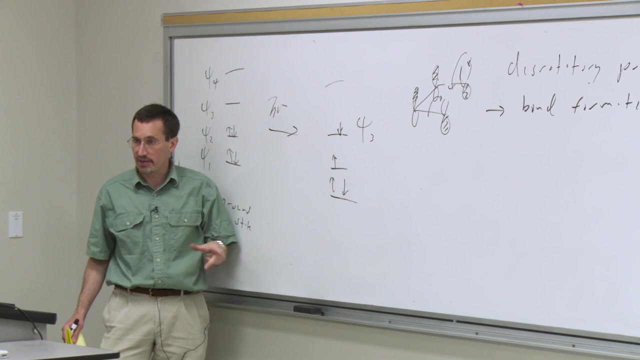 bad here, And technically, by the way, this is what I've called what one calls an excited state singlet, meaning that the electrons still have opposite spin to each other. If they were both the same spin, then it would be an excited state triplet. 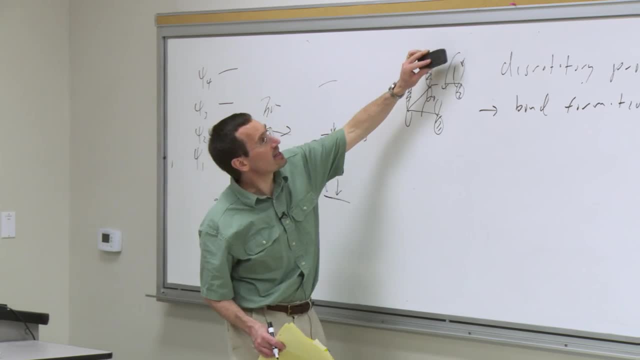 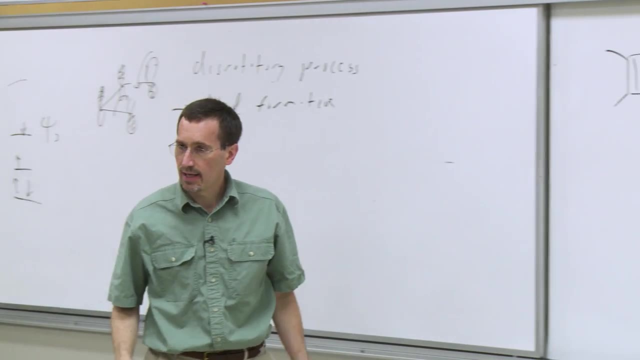 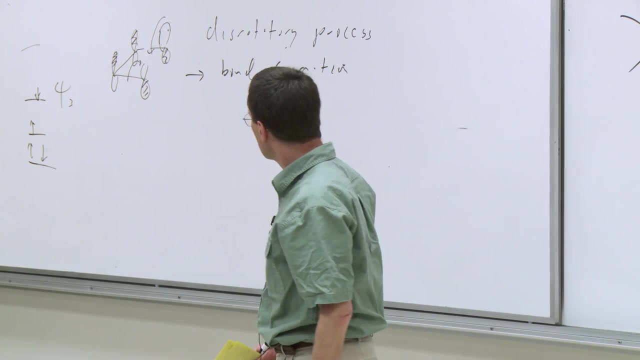 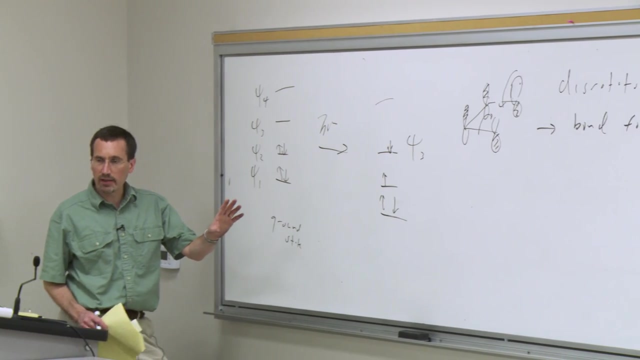 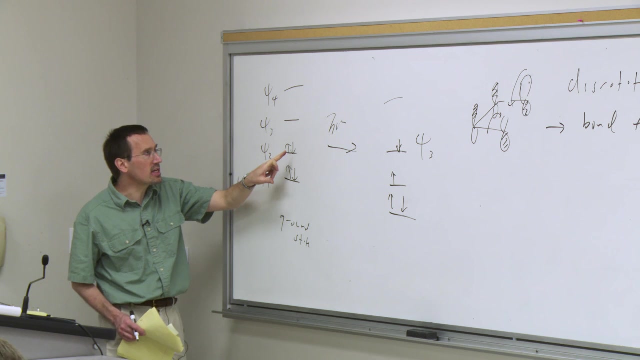 Other questions? I'm going to neaten this up. Thoughts or questions. Other questions: Yeah, So okay. so in the photochemically, so okay. So, if what happens now is in the ground state, Psi 2 transforms into the HOMO of the product, So, in other words, Psi 2, the HOMO of butadiene. 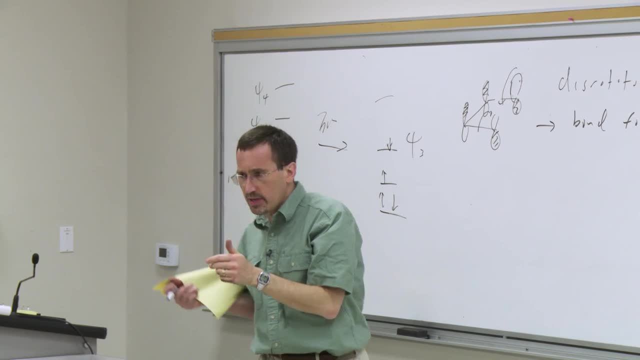 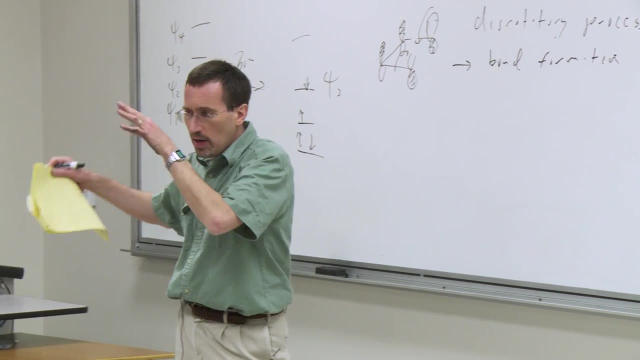 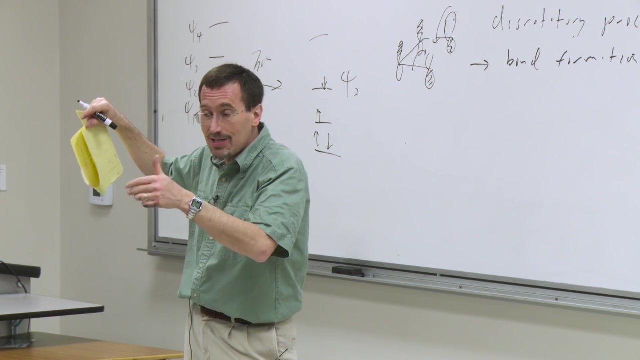 transforms into- we're just considering the opening- transforms into the HOMO of the product. Psi 3 becomes the homo of butadiene. Psi 2 of butadiene becomes the homo of butadiene. transforms into the LUMO of the product. 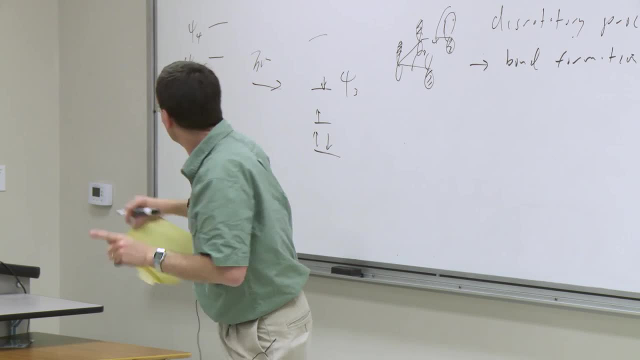 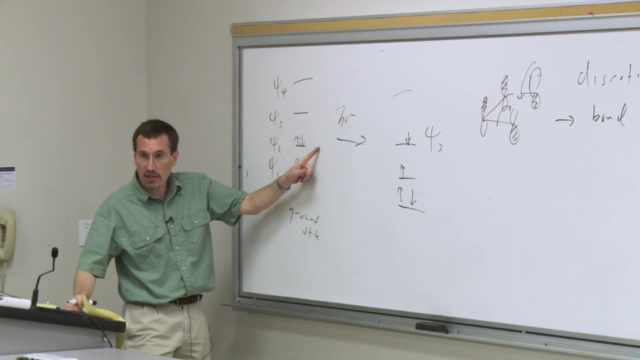 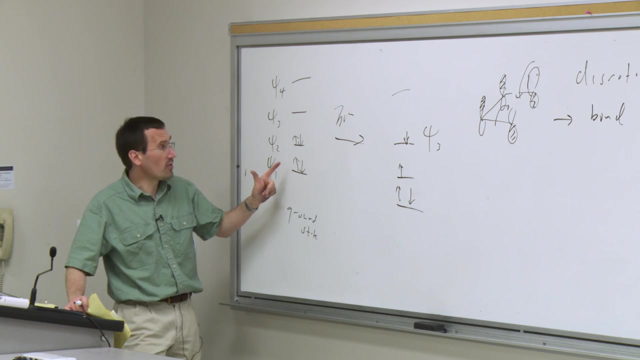 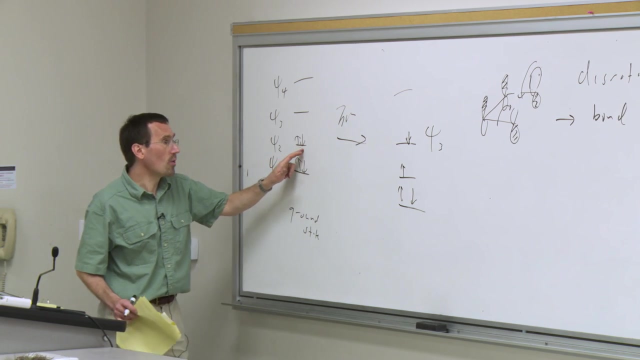 I'm sorry. Psi, no, that's right. Psi 2 transforms into the HOMO. Psi 3 transforms into the LUMO by a conrotatory process. But right, so a conrotatory process would translate: wait. 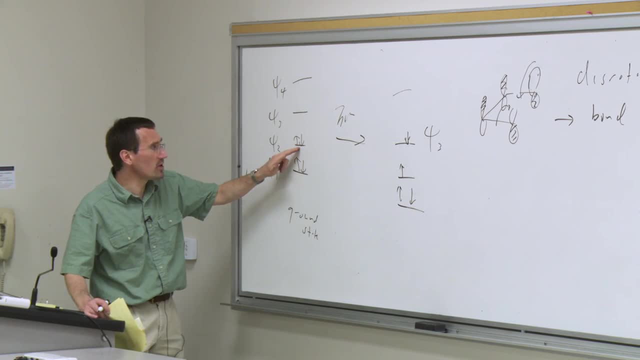 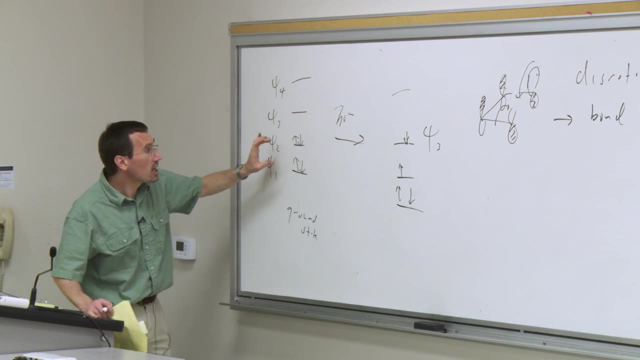 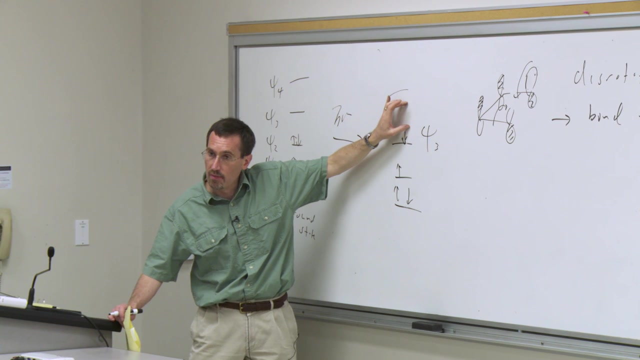 right conrotatory for electrons. So a conrotatory process translates Psi 2 into the HOMO. A disrotatory process translates Psi 2 into what would be the LUMO of the product. but That means you would generate the product excited state. 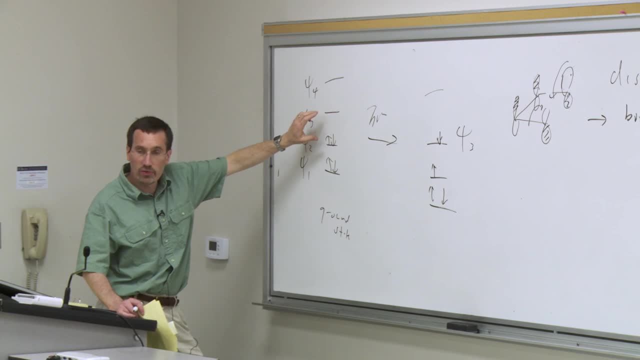 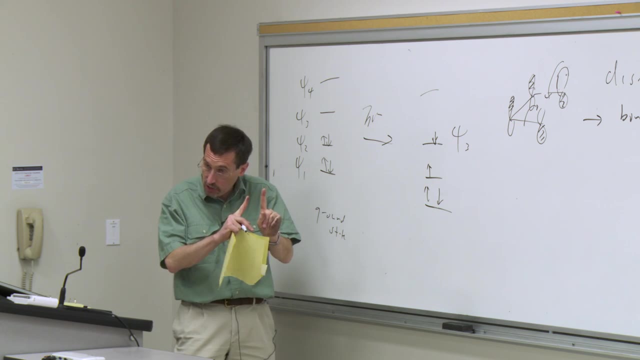 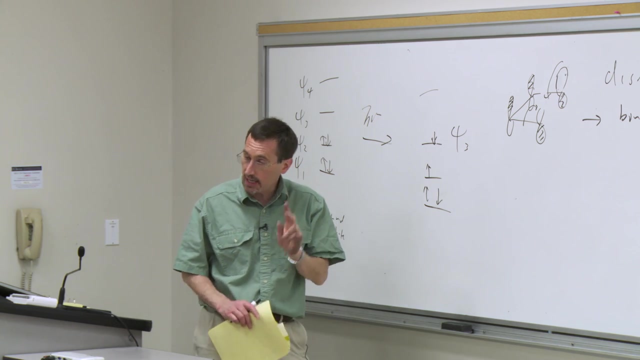 Now here what happens is, because you have both Psi 2 and Psi 3 populated, you still get an excited state product. You just switch them around. You still have two half occupied molecular orbitals, but you're not generating a molecule in the doubly excited state where two electrons are. 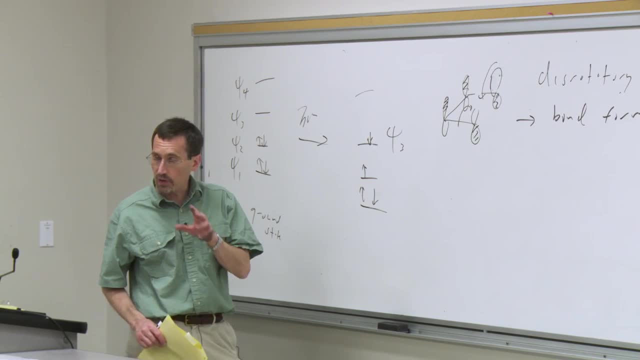 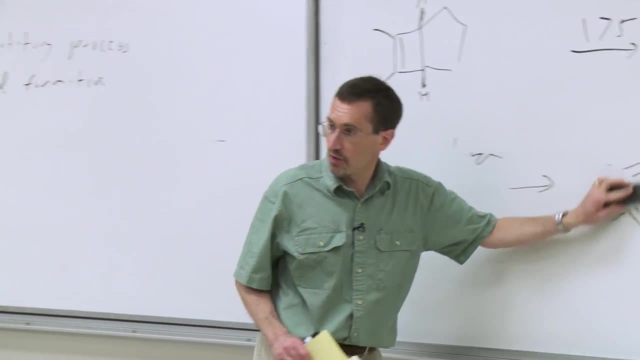 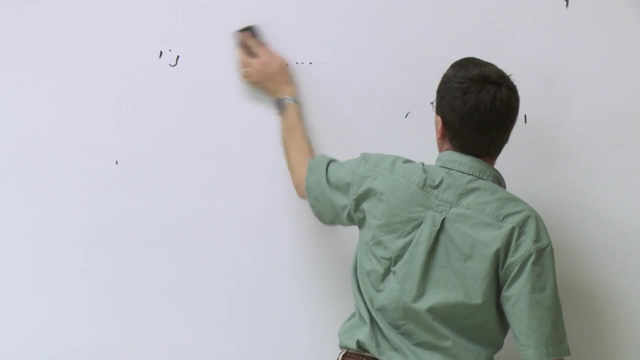 in an antibonding orbital. Basically, what happens is you have to have electron in order to have a reaction occur. you have to have electrons going into a low energy orbital. You can't go and populate a high energy orbital, All right. 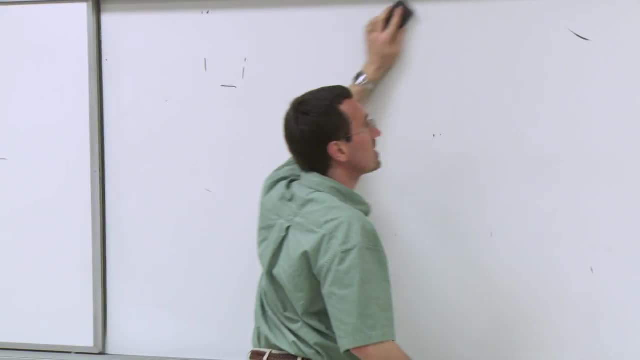 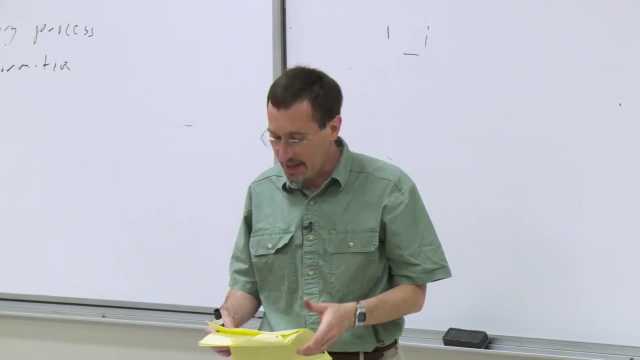 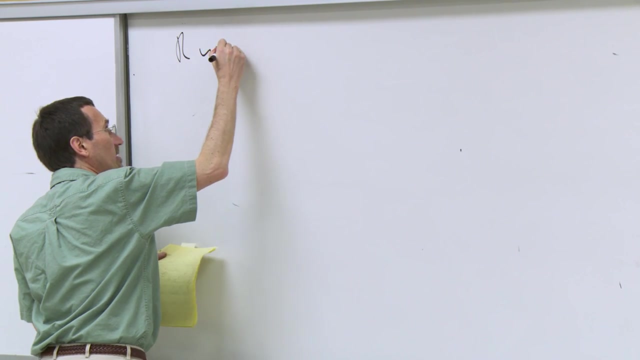 I want to give a little table to sum up- and honestly I never use this table because I always just sketch out the molecular orbitals for the HOMO and think my way through from there. but I want to give you the rules for electrocyclic ring opening or closure to finish up. 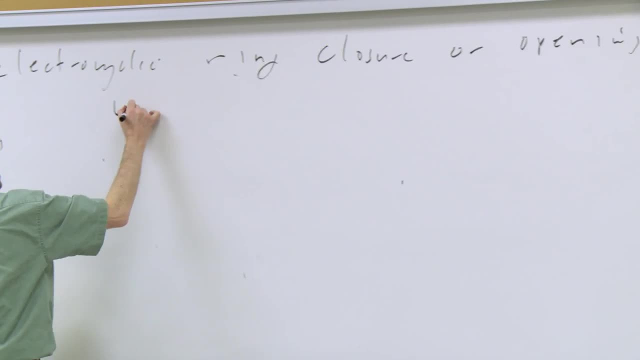 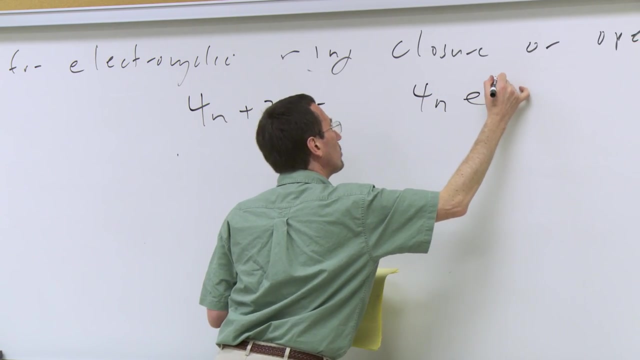 And all I'm doing is generalizing the things that we've said. We're going to talk about 4N plus 2 electron systems and 4N electron systems, And we're going to talk about the HOMO and the HOMO. 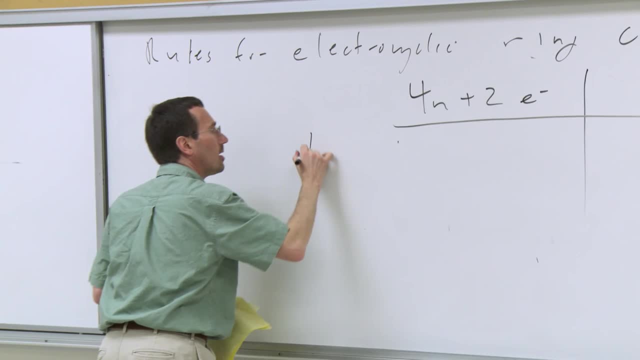 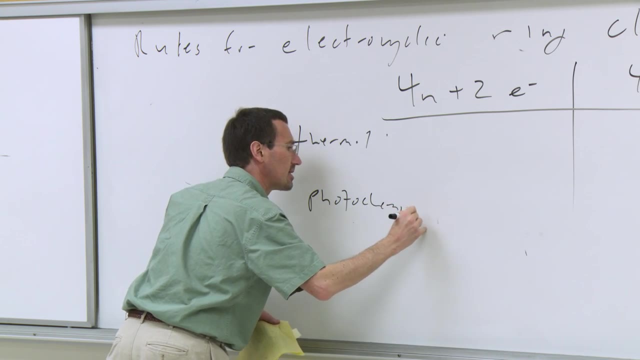 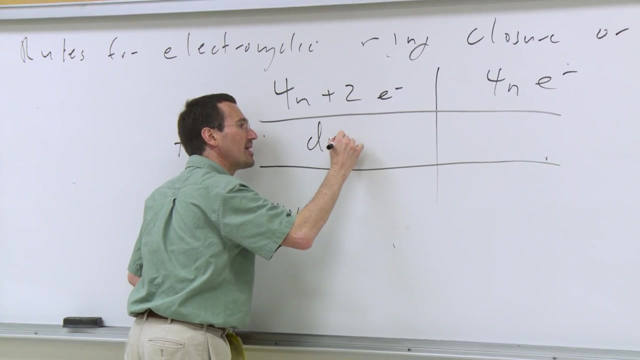 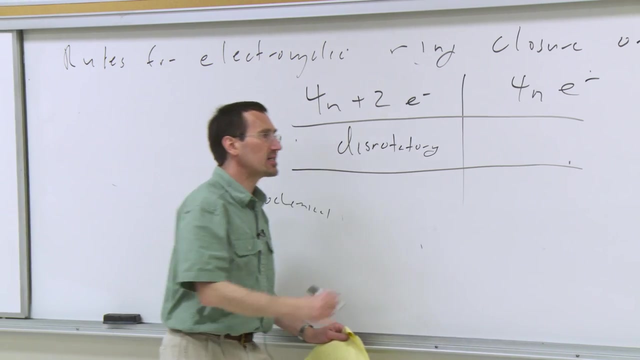 And we're going to talk about thermal and photochemical processes And basically, if you know one, you know them all. We started with 4N plus 2 in a thermal manifold is disrotatory and 4N is conrotatory. 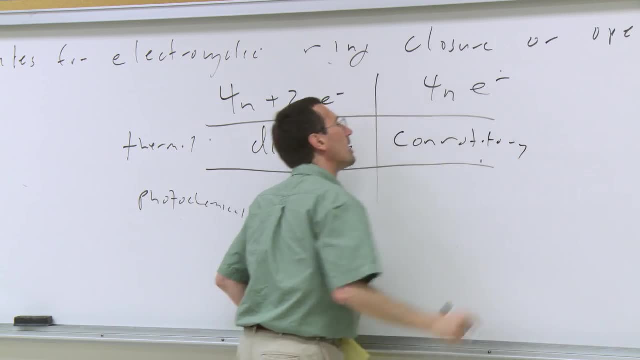 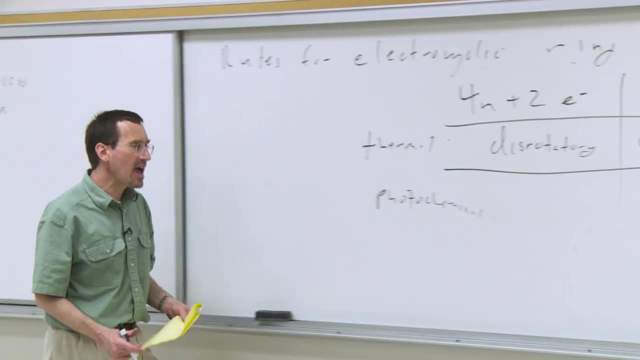 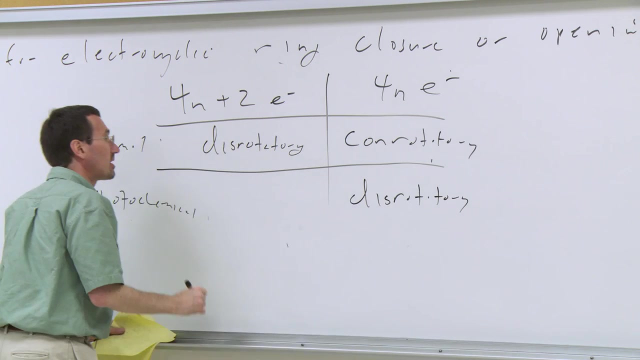 And then we're going to talk about the HOMO and HOMO. And we're going to talk about the HOMO and HOMO. And then we said the rules swap when you go into a photochemical manifold. And now 4N is disrotatory and conversely.